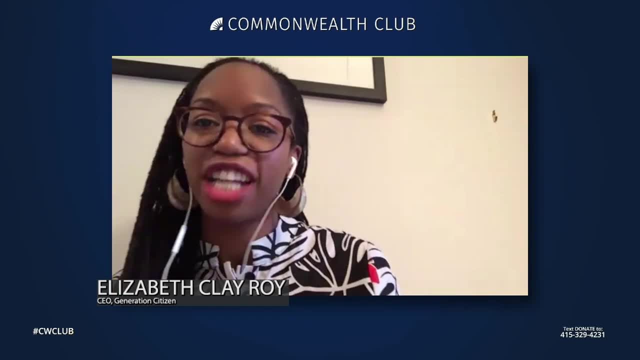 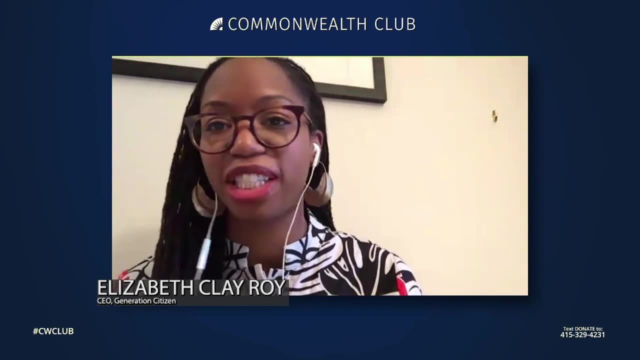 across the country giving students the chance to experience real-world democracy, And our Action Civics program is in classrooms from the Bay Area to Oklahoma City, New York City, communities, small and large, around the country, And I'm so glad to be with you today. 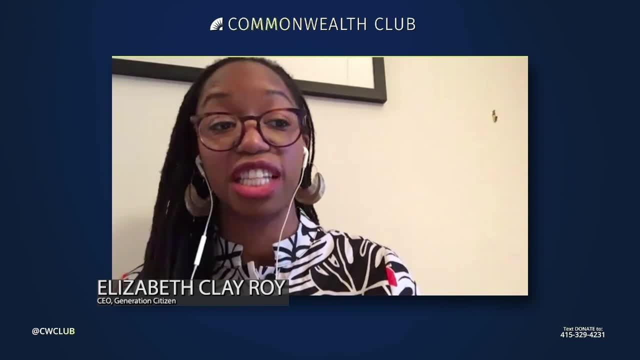 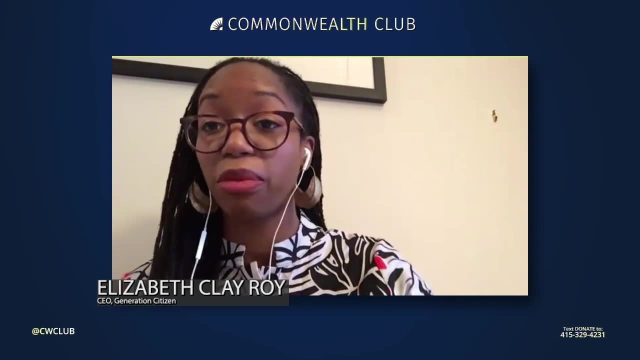 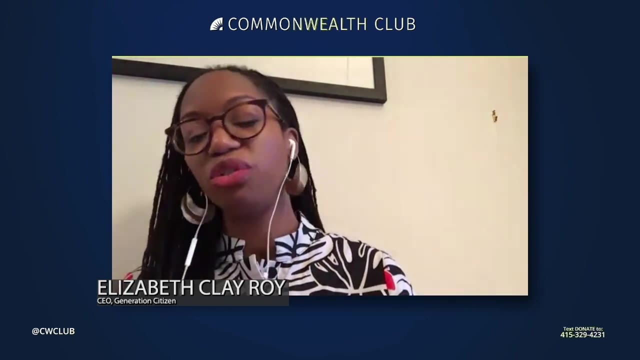 I'm especially pleased to be moderating a conversation for today's Commonwealth Club program After the Capitol siege- the need for civics education, with some incredible leaders and thought leaders in this space. This program is part of Creating Citizens, the Commonwealth Club's new civic education effort launched just last year. Today I'm joining you from my home. 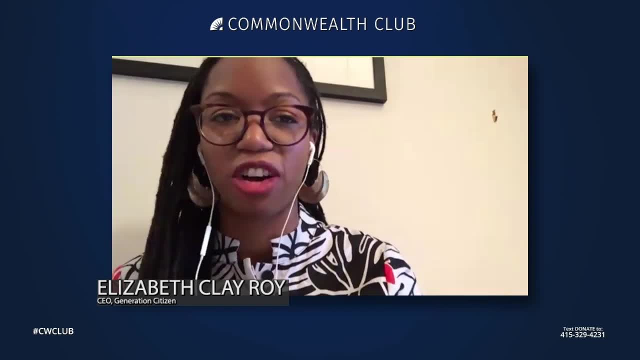 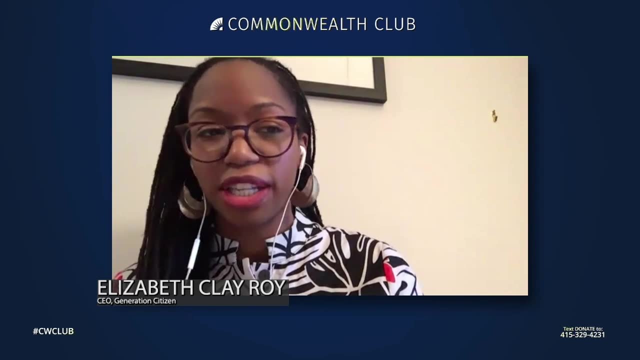 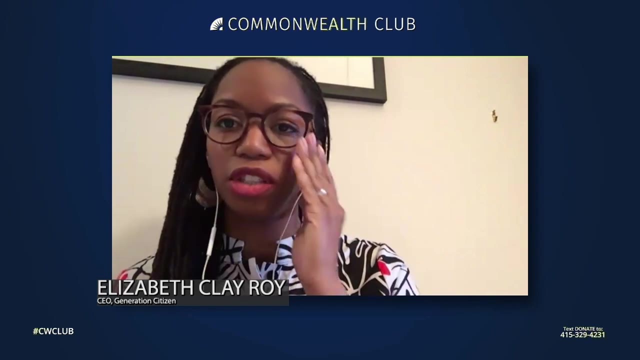 in New York City. I started my job at Generation Citizen on January 4th 2021, just two days before the riot at the Capitol. We, as an organization, instantly recognize the need to support teachers and students, to have conversations and make meaning of these tragic and scary events. 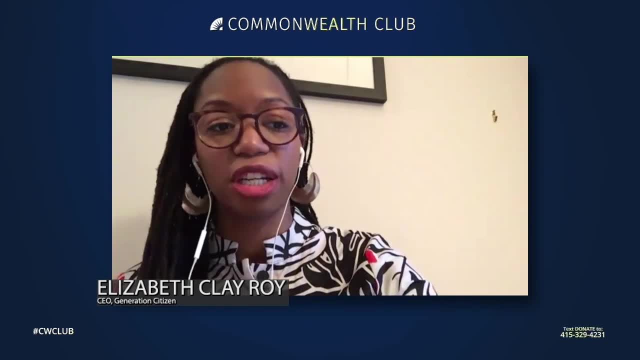 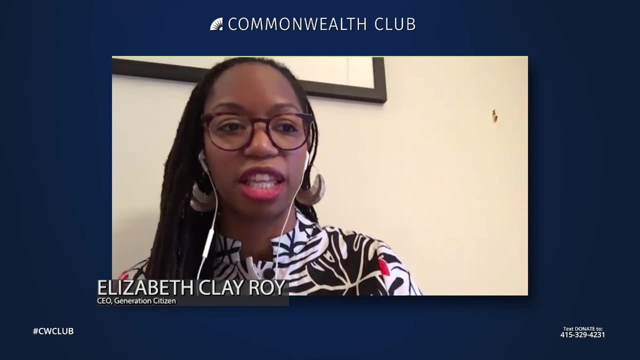 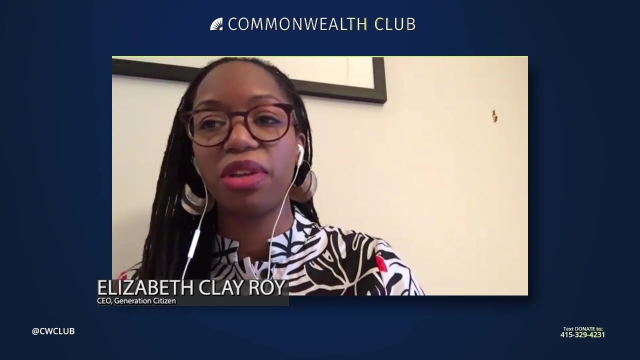 The long overdue to commitment in civics education across the country means there's a short-term outcome of leaving young adults adrift in difficult moments like these about their role as citizens, And it further leads to a crisis in terms of the continued erosion of democracy more broadly. Two of our speakers today, Mark and Lauren, felt that urgency instantly. 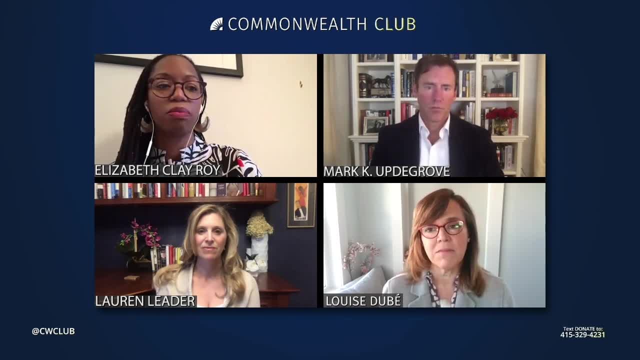 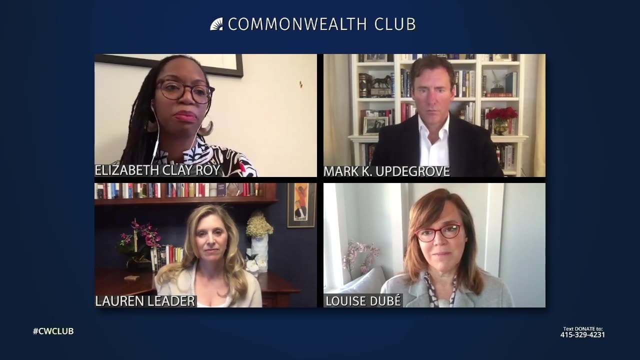 and put together an important piece in the Hill And we look forward to hearing from them about that article Before I turn it over to our great speakers to share a little bit about their experience and perspective on this moment. I just want to share something, And I know many of you. 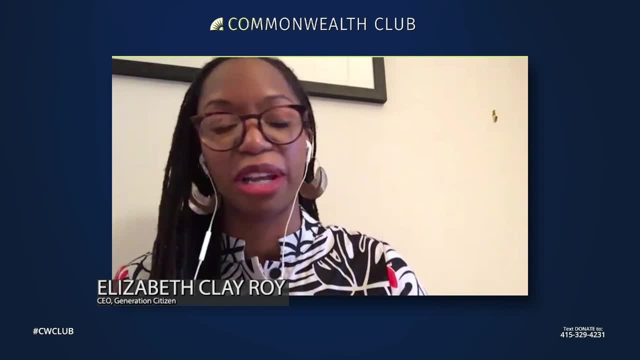 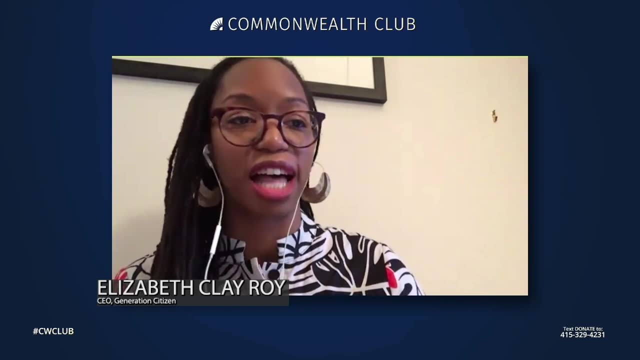 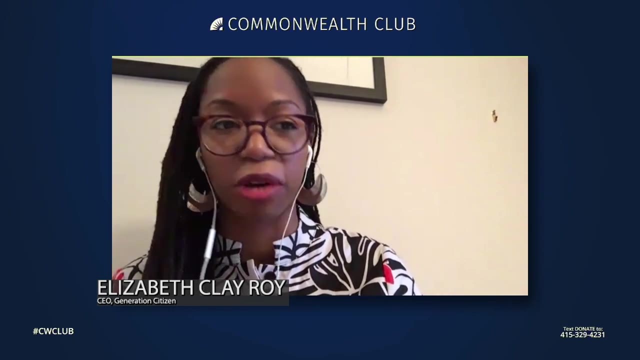 like me, were moved by inaugural poet Amanda Gorman and the perspectives that she voiced so powerfully in her poem The Hill We Climb. The first, of course, is that we did not feel prepared to be the heirs of such a terrifying hour: Pandemic economic crisis, racial injustice. 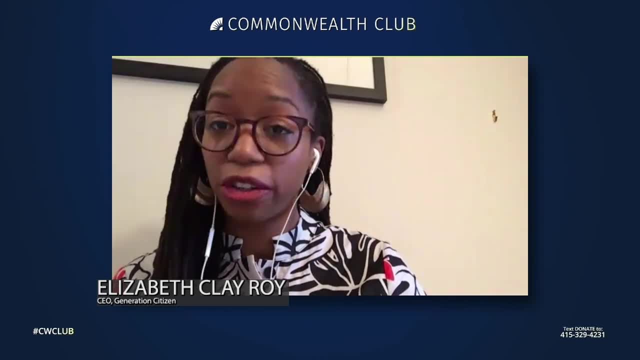 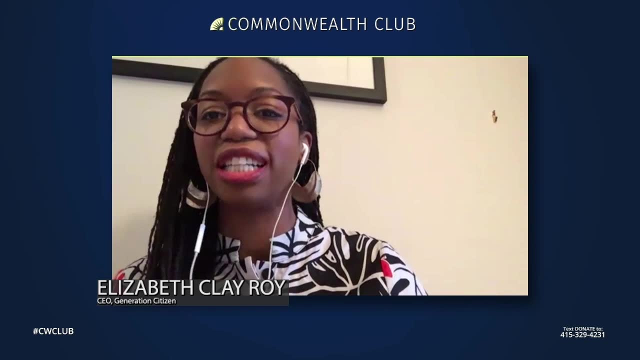 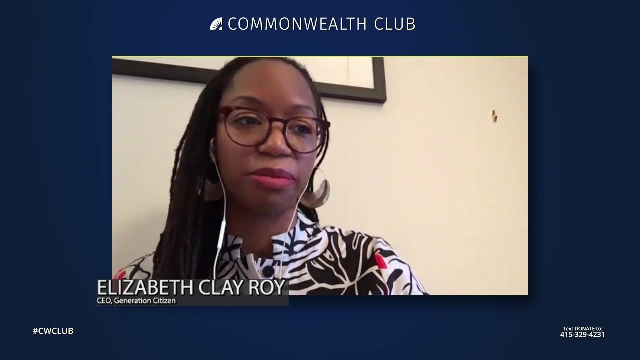 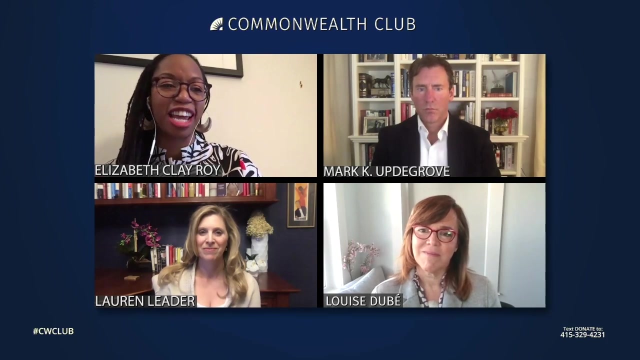 a contentious election, fires that continue to demonstrate the climate crisis, And 2021 itself has brought three consecutive and consequential Wednesdays: an insurrection, a second impeachment and an inauguration. Coming back to Amanda Gorman again, she said on that last Wednesday: 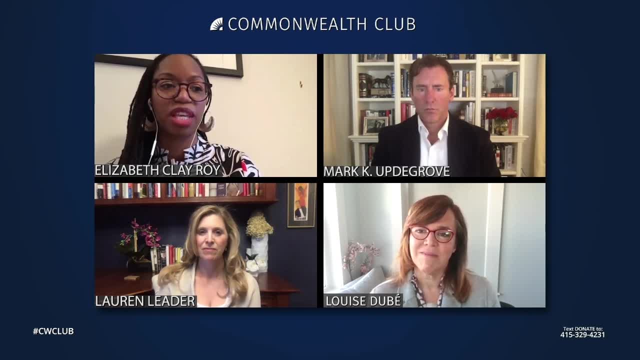 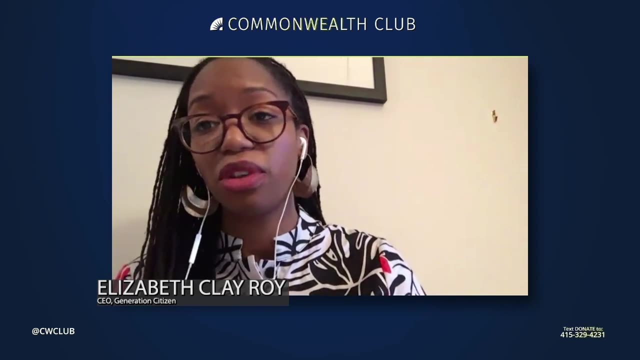 we will not be turned around or interrupted by intimidation, because we know our inaction and inertia will be the inheritance of the next generation. That's really what we're talking about. We are in this critical moment now for civics education and we're really having, I think, a conversation that may be a call for action, for comprehensive 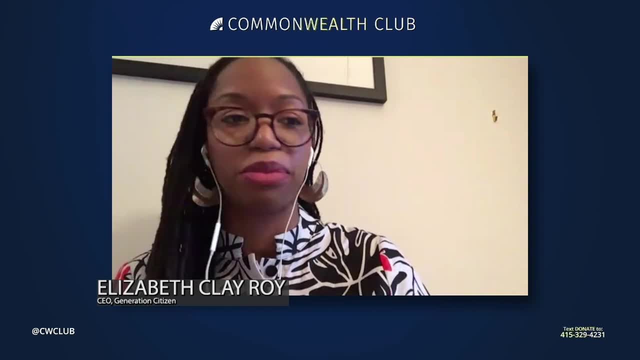 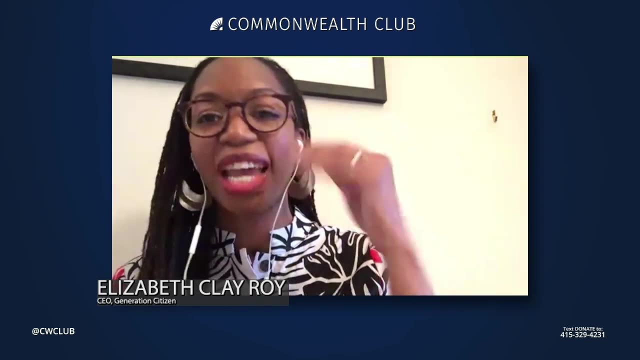 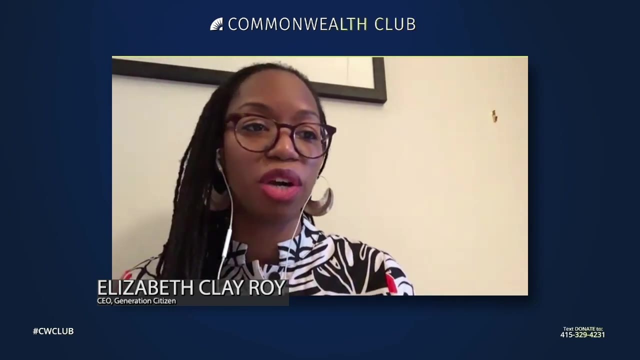 civic education that is different, perhaps, than past ones, And we want to talk about how we can have a lasting change in our understanding of diverse civic traditions, how government works, and roles and responsibilities. So today, to discuss these issues, I'm really thrilled to be joined by three people who 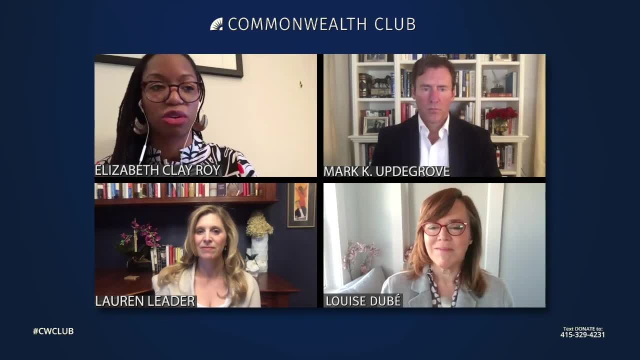 represent different organizations and perspectives on the importance of civics education across the country. We're going to start with hearing from Louise Dubé, who leads iCivics, one of the country's leading civics education organizations, who's pioneering new approaches to this critical 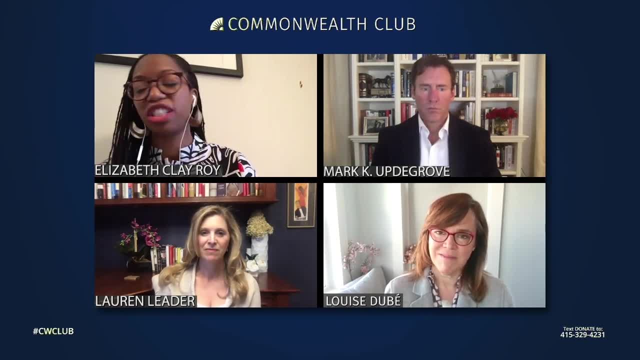 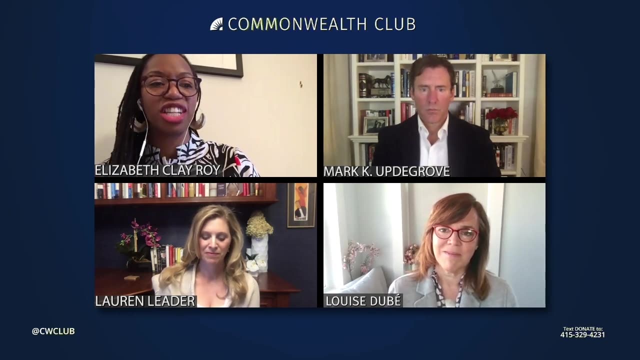 issue And, as I mentioned earlier, the author of a recent editorial on civics education published in The Hill. Lauren Leder, the founder of All In Together, a nonprofit- a nonpartisan nonprofit women's civic education organization, also here in New York City. And Mark Updegrove, the president. 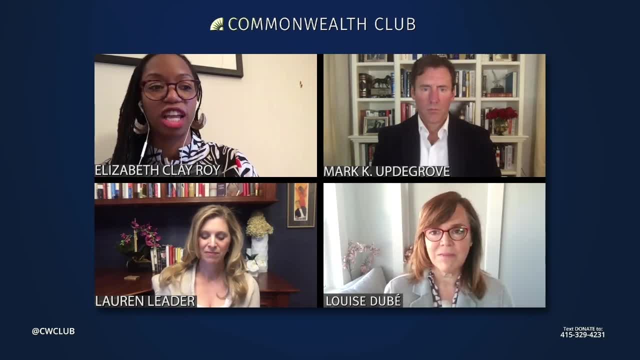 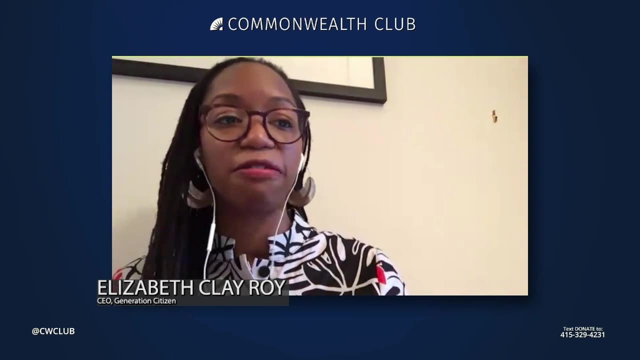 and CEO of the LBJ Foundation in Austin, Texas, and presidential historian for ABC. Before we turn it over to them and our conversation, a little bit of housekeeping. If you have a question for me or any of the panelists today, please use the YouTube chat feature. Questions there will be submitted. 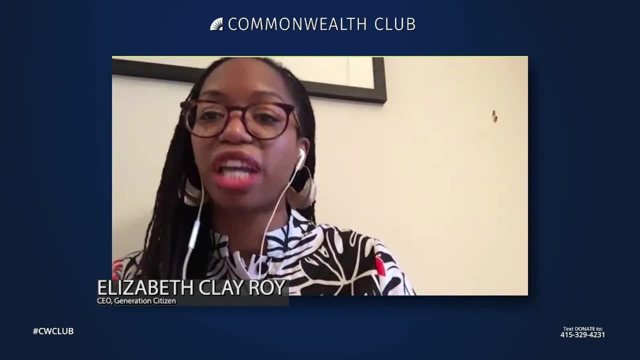 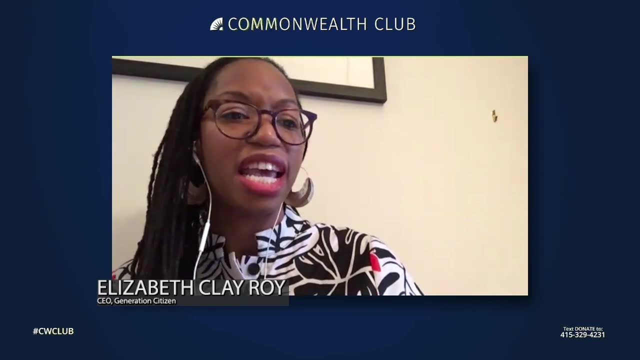 to me throughout the program and I'll try to ask as many of them as I can. So we'll be talking about the different perspectives that we've heard from the speakers and bringing them into our conversation, or making sure that we get to them after we've had a chance. 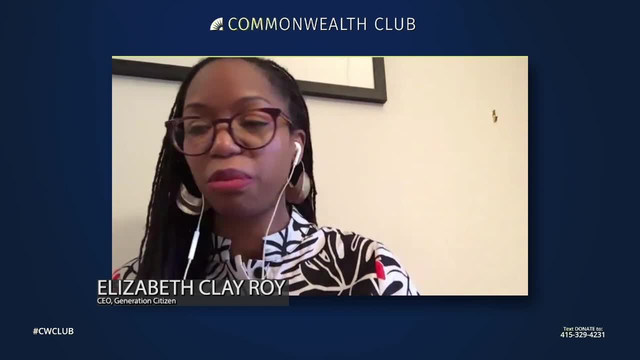 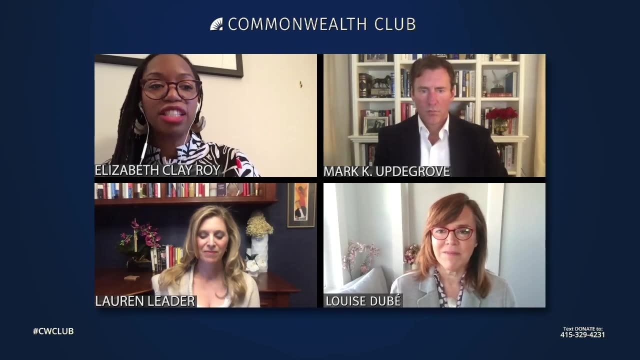 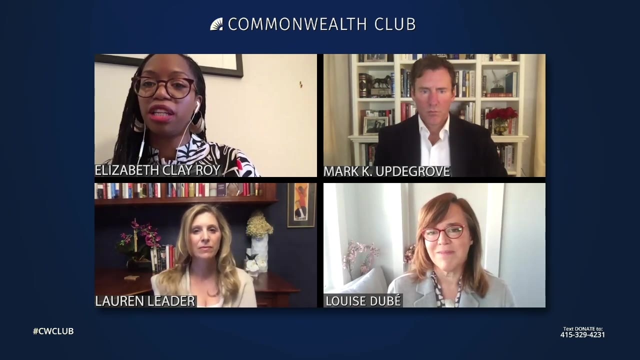 to hear from the speakers And I really could not think of a better group to bring together to make this urgent call for action. So I want to begin by hearing from Louise. Why is this such a critical moment and what makes this moment different from others where there has been discussion of the need? 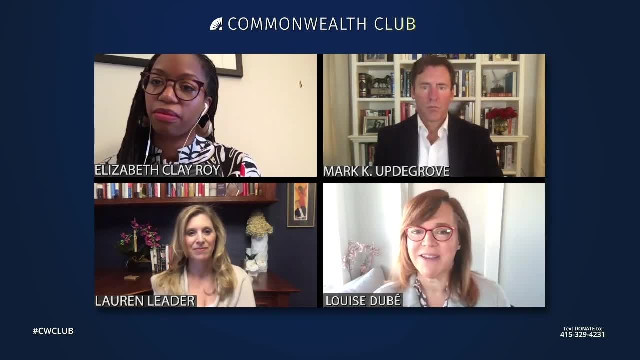 for civics education. Well, thank you so much. Thank you to the Commonwealth Club for bringing us together about this important issue and thank you, Elizabeth, for this beautiful opening. I think starting with Amanda Gorman is a great place to start. 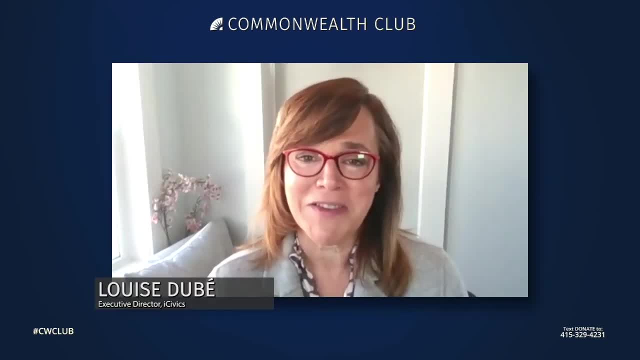 I think she captured the moment. That's why she's been such a sensation after her poem was read- And she captured this idea that America is a beautiful ideal and it is also very troubled. And so I'll just talk to you in my own experience. I'm an immigrant, I came from 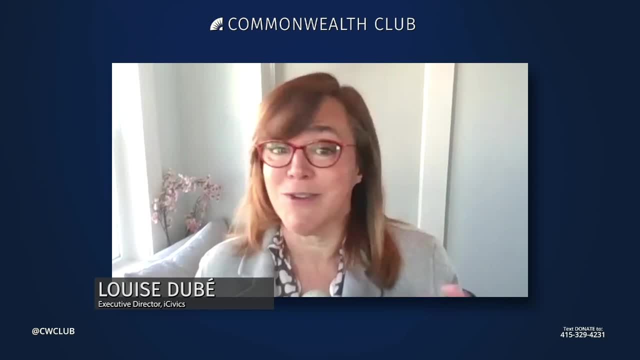 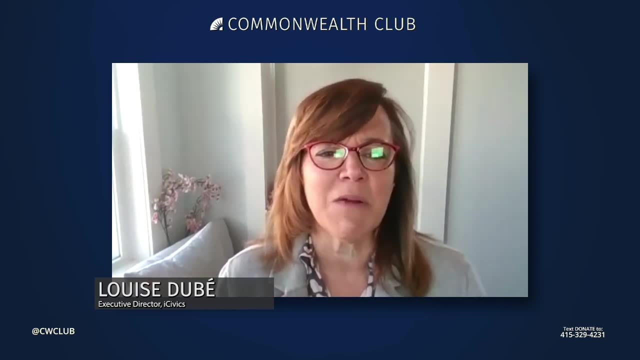 Canada. I wanted to come here since I was a little girl And for me America was this beacon of freedom, It was this pluralism, It was just a country of exceptional achievement. I understood all of its problems, but I also really believed, and believed that it was a democracy, that every 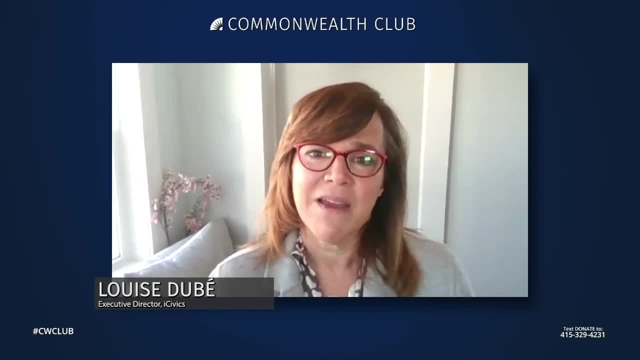 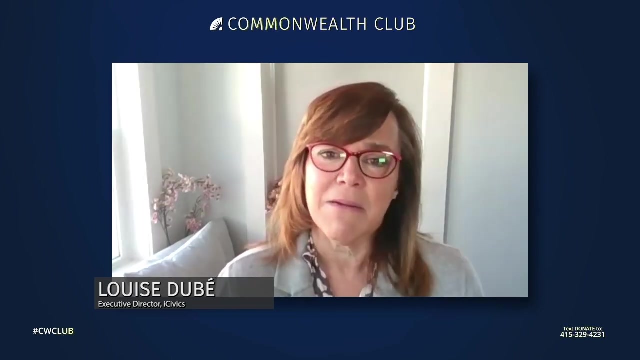 other country looked to as its, As the best right, And I think all of us ordinary Americans that I did it- took January 6th as a personal failure. It was like, really, I felt emotionally downtrodden by what had happened to our institution. It shook my pride And so a 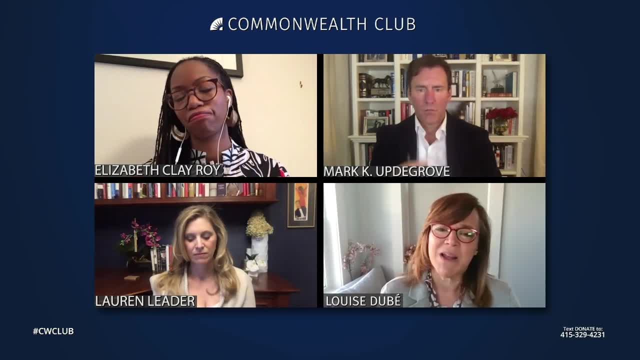 lot of people are saying how the heck did we get here? But I think, as Americans, we have to be more interested in how do we go away from here, how do we rebuild the civic strength of our country- and I think that's going to take all of us, And for that we have to look back. 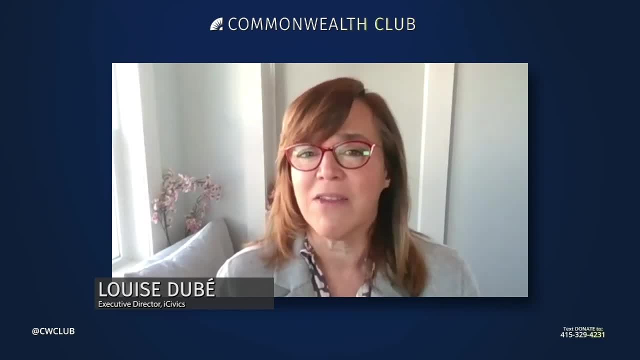 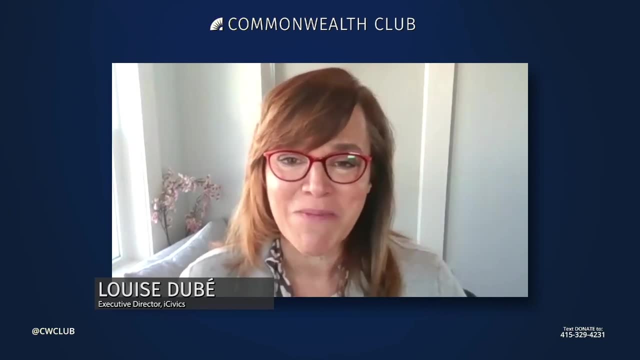 a little bit and think about the founders who really understand. they understood the dirigility of this country and they understood its resilience. I was actually talking to my mother yesterday. She still lives in Canada. She says to me I was so naive and naive and I had an argument. before. That's your friend's eyes. She'll react to me. later on She will ask me things like: no, actually when I was 15 or 12, when I was a 15-year-old and I assumed I was gonna be able to do all. the things that a story tells me. How important are these больш climate因為 issues. How interesting if many great JACKELORsche's? Because it's quite interesting to me think that the language and political. I was so impressed with these Americans. 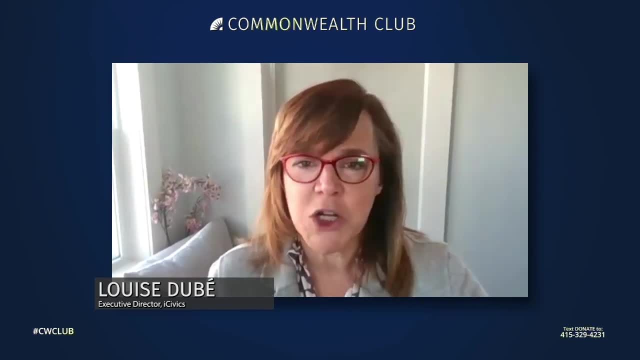 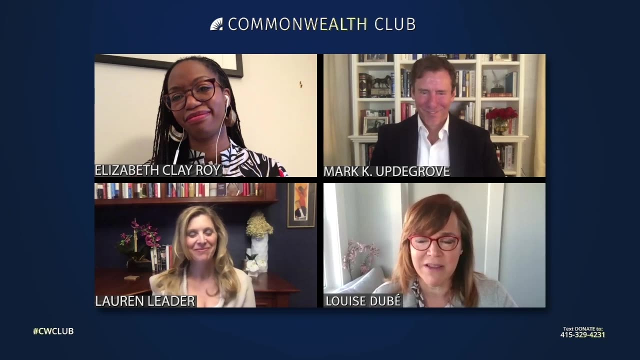 They dusted themselves off and they put on a great show. It was, and I always say: well, yeah, exactly, Americans can do this. So it is not to diminish the incredible divisions that are in this country, but I believe in. 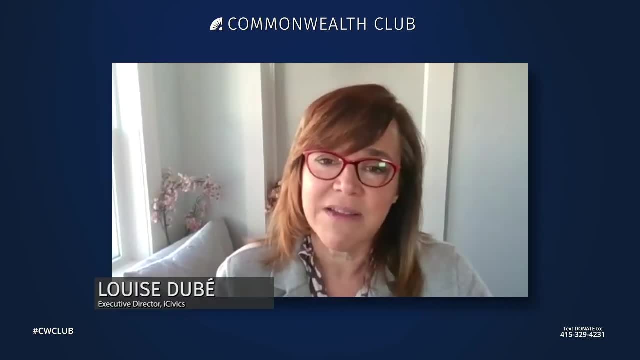 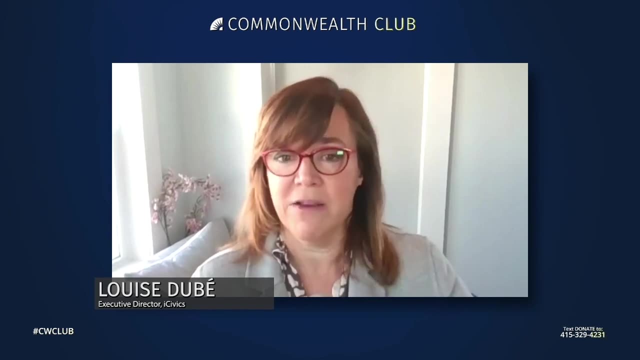 America, and I think we can do this, But the only way to do this? this is a country that is very complex. We have a structure that involves multiple layers of government. There is no one entity that's going to tell you the truth. quote unquote. 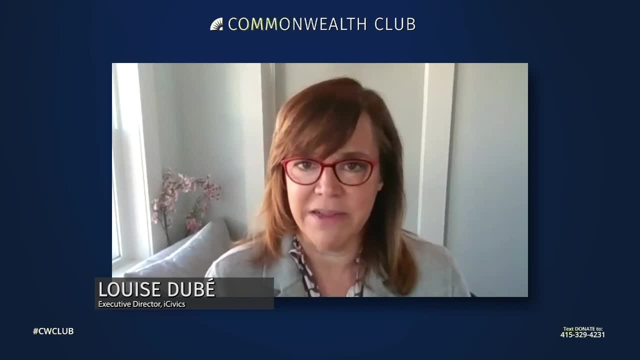 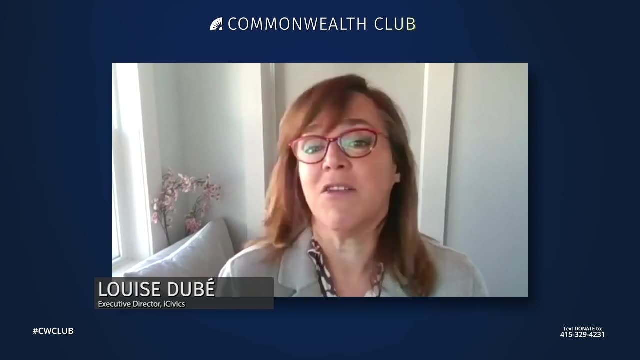 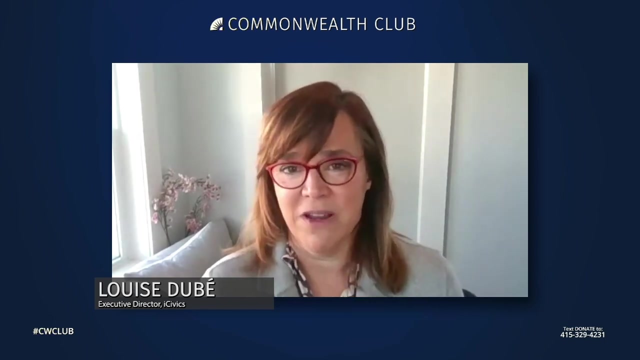 There isn't a way. Self-government is an institution that requires each and every one of us to understand how it works and to be able to talk to others. You don't expect other people to agree with you. You expect division. You expect that there will be debates and you just need to engage with them based on 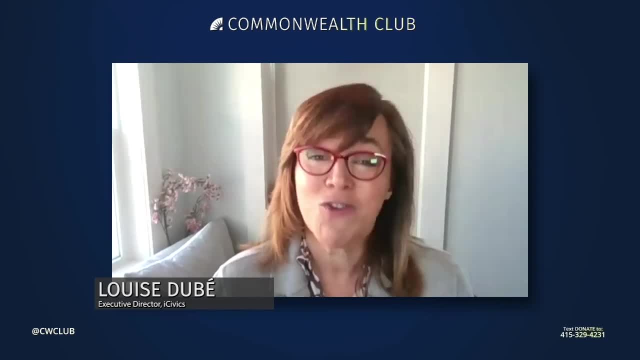 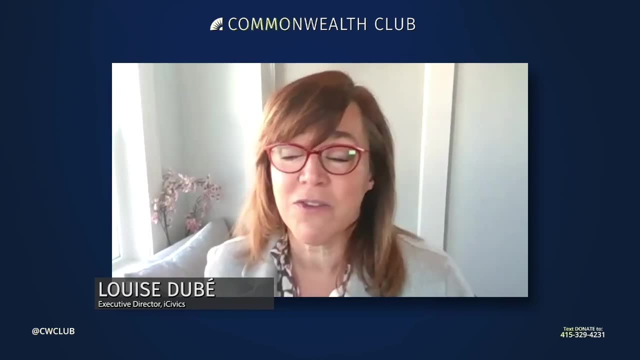 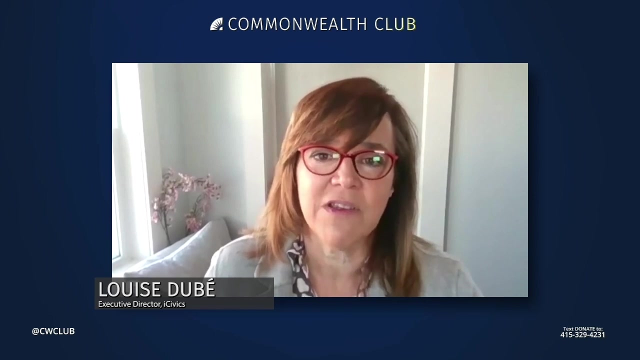 truth And that you cannot do without education And that it's a requirement of this kind of self-government. Our founder, so iCivics- was founded by Sandra Day O'Connor in 2006, after she came off the bench, and she knew this. 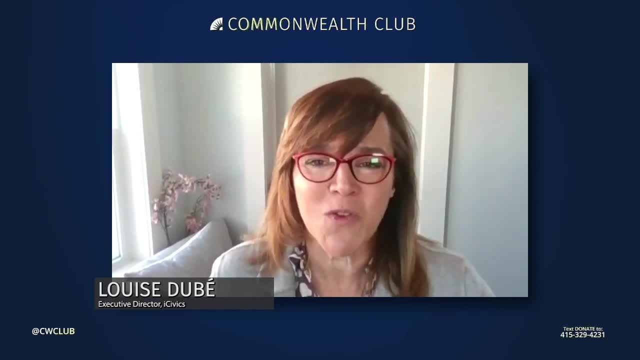 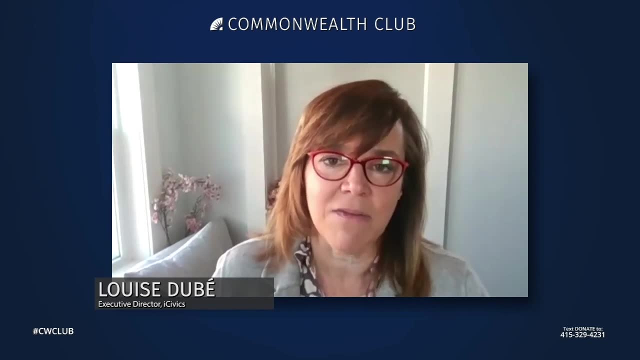 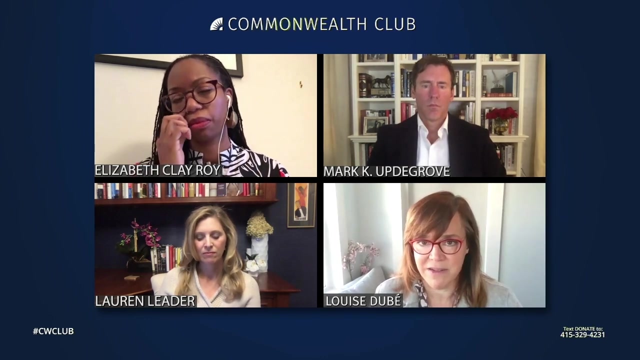 She said clearly: civic education and the rules of our self-government are not transferred from generation to generation. They're not transferred to the gene pool. You must teach it anew every generation. So that Is what we need to do. for decades We have disinvested in civics and history education. 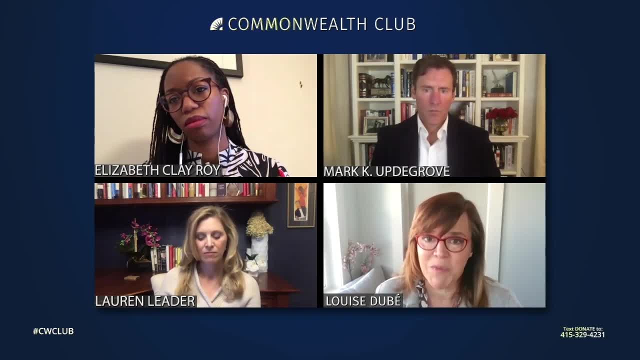 We perform at the lowest levels. It is not acceptable, And K-12 schools are a point of aggregation in which we can make significant change. But the only way to do that, as my co-speakers pointed out, is to invest in civic education. 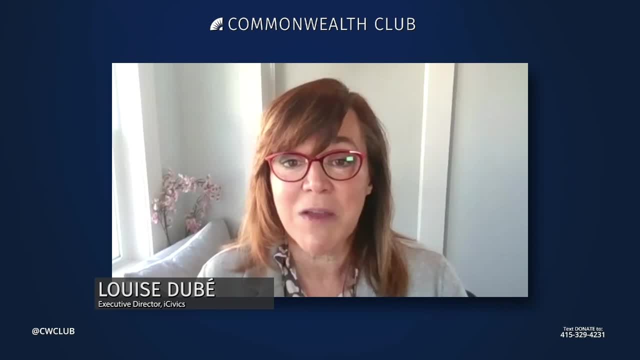 history and civic education. We need to take those, Take those things seriously. So in 2018, we, based on the legacy and the leadership of Sandra Day O'Connor, who unfortunately could no longer do that work, founded Civics Now, And Civics Now is what you do when you don't have any money. 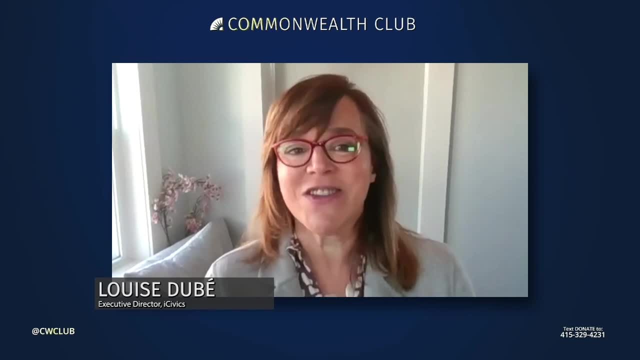 You band together and you do what civics teachers do, which is to organize together a strong force of cross ideological organizations. So it involves a lot of presence. It involves the Central Library Foundations, like the one that Mark represents. It involves Generation Citizen that we work with closely, the Center for Civic Ed, the 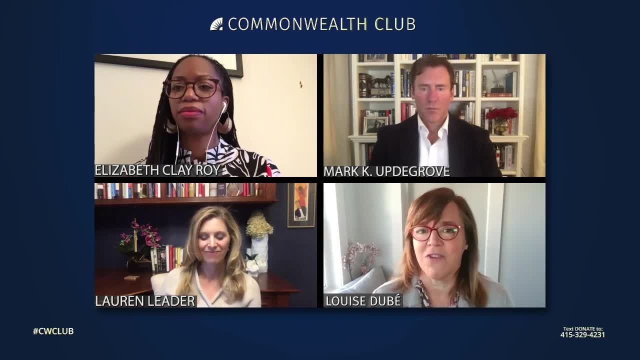 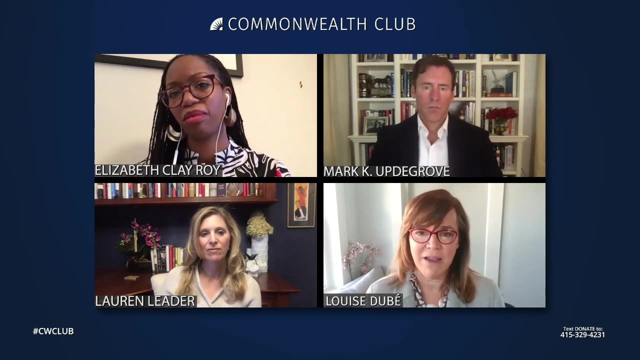 Girl Scouts of America. You're talking about a broad range of organizations that have the same goal: Prioritize civic education, Invest in civic education for our country's civic strength. This is not a political issue. This is an American issue, So we just have to be very clear about that. 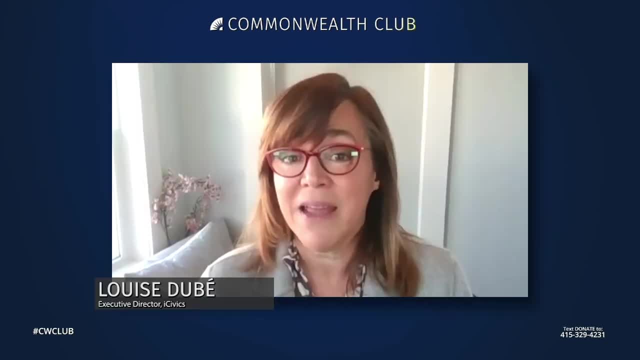 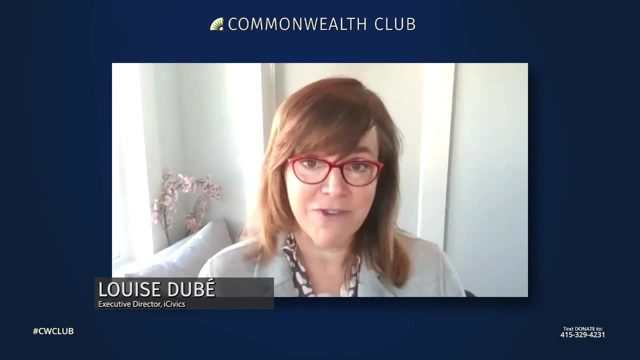 And then I represent iCivic, And at iCivics we have about 8 million kids every year come and learn on our platform. We're known for our games. They're all free, So parents and teachers can all come. 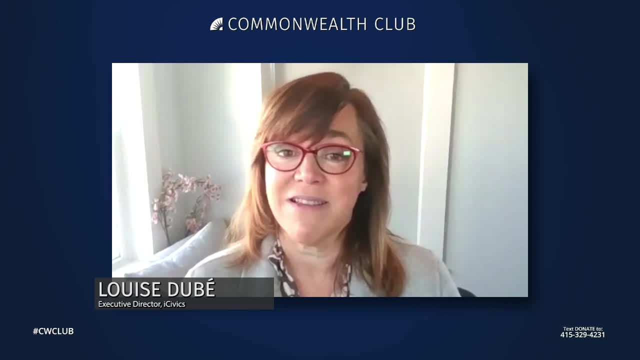 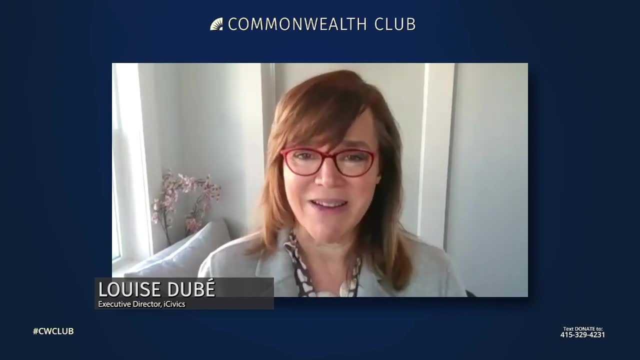 And you can play as though you're the president of the United States in executive command. You can see what that's like. You can run your own campaign to become president. You can be the county administrators. We have a new game in Texas, actually. 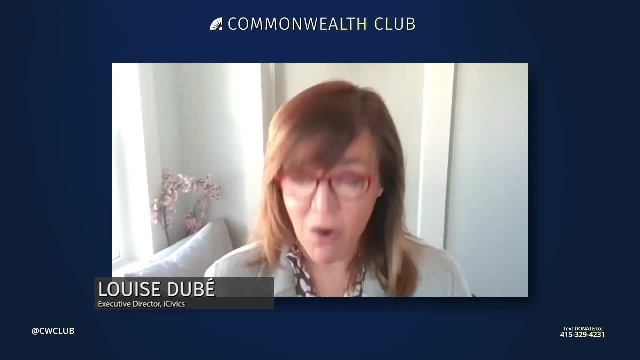 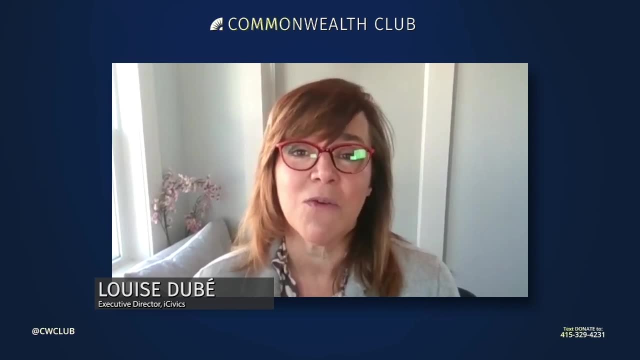 To be a county administrator in Texas. So all of those things are available. They're for free. But most of all, it is a community of educators. We have 120,000 educators. I think we underestimate the desire for educators and young people to learn about civics. 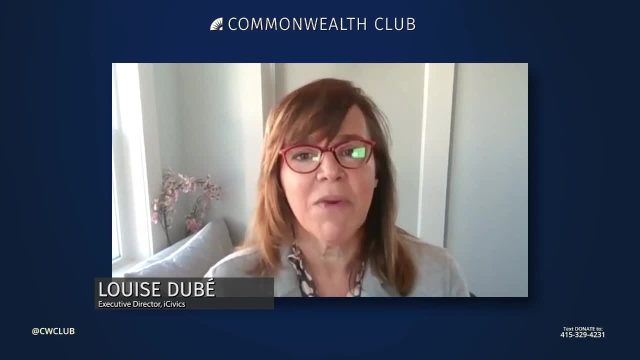 Yes, it is political, Yes, there is fear, But there is also a great deal of enthusiasm on the part of young people and educators And educators to do this work, And so what I hope will happen is that we allow January 6th to be the wake-up moment that it needs to be for our country. 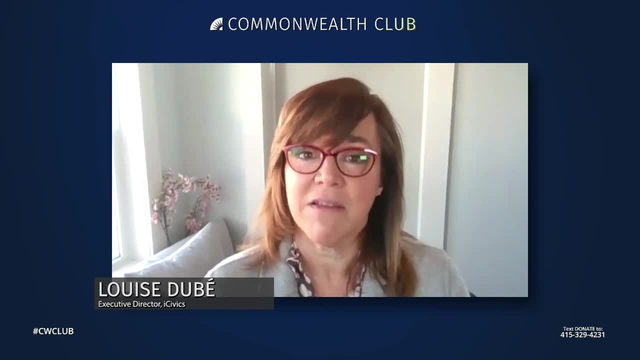 Just like Sputnik was a wake-up moment for us on science in defending our country, January 6th, the insurrection should be a wake-up moment that we need to return the investment. And I will make one suggestion as I end. 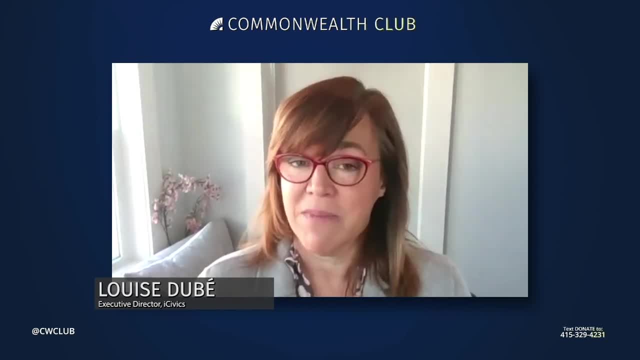 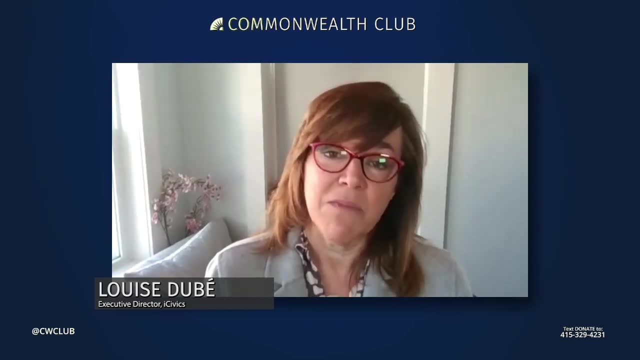 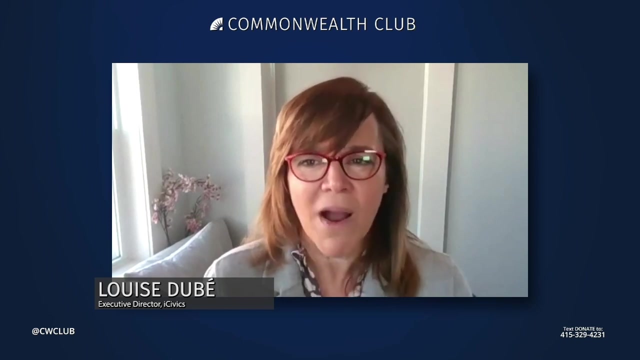 Which is that corporations- many of them- have paused or they've decided no longer to put in money in political pacts. They've made different kinds of decisions. Why not use some of that money to invest in civic education? Why not make a contribution to this country in that form? 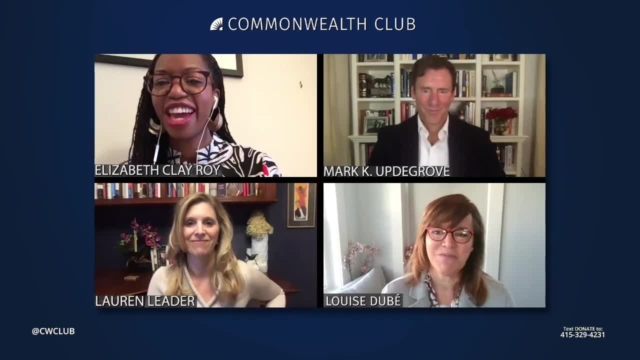 So I will leave that with that thought. Thank you, Elizabeth. Yeah, Thanks so much, Louise. You know So many great points for us to pick up. Thank you, Elizabeth. So many great points for us to pick up on and thread throughout our conversation today. 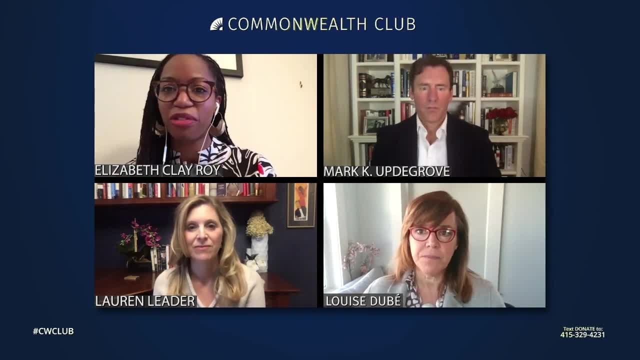 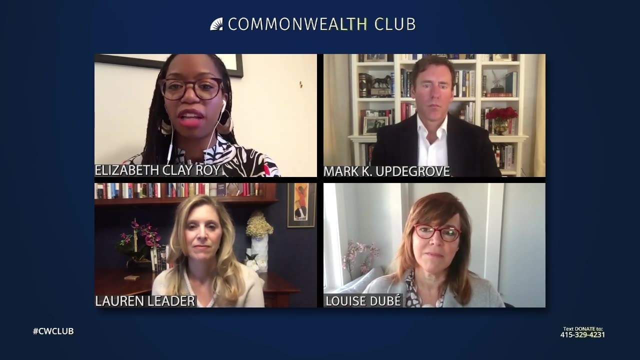 But, you know, sticking with some of those feelings, impressions, ideas that we were swirling with, sitting with on and after January 6th, Lauren, I want to go to you. What drove you and Mark to put pen to paper and share your perspective with the Hill. 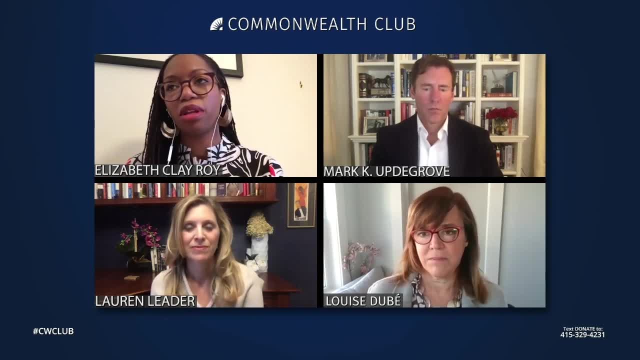 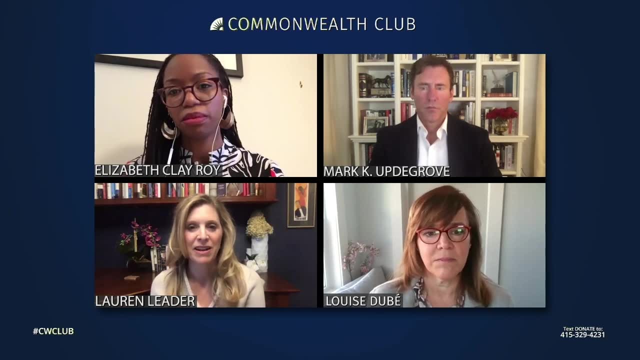 And how has your organization come about And what are some of the things that you've learned in the past and that you've been committed to the work of civics education? Yeah Well, thanks, Elizabeth, And I'm so admiring of everyone's work on this panel. 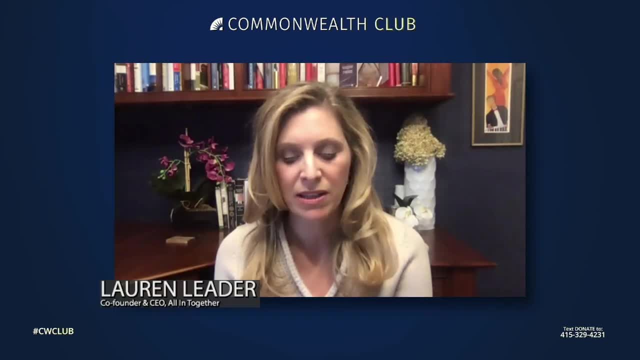 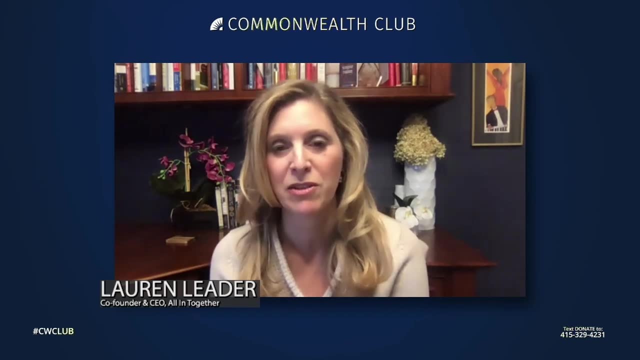 So All In Together was founded in 2014 because at the time, the United States was 54th in the world, according to the World Economic Forum, for the political participation of women. Last year, the World Economic Forum ranked the United States 98th. 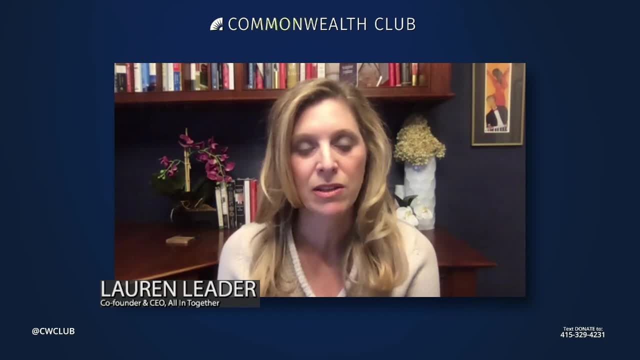 And one of the reasons for that is because of the political participation of women. I mean, it's obviously a political participation. reasons for that is partially the low representation of women in elected office relative to other nations, but it is also the low civic participation of women. So even though they outvote men, 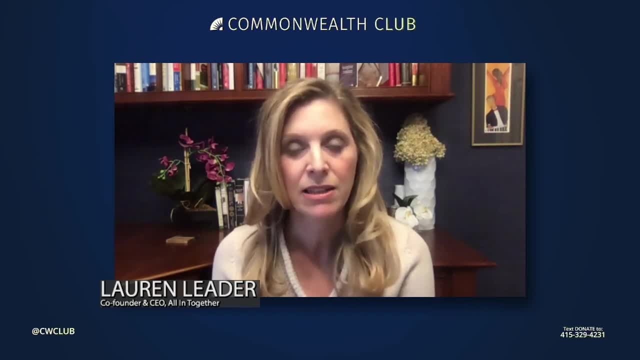 and they have outvoted men in every election since 1980, a fact that very few Americans actually know. even people who work in politics don't all know that. but women have, and they turn every election and they turned this last one as well. They have not historically been engaged in the 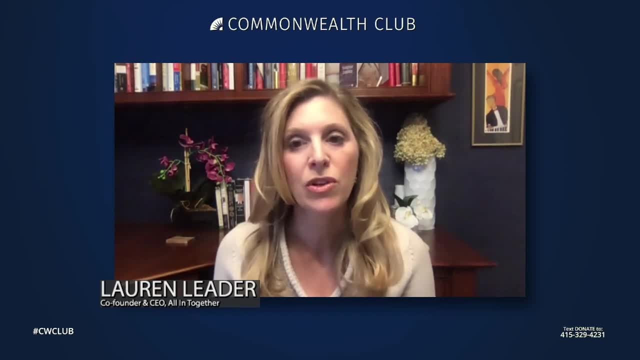 political process beyond the ballot box. They don't hold their leaders accountable for representing the issues that they've sent them to high office to work on. They are less likely to write to their members of Congress to engage with them, to partition their grievances, as is their sacred. 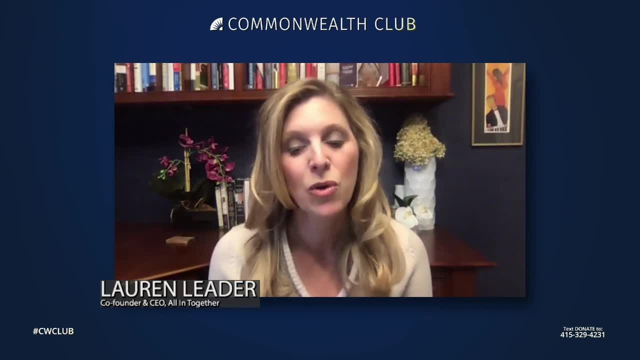 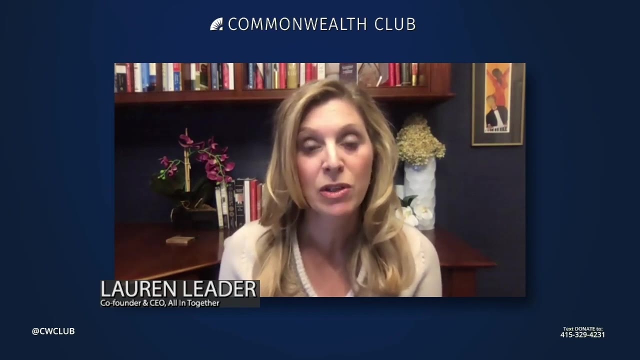 right as outlined in the First Amendment, And the core reason that we found was not any of the things that most people thought about why women weren't participating. The reason was that they felt they didn't know enough to participate, And Louise is right that there is a broad civic crisis in the United States: 70% of Americans. 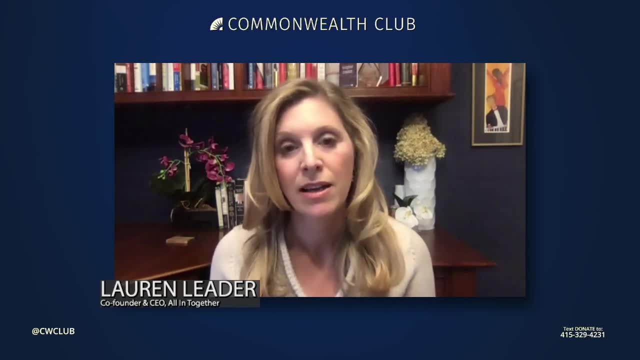 can't name a single person who represents them in Congress. Most Americans could not pass the civics test that is part of our citizenship exam. I mean, the list goes on. Americans do not know how our government works, But for women, that lack of knowledge which is actually about the same as men, 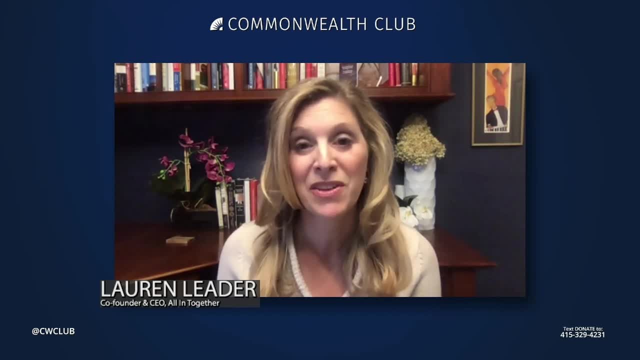 disproportionately keeps them out of participating. Women feel they need to know what they're talking about in order to participate, And I think that's one of the things that we need to do in order to participate. And I think that's one of the things that we need to do in order to participate, And I think 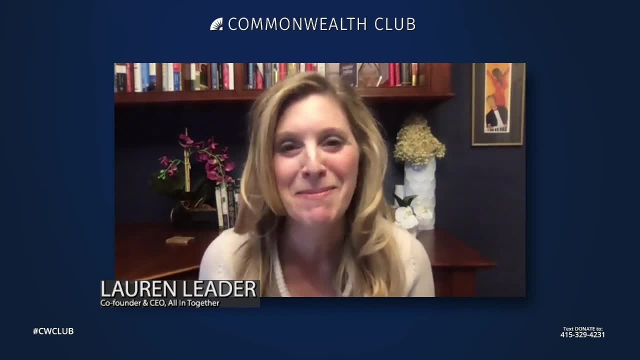 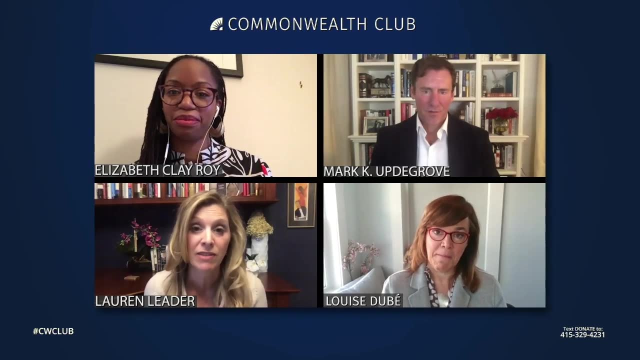 that's one of the things that we need to do in order to participate. I could make some jokes about gender differences there, but I will hold back. Women actually want to feel qualified and want to feel that they know, So our mission is to focus on adult civic education. Civics already existed. 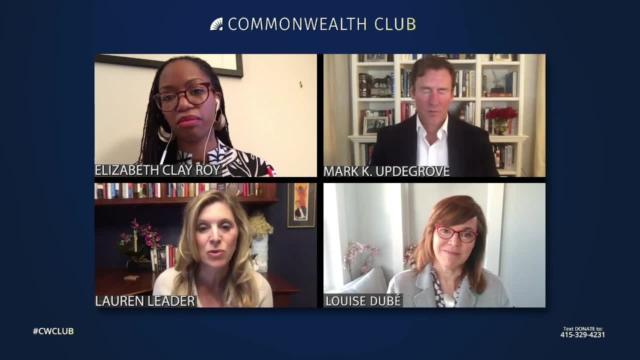 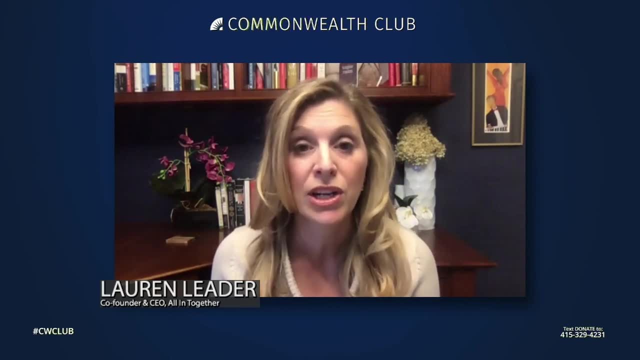 When we founded, we knew there were organizations that were working on this at the school level. We wanted to get to the voting age women across America who didn't have other resources to learn, And our goal is civic education for the purpose of participation and engagement, not just education for. 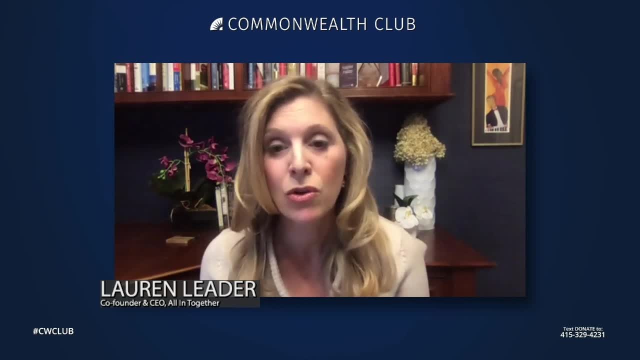 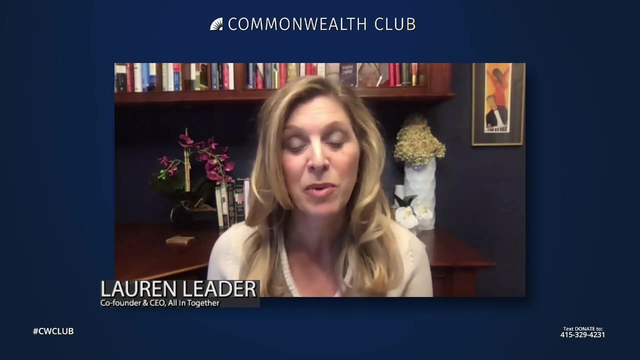 education's sake, but education for activism's sake. So just to answer your question about the panel- and I won't go on too long- but part of how Mark and I came to know each other and our wonderful friendship is because of a fantastic civic-related program that was founded by the 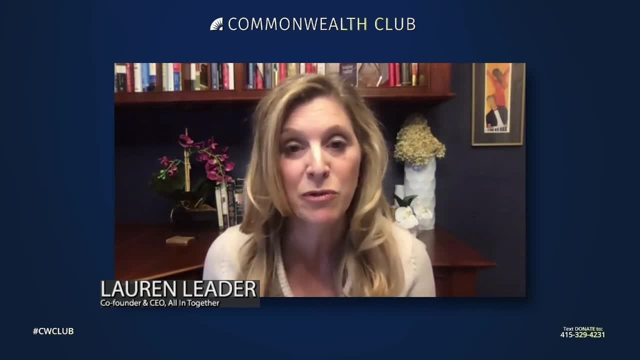 presidents, former presidents and presidential libraries- President Bush 41,, President Bush 43,, President Clinton- in partnership also with the LBJ Library, which is called the Presidential Leadership Scholarship, And I think that's one of the things that we need to do in order to participate. 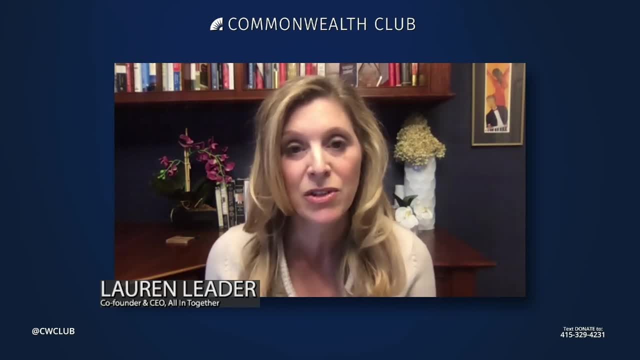 So we have a $1,000 program, which is a very special program that they built together to try to starting in 2015, to foster the future civic leaders of America, And I was lucky enough to have Mark as one of our faculty at the LBJ Library as part of that And part of what that experience. 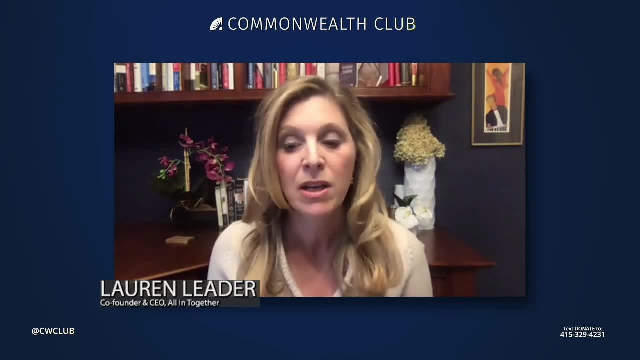 taught me, as somebody who works on these issues all the time, one is that when we talk about the importance of understanding civics, I actually really believe that understanding the history of our presidents should be part of that, That learning from you know. 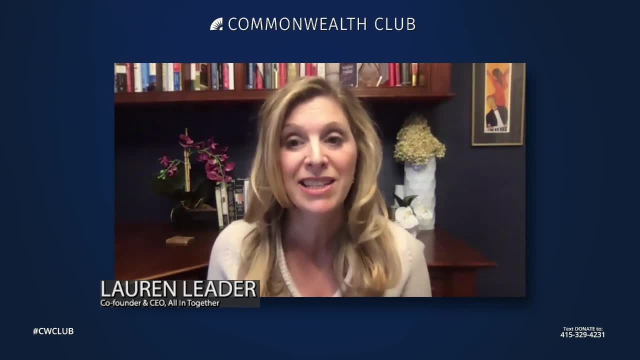 the recent and distant past is essential to understanding the present. There's so many parallels from 1968 to now, which I will let Mark talk about because he's the expert on that. But as we've talked about sort of what are the remedies for the divisions in this country, 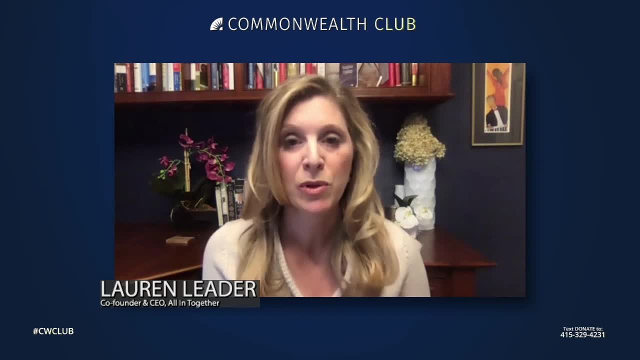 at the core. the president was able to exploit the ignorance of Americans to persuade them that their vote did not, that their votes were falsified, that the election was rigged. He but he has done that. he was able to do that. 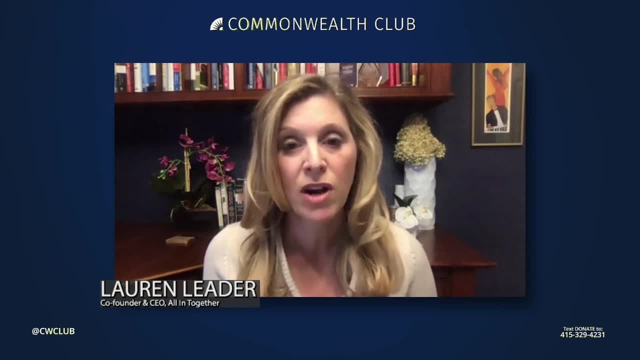 throughout his presidency. He did it during the impeachment trial. the first time. Really, at every turn, you had somebody who exploited civic ignorance, exploited ignorance of the core principles of democracy: the separate, equal separation of powers, three co-equal branches. 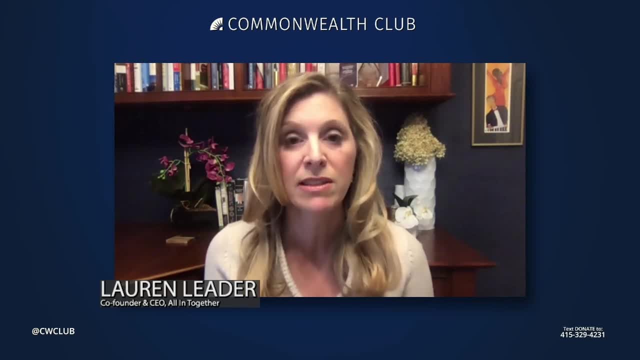 of government, the right to petition your grievances, All of the freedom of the press. The president was able to persuade millions of people that those were, that those did not matter because they did not know better, And our view, as Mark and I talked about it, was that obviously look, white supremacy. 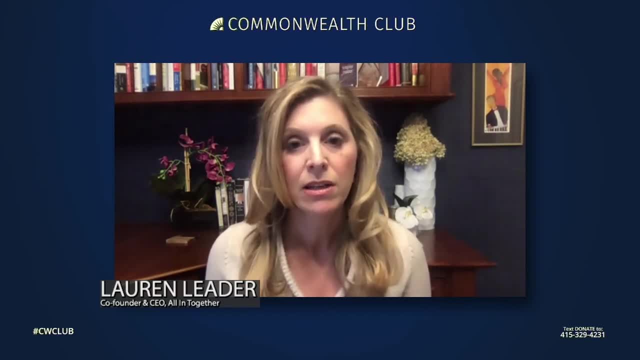 hate, anti-Semitism. these are deep-rooted issues in our country. You know we've been talking a lot about the recent past. I mean, look at Tim, we knew this was a coming. Timothy McVeigh was a white supremacist who took down the building in Oklahoma. 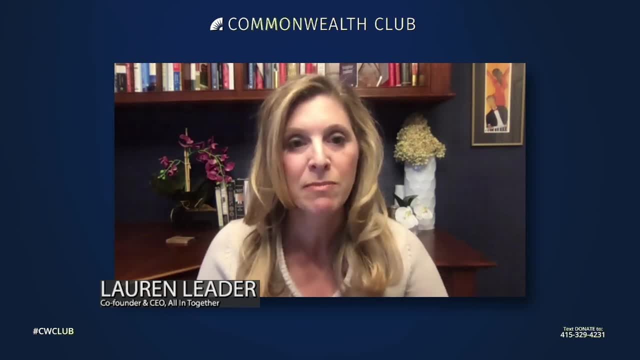 it's now more than 30 years ago. That was one of the first major, you know sort of recent terrorist, white supremacist, terrorist attacks. We've failed for years to take seriously the threat of white supremacy in this country And that is what was behind the six, But also 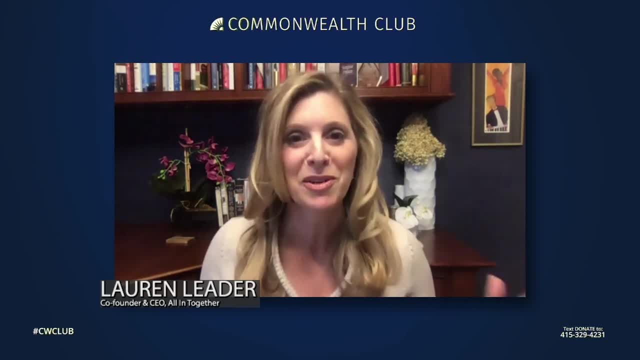 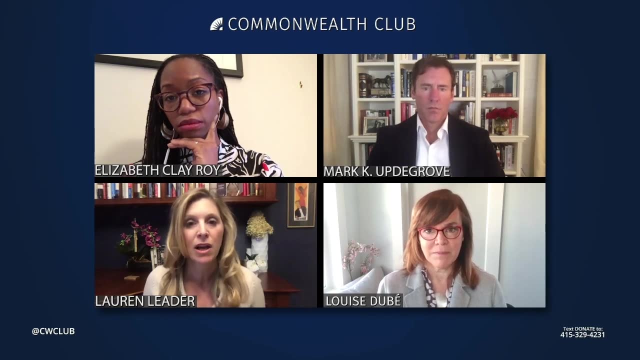 and so that I put in a separate category from just Americans who need to learn more about our institutions. right, Those are hate-filled, loathsome people who should go to jail, And I believe they're mostly beyond redeem. I don't think that's worth investing a lot of time. 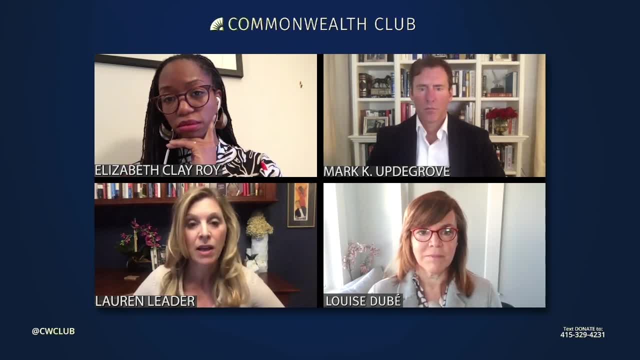 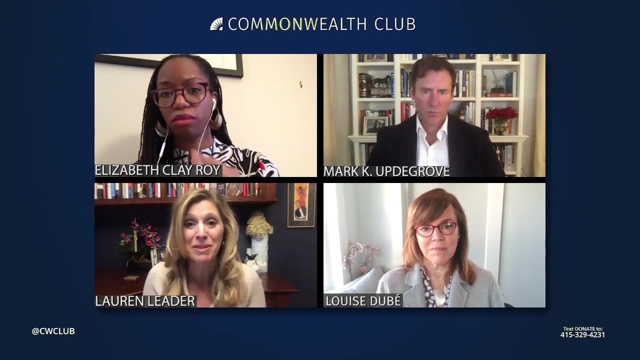 to try to convince white supremacists not to hate you or me. On the other hand, there are 75 million Americans you know who were willing to support a president who fundamentally opposed the core roots of what it means to be American, who opposed democracy And 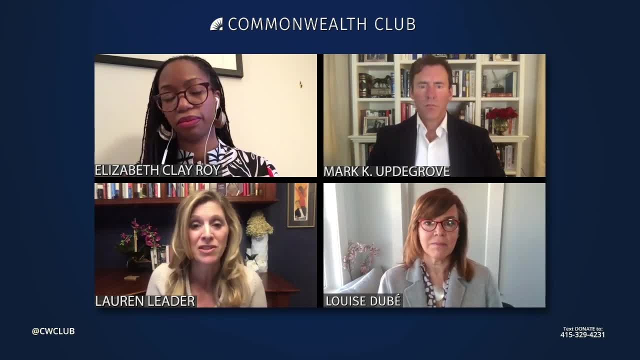 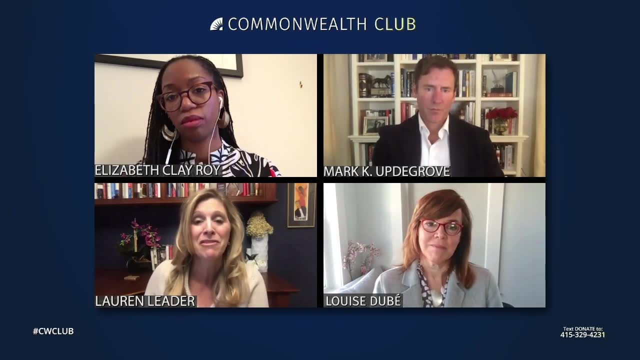 that can't happen unless people have a fundamental misunderstanding of what it act, what the flag I'm wearing actually means, what it actually means to be American, And the idea is that there were people carrying an American flag into the Capitol in order to try to overthrow the government. They 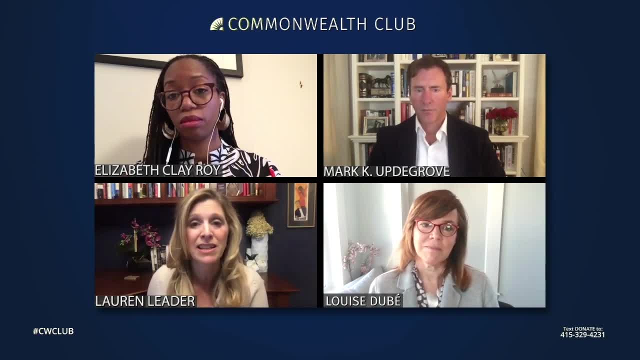 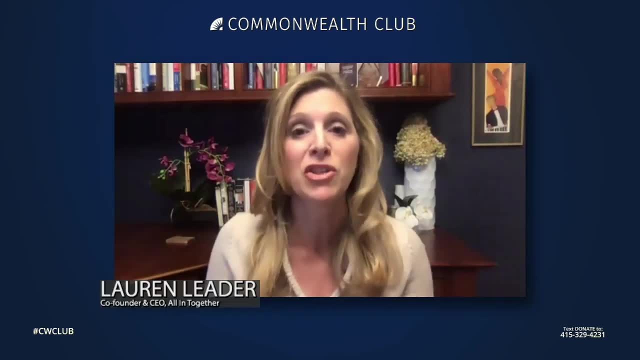 were also carrying the flag of a president who. that's not who we are. That's just fundamentally not what America is. to worship one leader, I mean. all of this is just the antithesis of what America means, what democracy means, what generations of people have fought and died to. 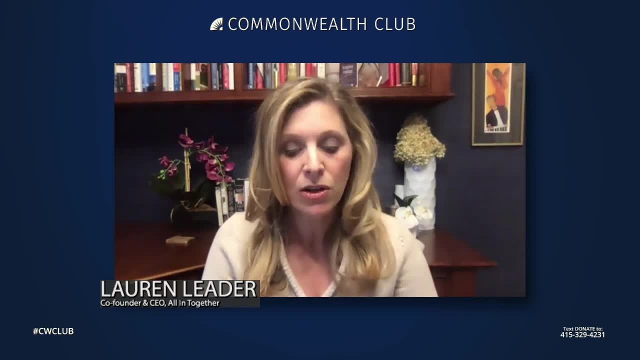 protect. So that's what I'll say about that. I think there are endless ways in which civic education matters, but there have been a lot of warnings about this over the years And we saw in this presidency. you know, and this is not about party, This is about 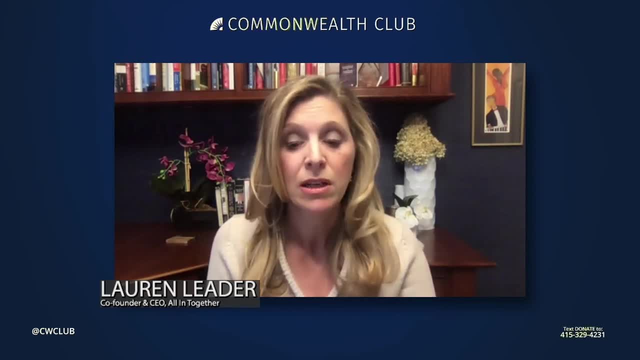 democracy. We saw in these last few years how possible it is to completely break down the core. We throw around the word democracy. People don't know what it means. They don't know what it means And that is why you can have that is what makes it possible for. 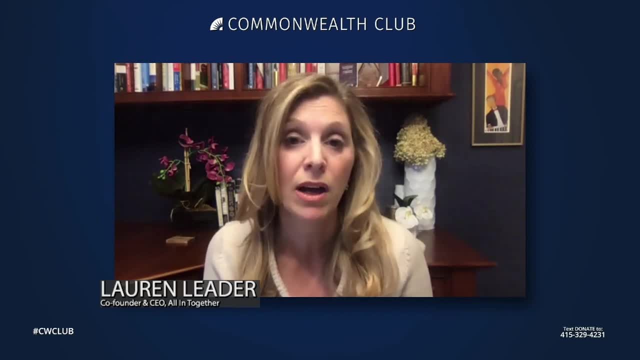 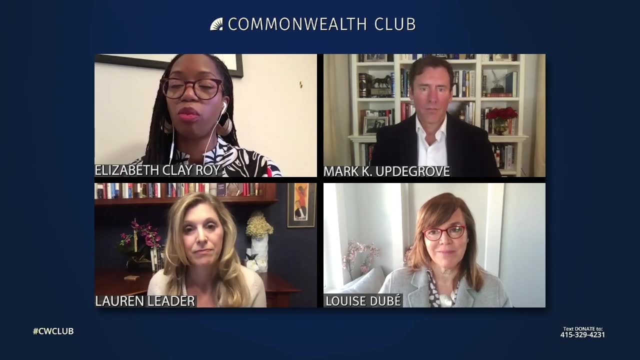 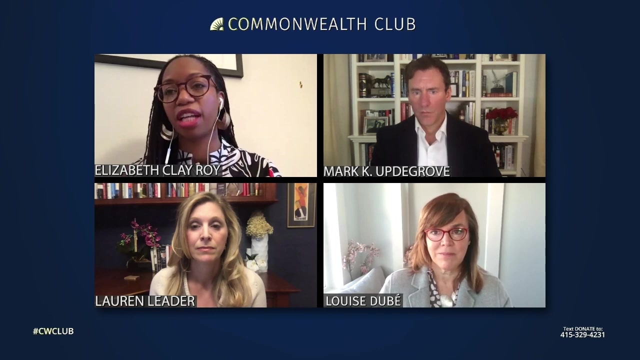 malintend to rise. Yeah, Thank you so much, Lauren, And you really lifted up with the way in which our recent history should have been more of a signal, for you know the really awful developments of the sixth And I know I've certainly spent a lot of time over the last few weeks reflecting on. 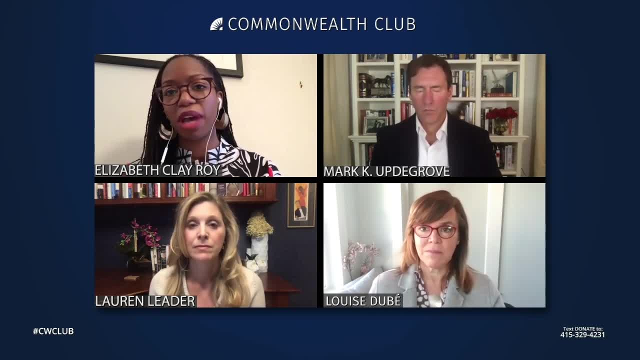 our history since then. But I think certainly we still keep up with the lessons we learned when we the Civil War, in thinking about the ways in which we have insufficiently, you know, addressed some of the underlying tensions that are still so deep and so clearly at play. 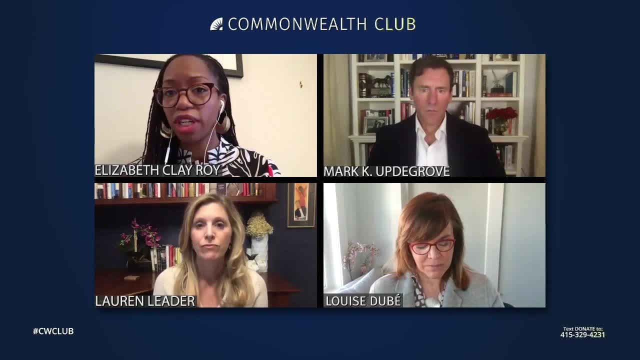 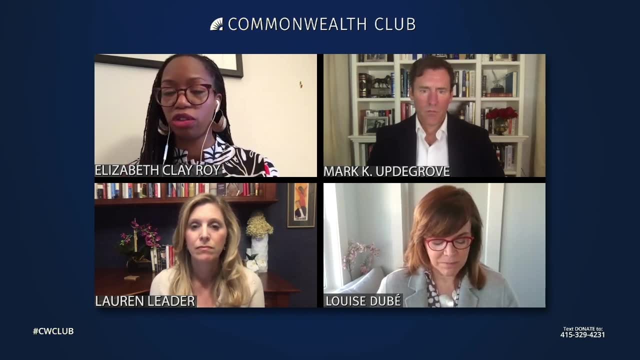 And Mark, I want to come to you as a historian and, you know, a leader of a presidential library, eager to hear you know what some of your reflections were. you know about the Sixth- and led you to want to really highlight civics education as one of the critical areas. 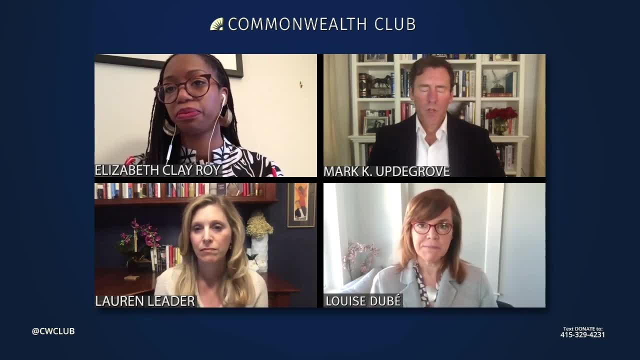 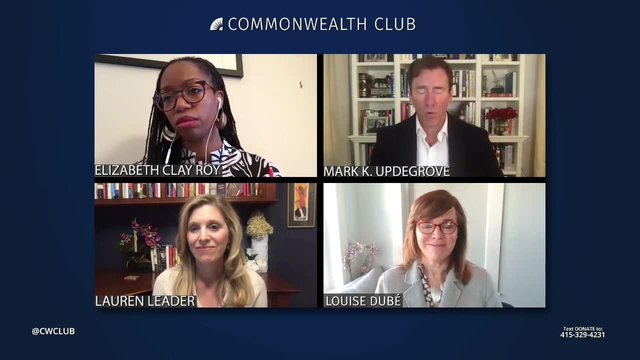 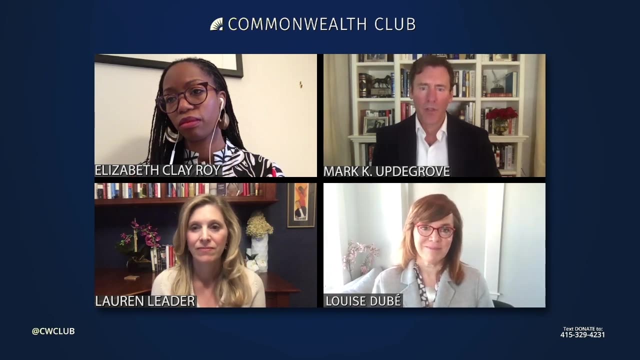 in which we need further investment and attention. Sure, And I want to thank the Commonwealth Club for having me and to thank you, Elizabeth, and Louise and Lauren, for the very good work you do. You know, I'm reminded, Elizabeth, of a conversation I had with Bill McRaven, who is the former. 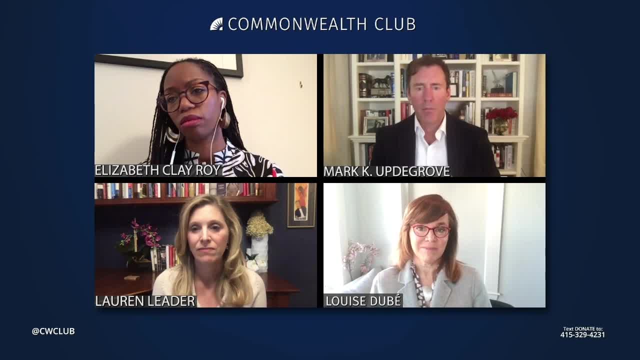 commander of Special Forces several years ago. Bill was the one who took out, who led the mission that took out Osama bin Laden, and then went on to become the chancellor of the UT, the Texas University of Texas system, after his iconic make your bed commencement speech that so many of us recall. 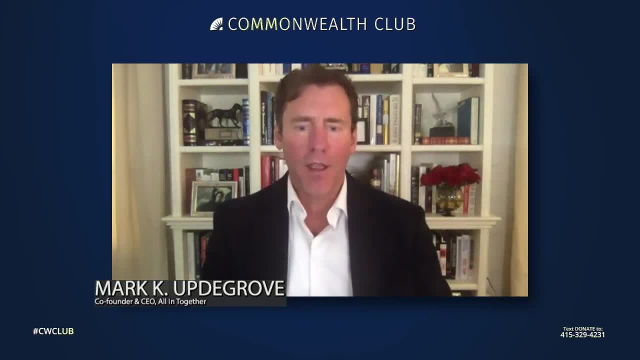 We were- this was a couple of years ago- at the LBJ library and we were waiting for former Vice President Biden to come and I was to interview him For an evening at the library. he was late due to his his flight had had technical problems. 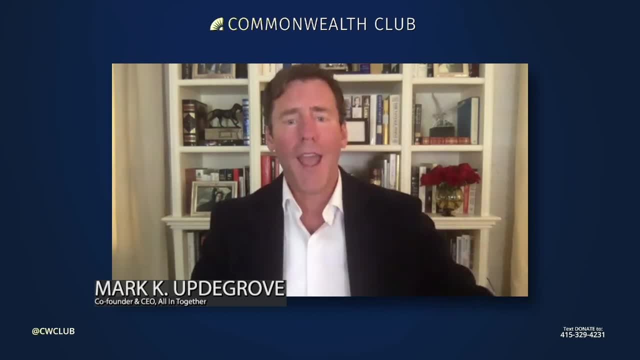 And so he was late to the interview. So we had Bill McRaven there. He's a friend And so he and I did a conversation for this large audience of 1000 people or so before the former vice president arrived, And I asked him what I thought the greatest national security threat to America was. 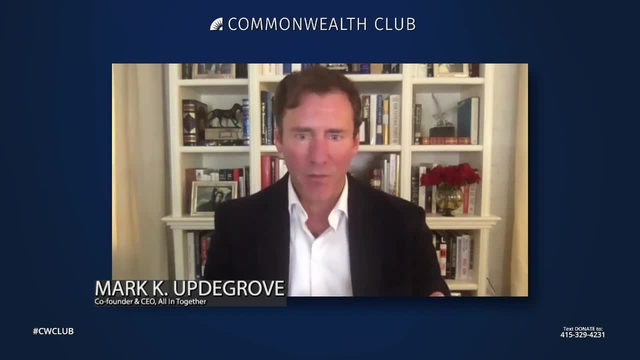 And he didn't talk about North Korea. And he didn't talk about Iran, And he didn't talk about Russia. He talked about our education system. Our greatest national security threat was our faulty education system And, in part, if we didn't educate our citizens, our young students, better on what our system of 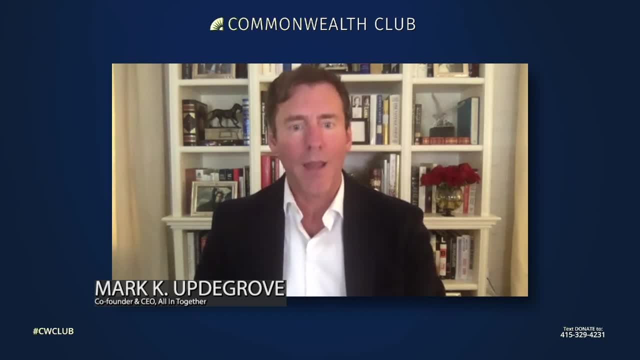 government is, then there would be a major threat And we saw that threat come to bear on January 6th- Earlier this month- in the most memorable way, and I will re quote Louise, who said: it shook my pride. it not only shook my pride, it shook me to my core. I love this country. I love what it represents. 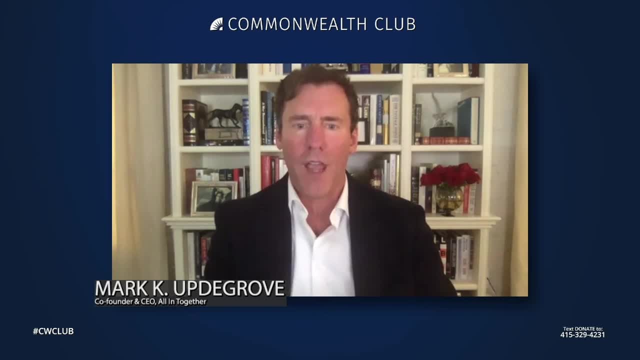 But we are only as good as holding up our ideals and what our government means, and we need to educate our students on on what America is And it's at its basic core. I mentioned to you before we did this session: as a young elementary school student I had a social studies teacher who was during the Watergate hearings, would wheel a TV into our classroom and show us the impeachment hearings for Richard Nixon. 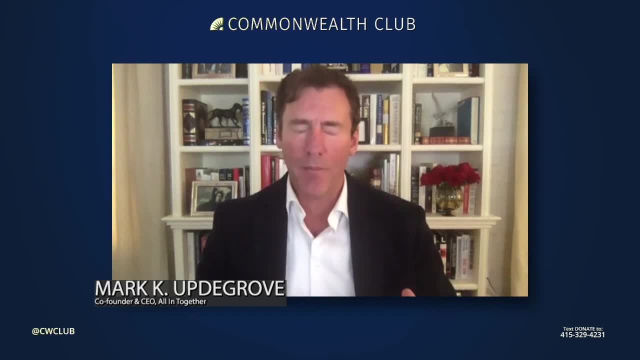 And I really didn't understand what that meant at the time. But I was left with the impression that Republicans and Democrats alike Were deeply concerned with the abuse of power of our president. So I was looking, I was watching the balance of power play out on my television set. 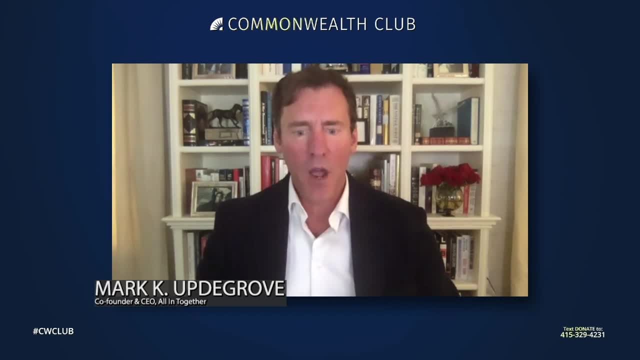 That's all I needed to know as a young student, to know that there was something bigger at work here. There was something keeping the president of the United States in check, And it was a very, very powerful idea And it got me really interested in the presidency, which probably led to where I am today. 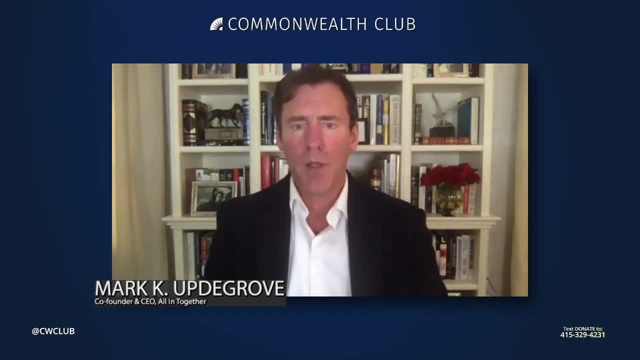 And I'll finish off by saying that one of my favorite quotes is from Harry Truman, who said: the only thing new in the world is the history you don't know. And that's, I think that's. that's very true. It doesn't necessarily repeat itself, but it rhymes. 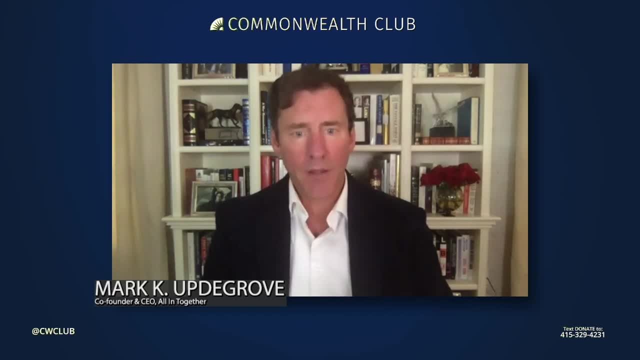 However, we have never seen a president of the United States try to sabotage an election And stage a coup against our government, And to go back to the point that Lauren made to see these ostensible, these people who call themselves patriots storm the citadel of democracy in the name of taking back their country. 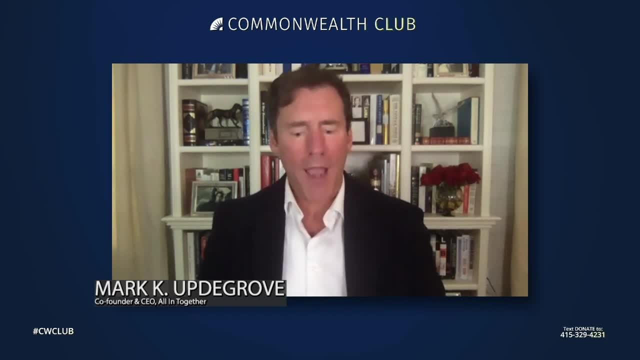 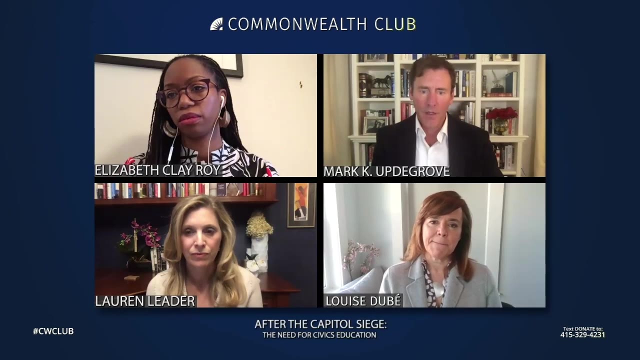 Something is deeply wrong You have to go back to. there's nothing like that in our country. You have to go to Nazi Germany or fascist Italy to see something that's similar Rather. so this is a wake up call. This is cold water in our face to remind us of the urgency of educating all citizens on what being America, being an American, means, so that we rally around a common identity as Americans and, hopefully, a common purpose. 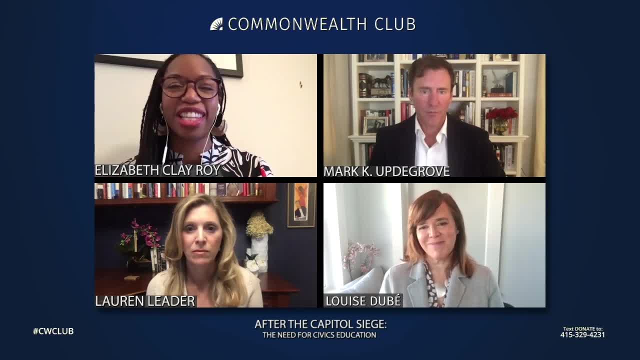 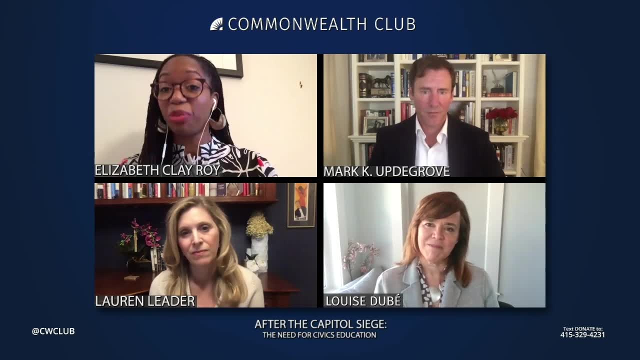 Yeah, thank you so much, Mark, And I want to share something that came up for me from your comment And then take us into the direction of asking each of you to talk about who else we need at this table. Right, Because we're all in. 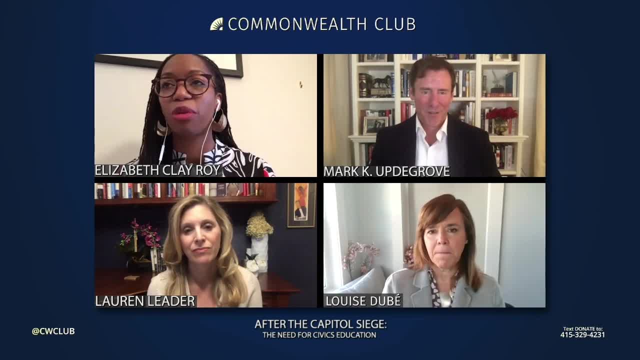 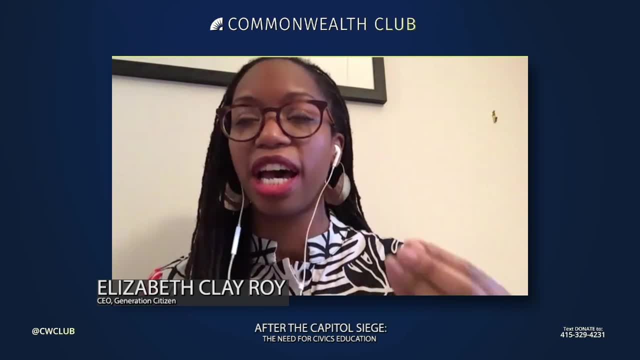 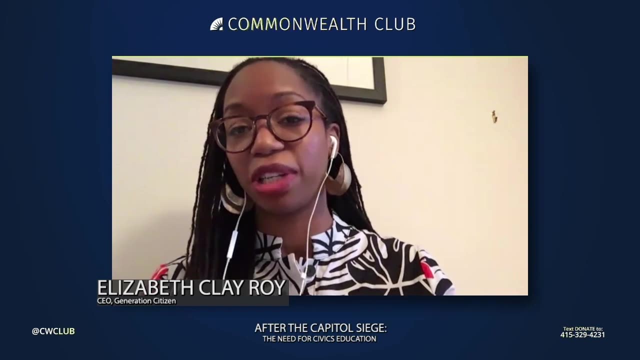 We know how important this is, but we've got to get more people involved to move this forward. One piece, though, you know that has been shared, and I think it is important that in this moment, we have been able to look through history and, globally, to look for potential equivalence, because I think that's important in helping us frame the 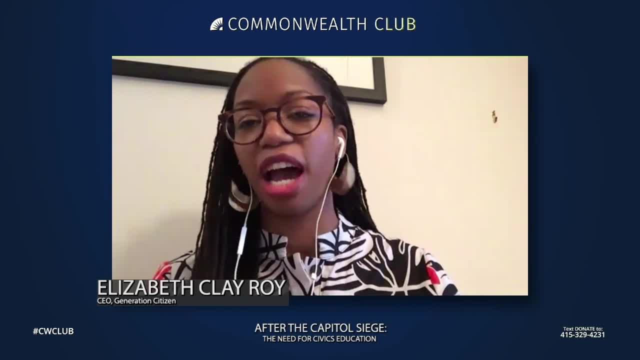 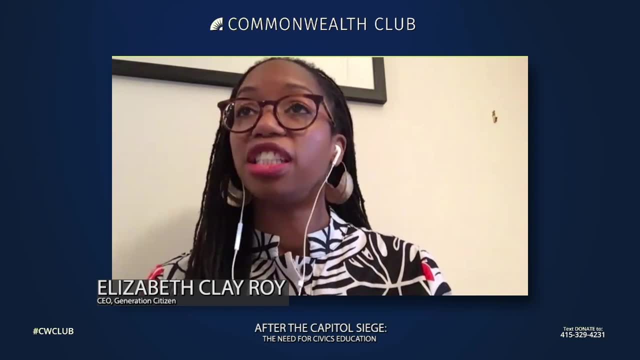 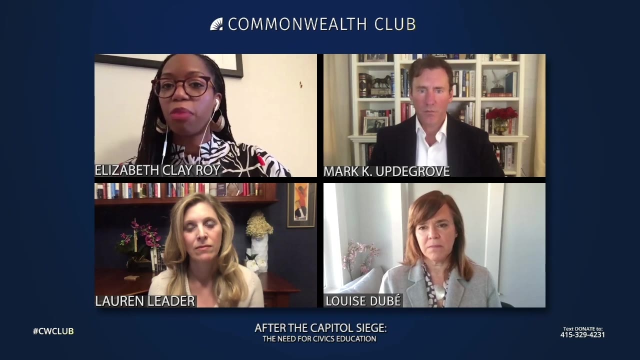 Gravity of the moment and how large our response needs to be, which I think is important in terms of the comparisons to fascism in Europe. the other place where I think it's important to look- just as we're looking back to 1918 and 1919 around global health- is looking at the post Civil War period. 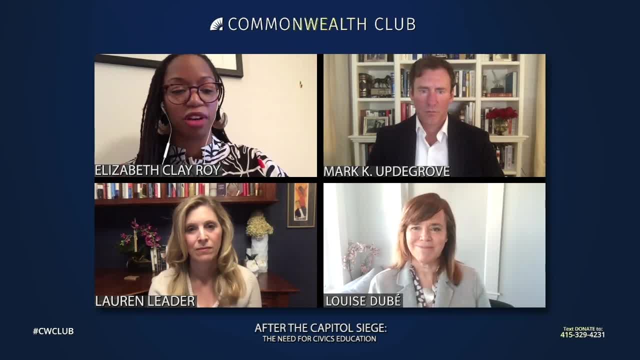 I grew up in Boston but have roots in North Carolina, and so I've actually been learning a lot more about the Wilmington in North Carolina insurrection of a US military, And I think it's important to look at that. And I think it's important to look at that. 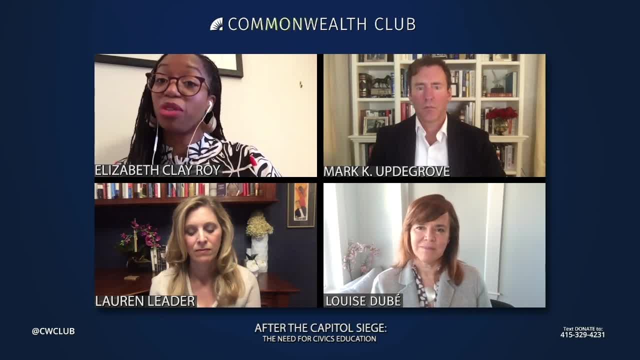 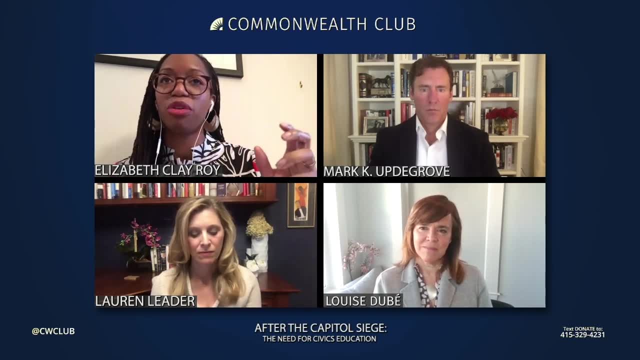 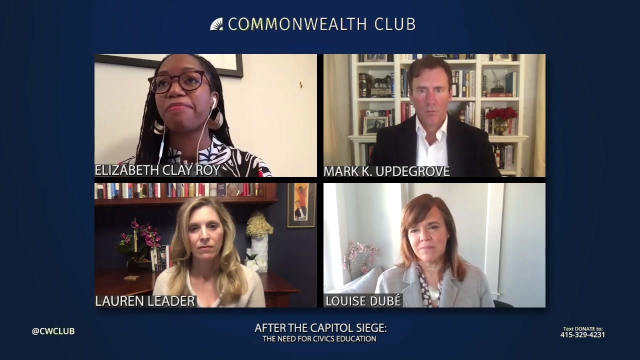 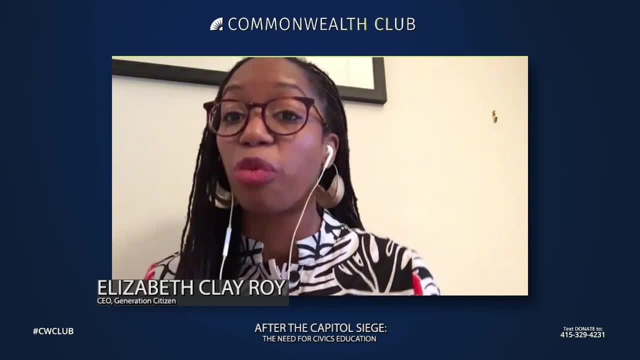 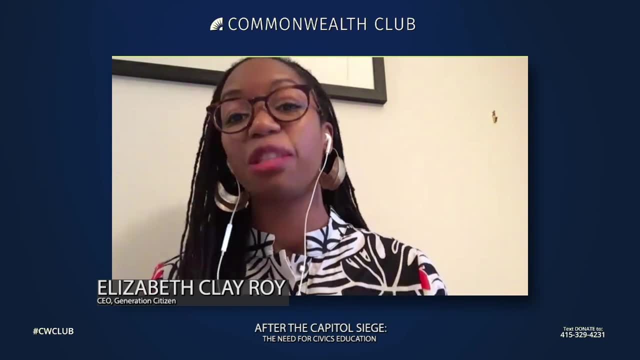 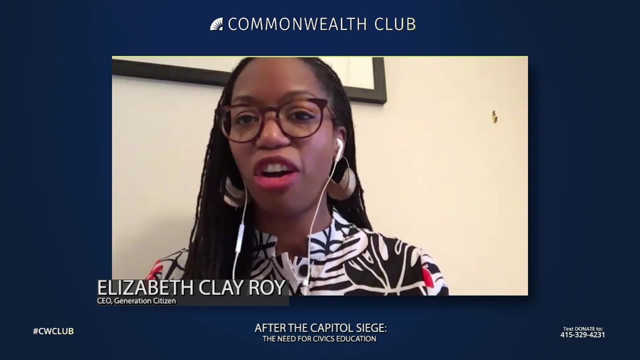 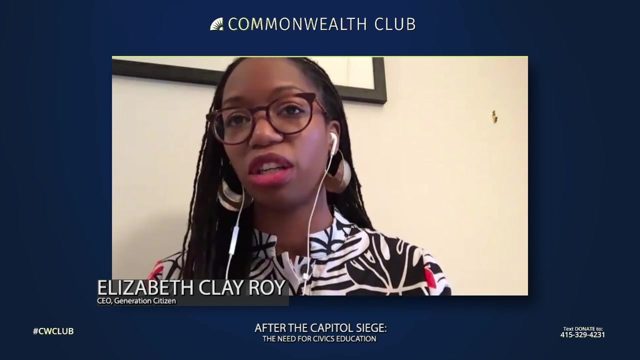 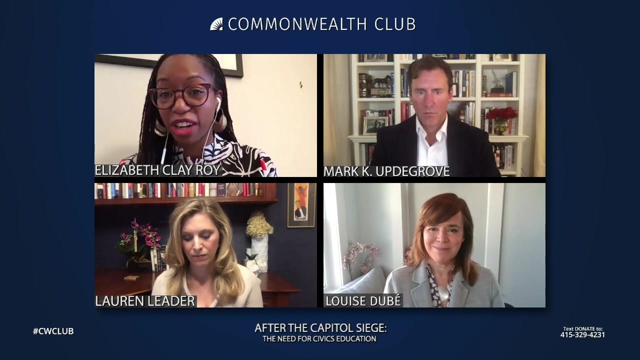 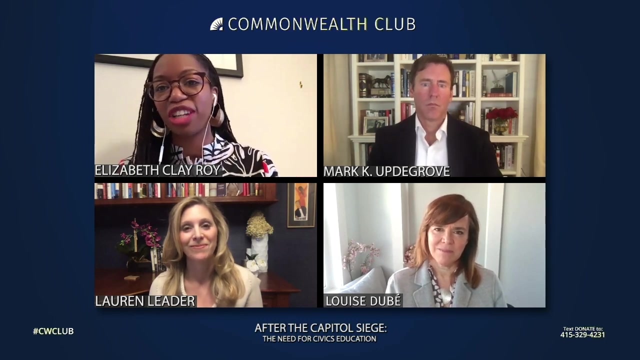 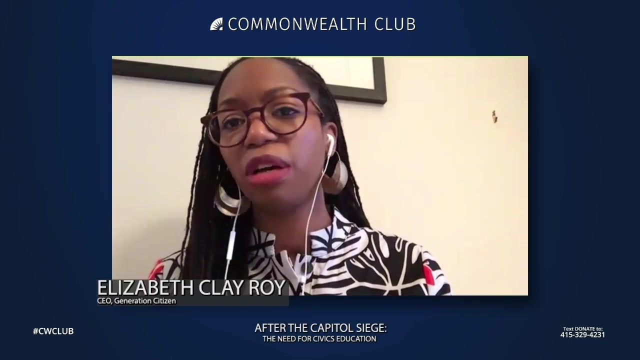 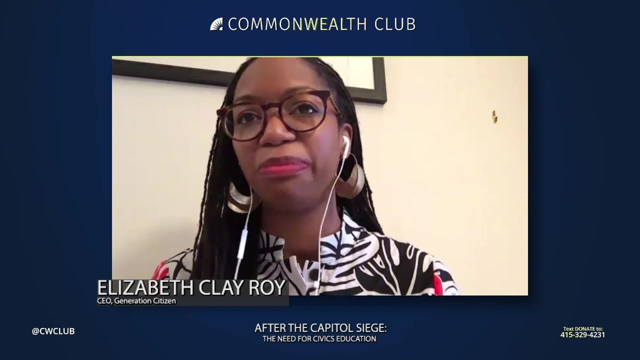 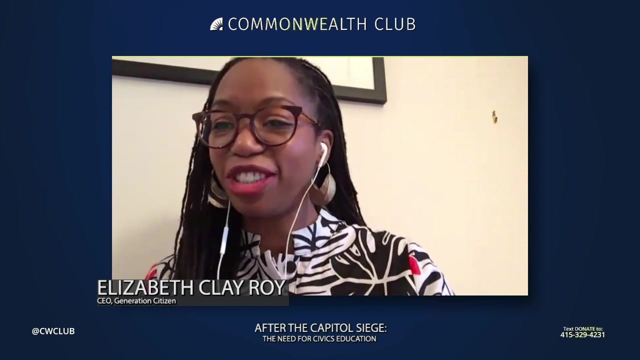 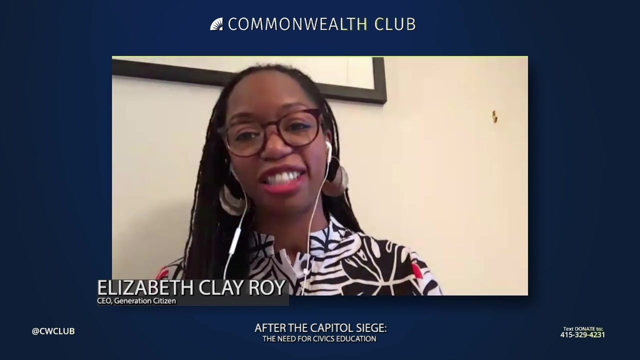 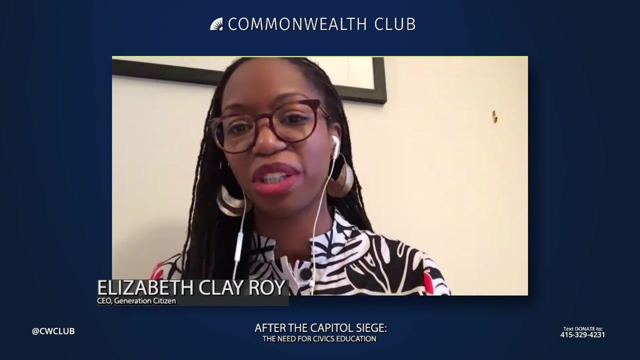 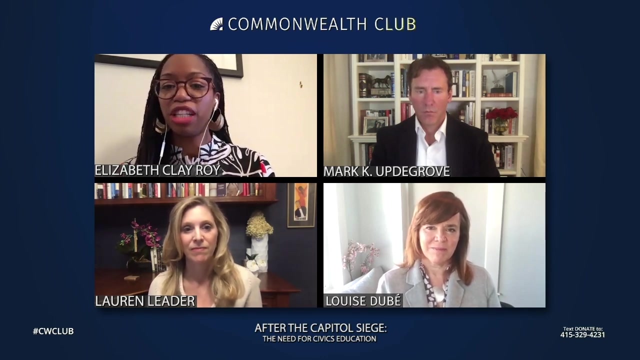 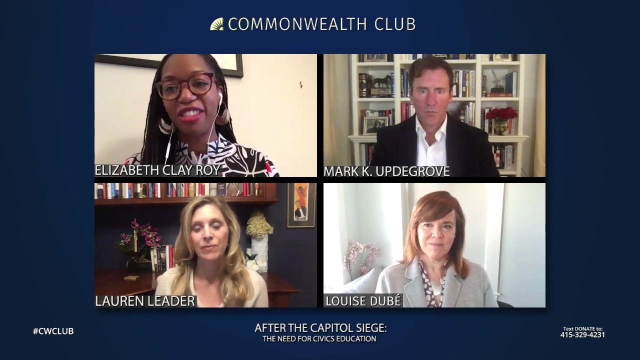 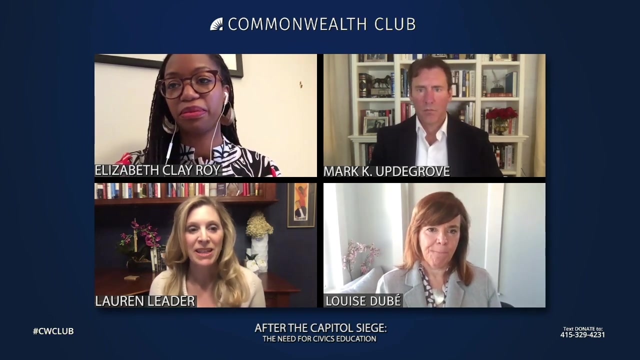 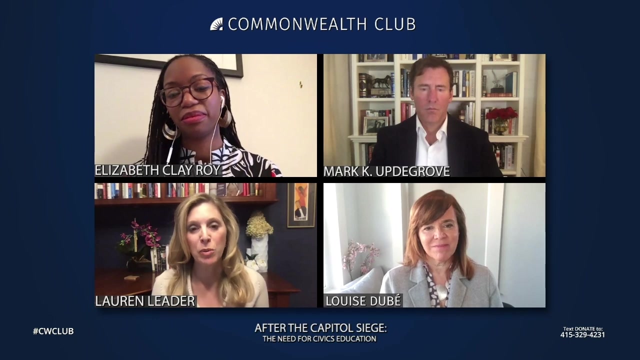 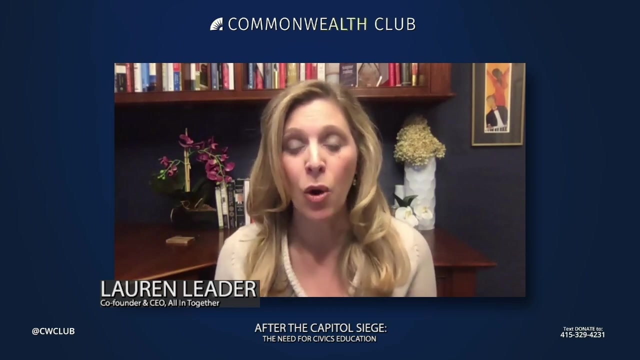 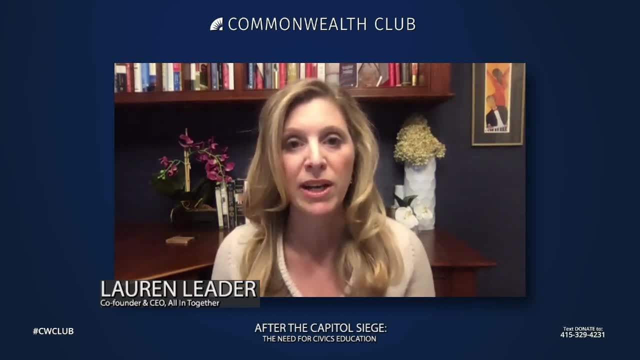 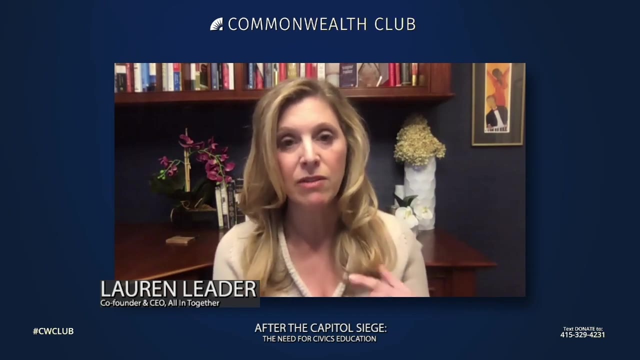 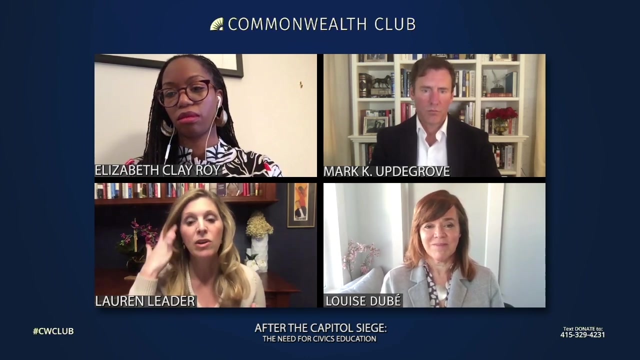 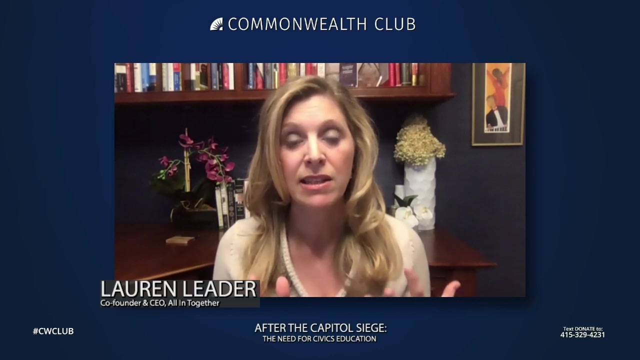 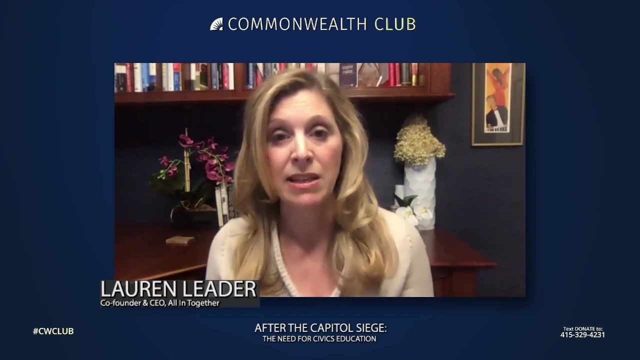 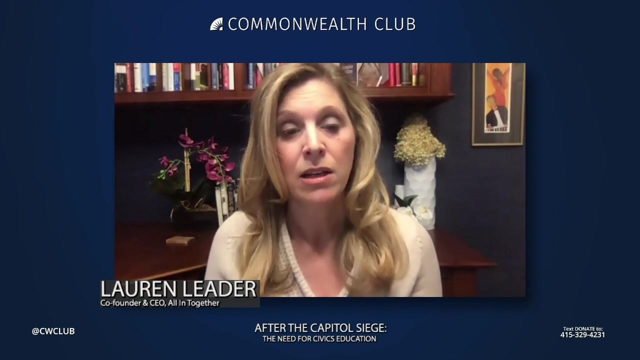 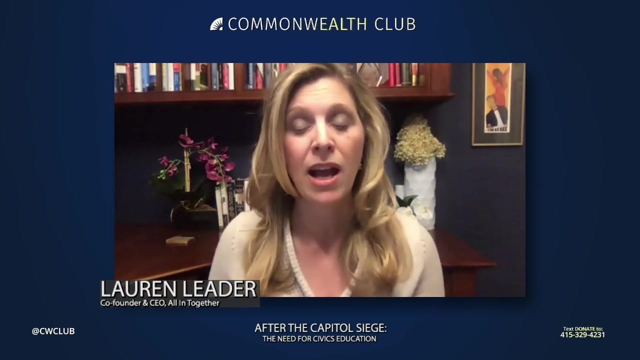 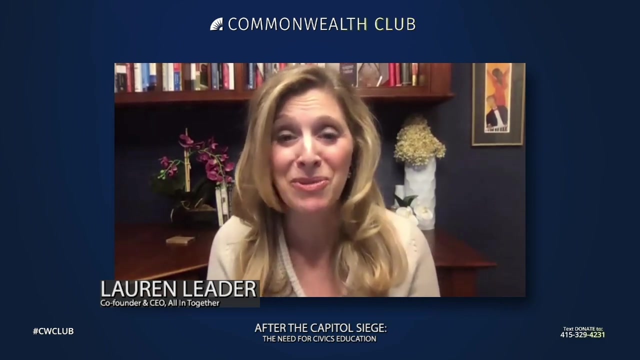 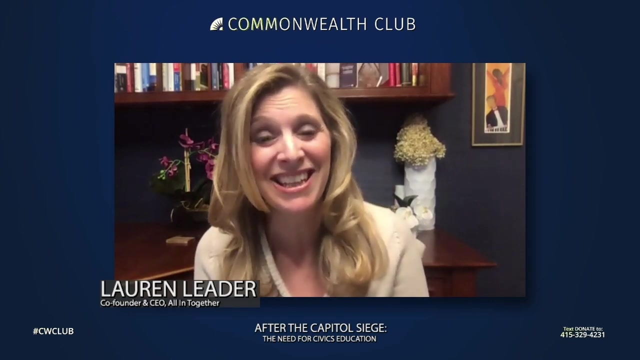 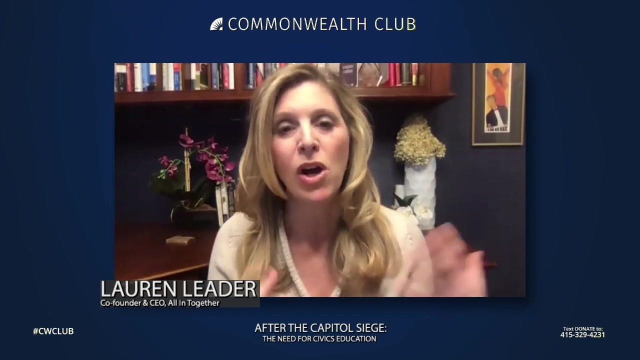 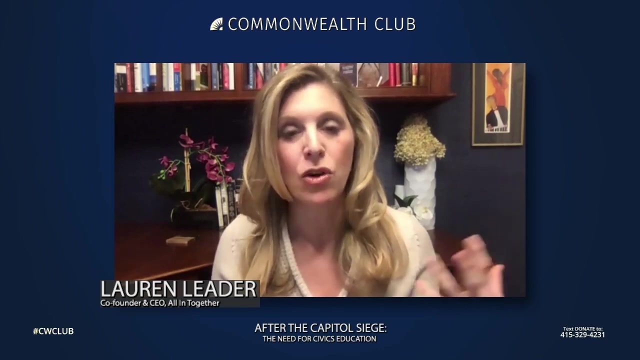 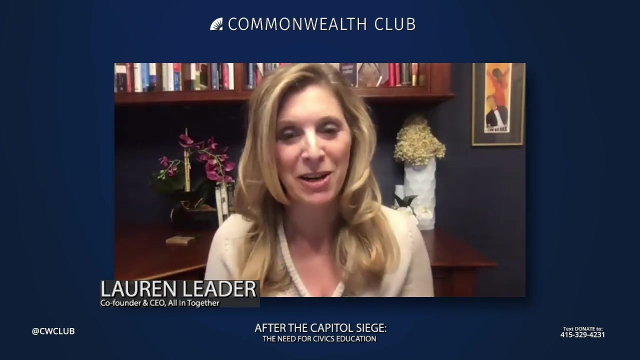 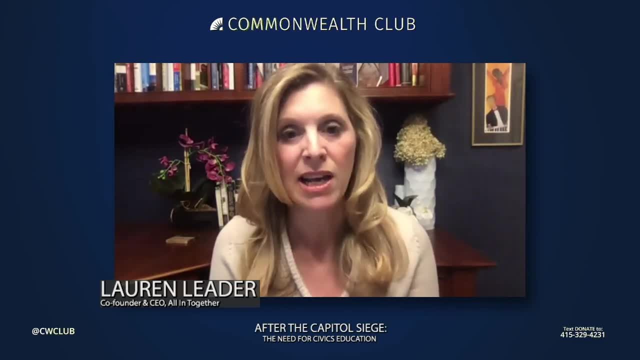 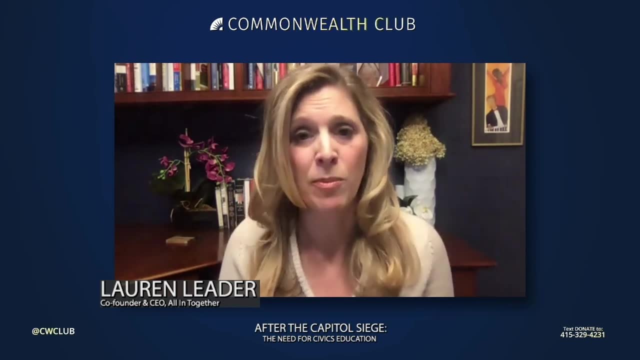 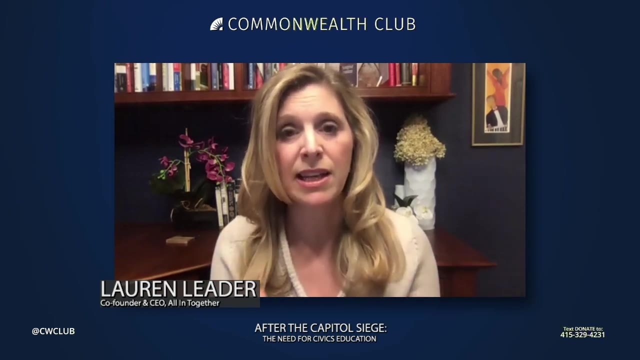 is that we partner with direct service organizations all over the country, everything from homeless shelters to domestic violence shelters to organizations helping to get employment for the formerly incarcerated. I think the organizations that are trusted support service institutions in every community across America, whether that's the YMCA or 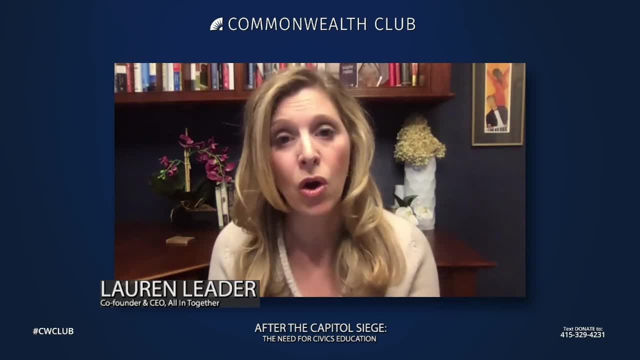 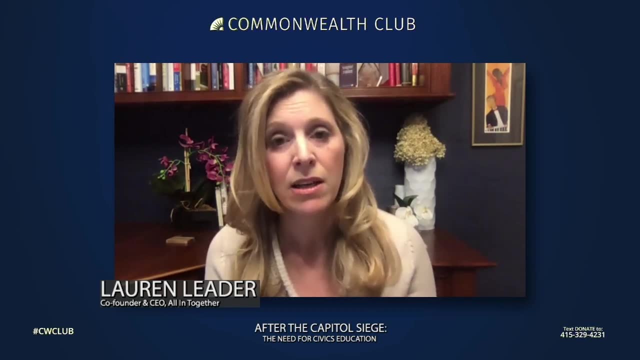 food banks. these are all places where we have an opportunity, if we can help them capacity build, to reach citizens that really have a right to have a voice and should have a voice, but may not understand how to have a voice. When we've done that, it's had really remarkable. 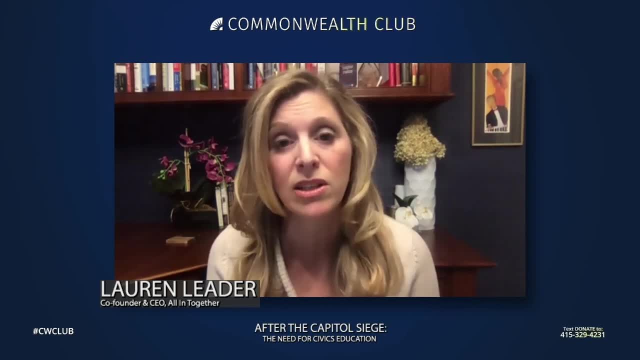 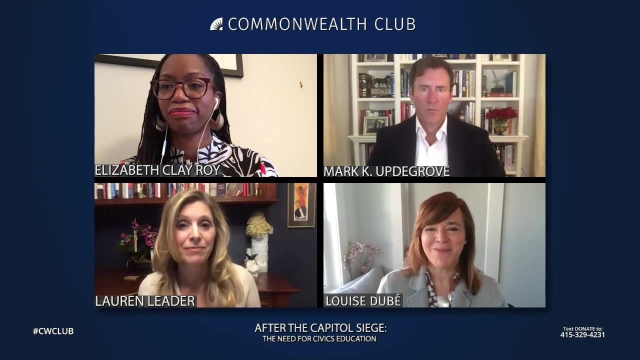 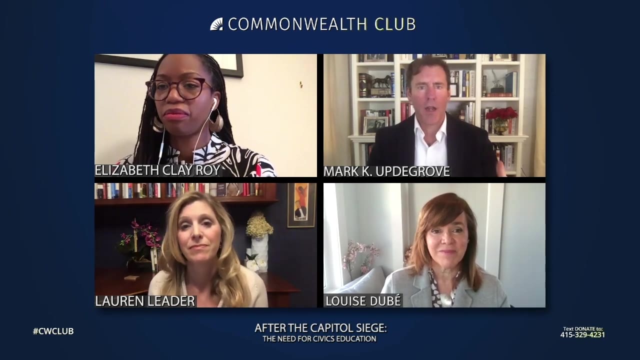 success. I think those local, trusted community organizations, grassroots organizations that are working across America all matter a lot. I'll jump in as well here, Elizabeth, if I may. I think again. Lauren and I have had lengthy conversations about the need for national service, bringing us all together. 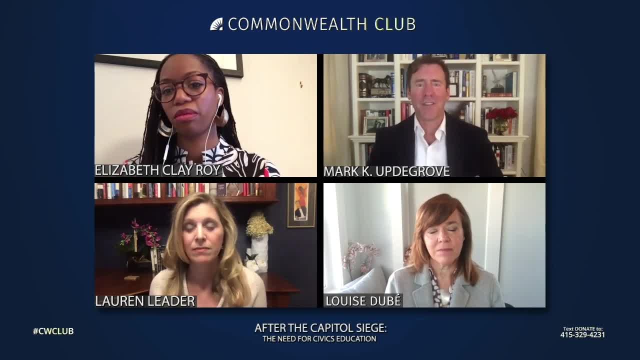 We talked about, for instance, during the orientation period, what we essentially the boot camp of that experience: teaching civics, giving people a better understanding of our system of government, but also allowing them to meet people who aren't like themselves. 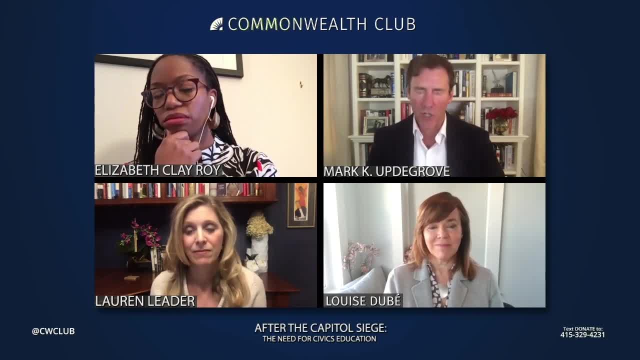 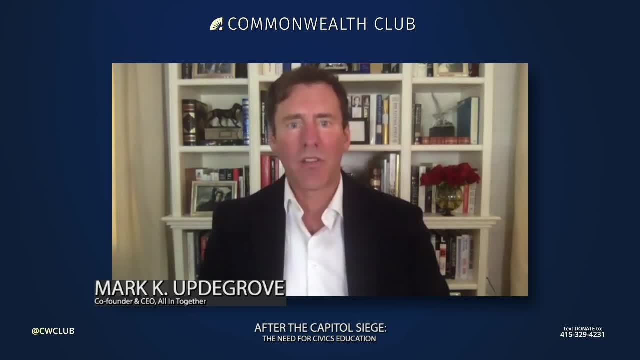 knowing that they're not the same people, Knowing that America is very different. Lauren and I, in our piece, quoted Lady Bird Johnson who, during the very tumultuous, very tempestuous 1960s, said: the clash of ideas is the sound. 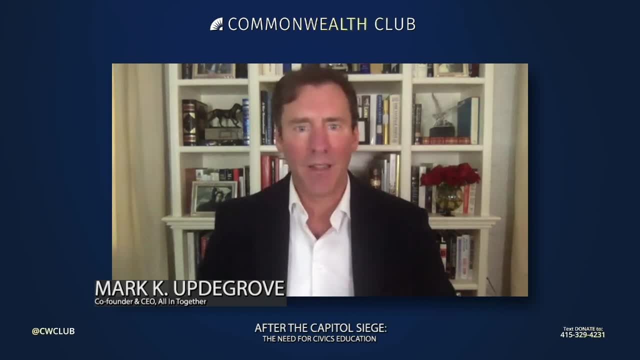 of liberty. Our very system allows for us to think very differently about different aspects of our government. That's a good thing. That's what makes us what we are. It's a bad thing when it results in violence. Our founding fathers were deeply concerned. 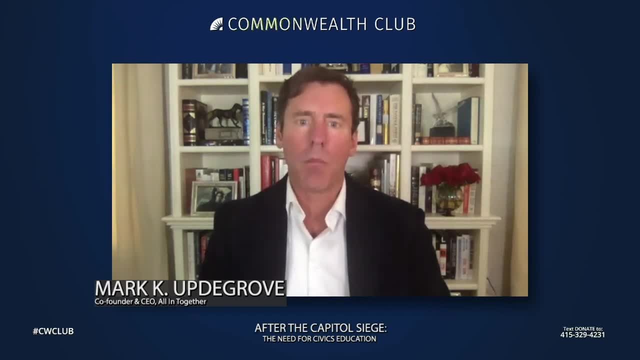 not only about an autocrat rising to power, but about the power of mobs. We saw both on January 6.. It was the worst of their fears And I think that it's important for young students not only to know about civics, which is essentially very important- ideas on parchment- but also about history. 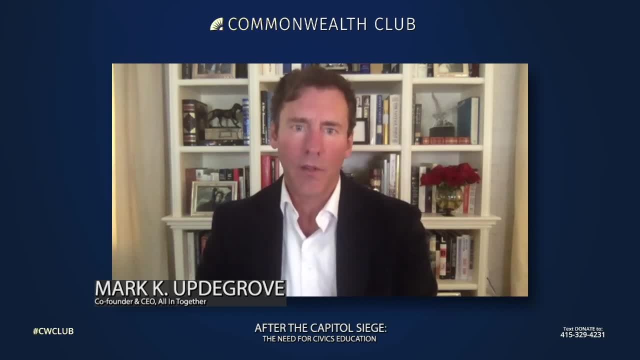 because history contextualizes civics. You can see it in practice And if you're a young student, like I was, you get caught up in these stories of these amazing people doing incredible things for this country and making the ideals of our country come to fruition in meaningful 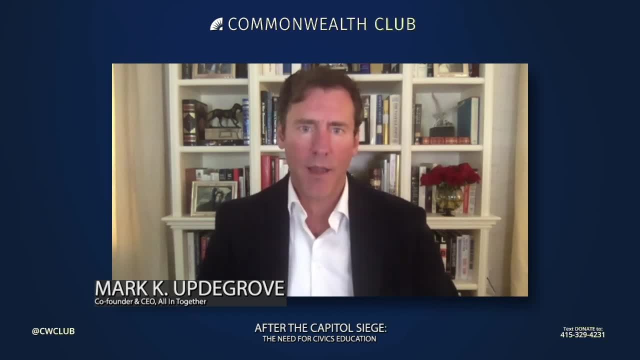 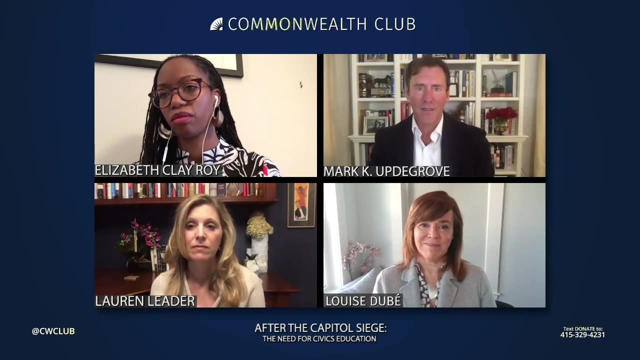 and important ways as we progress as a nation. So I would also suggest, too, going back to not Lady Bird Johnson, but Lyndon Johnson. Lyndon Johnson showed us in his presidency that you should let no good crisis go to waste- Every one of the civil rights bills that he passed. despite a very resistant Congress, was done in the wake of tragedy. He got John F Kennedy's Civil Rights Act passed due to the martyrdom of John F Kennedy, exploiting that as a means by which to get reluctant lawmakers to say yes to something that was extraordinarily controversial. 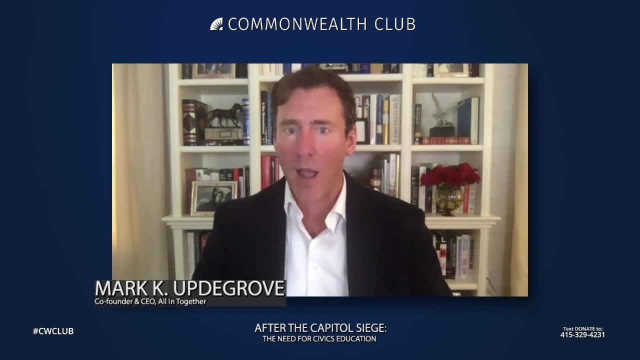 and, by virtue, broke the back of Jim Crow and its false promise. He got the Voting Rights Act passed less than a year after the Civil Rights Act was passed. because of the tragedy of the Edmund Pettus Bridge, what we now know as Bloody Sunday and the thwarted 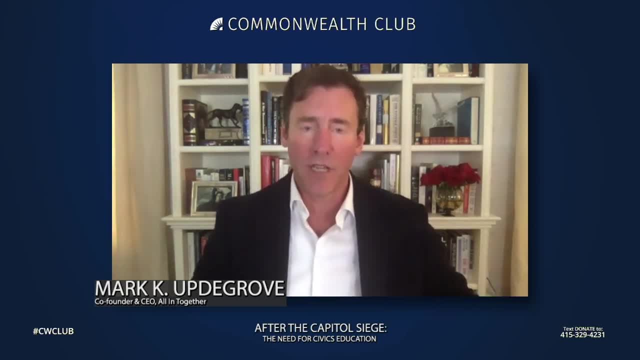 civil rights march from Selma, Alabama, to Montgomery, Alabama, in the name of voting rights thwarted brutally by Alabama state troopers. He exploited that opportunity to show the racial injustice And we got the Voting Rights Act passed in the wake of the 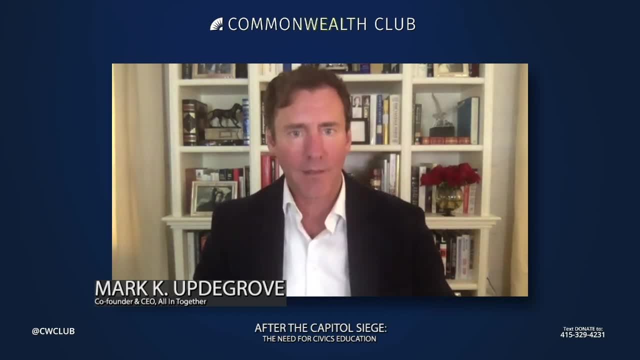 assassination of Martin Luther King. This is a crisis moment And I think President Biden has an opportunity to do something meaningfully, legislatively, to advance our society by looking at this as an example of where we've gone wrong. Wonderful point. 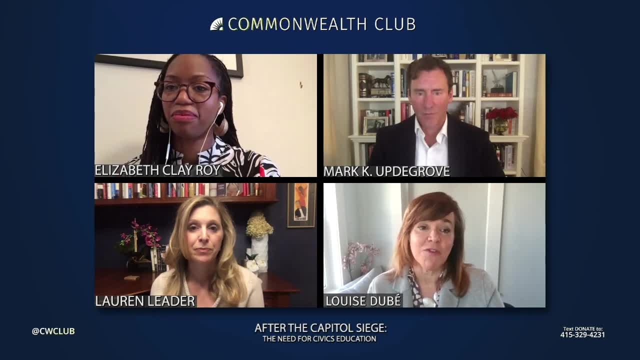 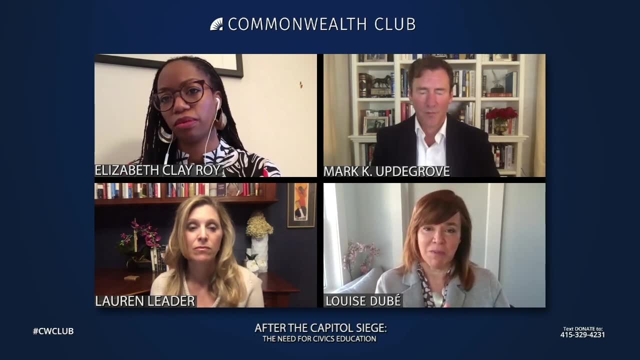 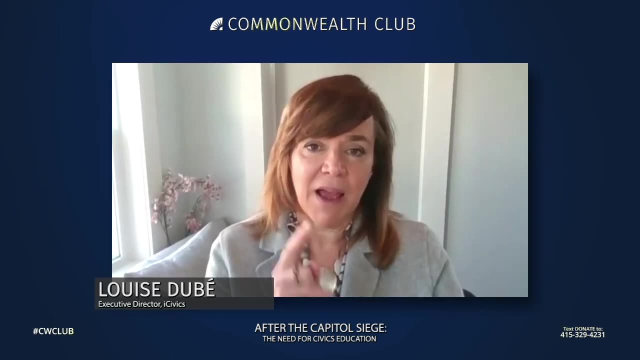 And I'll just first of all. I agree with you completely, Mark. History and civics are indivisible. We are just about to publish our report on the Educating for America Democracy Project, on which we've been working almost 18 months, about how to integrate those two disciplines. 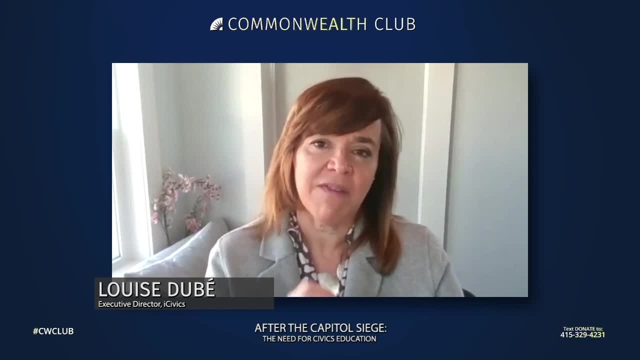 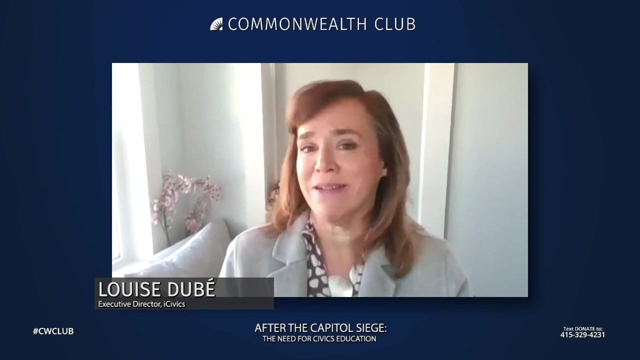 K through 12, in a very detailed way for civic agency National guidance about how to do that. So look for that on our launches March 2nd. But the answer to the question that Elizabeth asked from my point of view is really everyone. 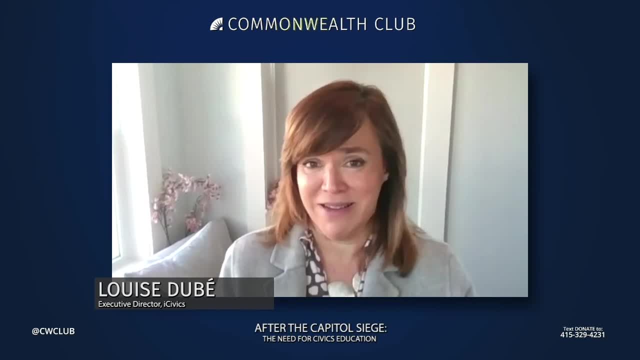 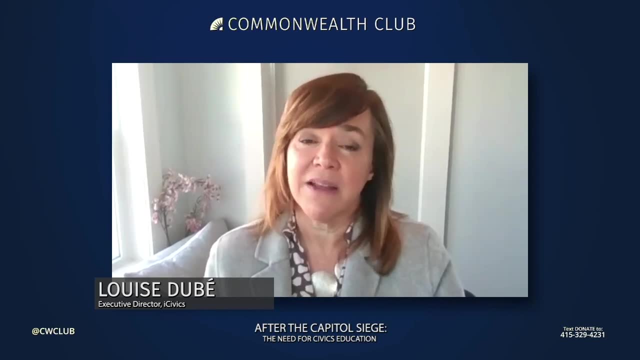 We need a movement. We need every single American in this country to say this must be prioritized. So we at Civics Now support a bill in Congress, bipartisan both in the House and the Senate, which provides for a substantial investment to states, for states to decide how to allocate. 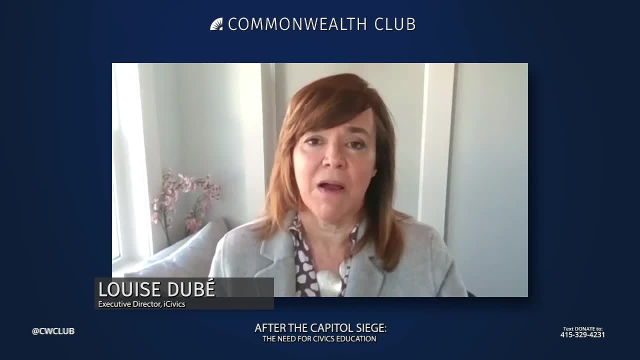 in history and civic education. That is a really important step and we support it wholeheartedly, and we certainly hope that the Biden administration will support it as well, but, most of all, that our legislators will see the crisis and use it for that purpose. 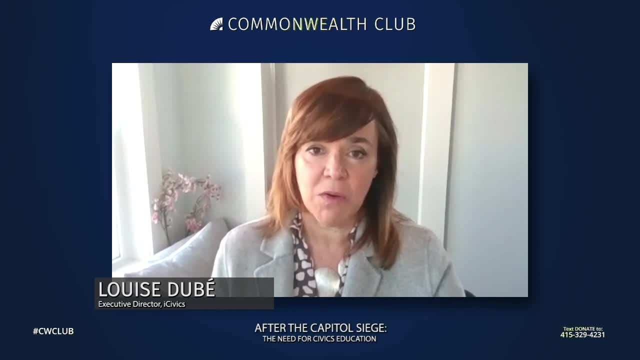 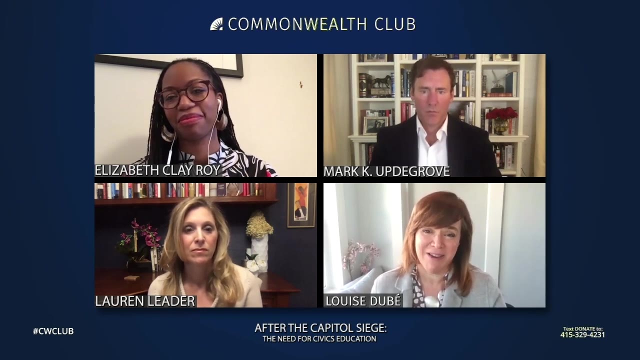 In addition to that, we have 20 state affiliate programs to change policy. So in 20 states we are moving forward. We're prioritizing civic education. But, to be frank, if parents went to their school districts and their school boards and demanded the 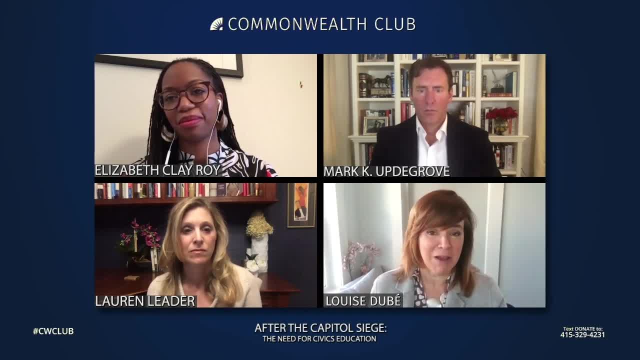 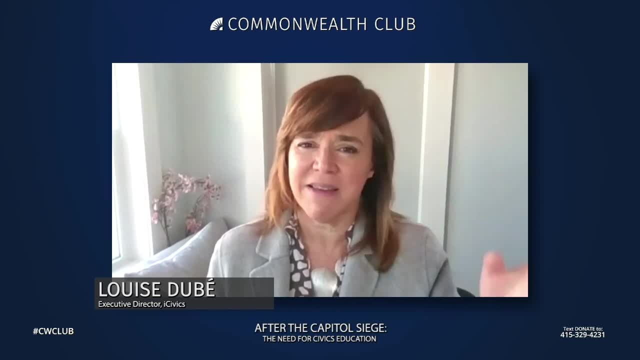 history and civic education, we wouldn't need policy- hardly at all. So I think that's really what I see is a shift in mentality about the importance of this, just to rebuild our civic strength. So that would be my answer: Young people, teachers, parents. 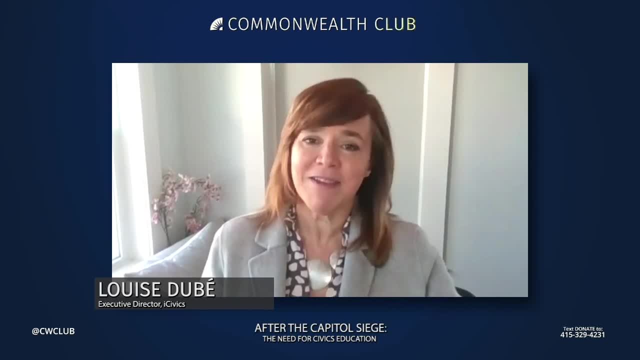 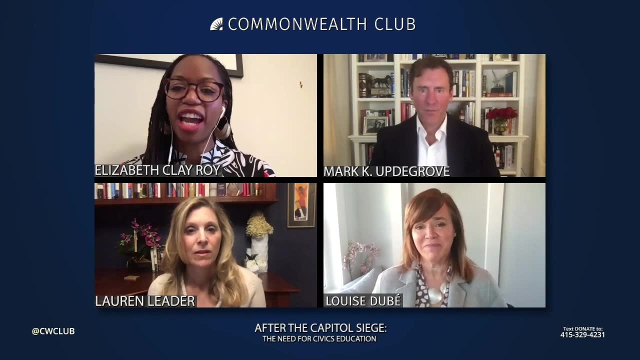 the corporate sector. We haven't seen as much investment in K-12, but I'm glad to see it's there and all together. Yeah, I completely agree about the need for a movement and voices from students and parents who are saying this is part of the education that they want. 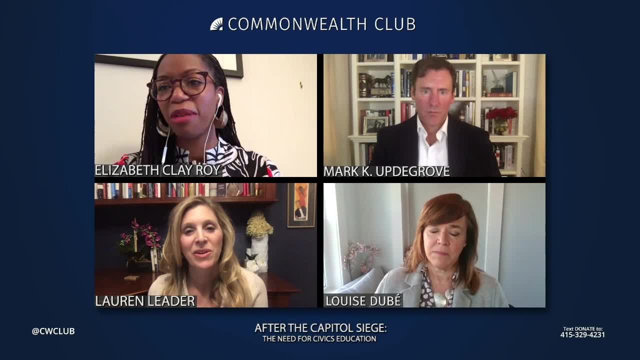 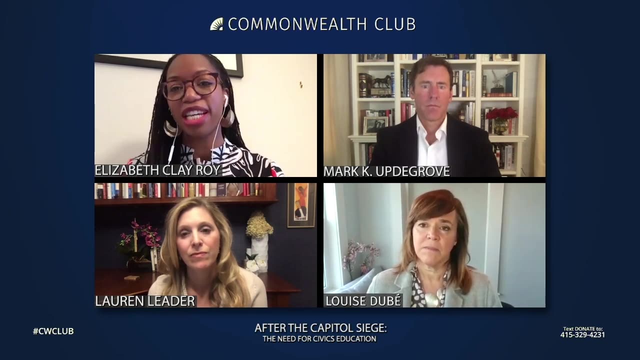 We've started to have some questions come in, and so I'm going to reflect some of those back out to you, But one of them is talking about how can we recenter the purpose of school so that it's about preparing citizens rather than workers. 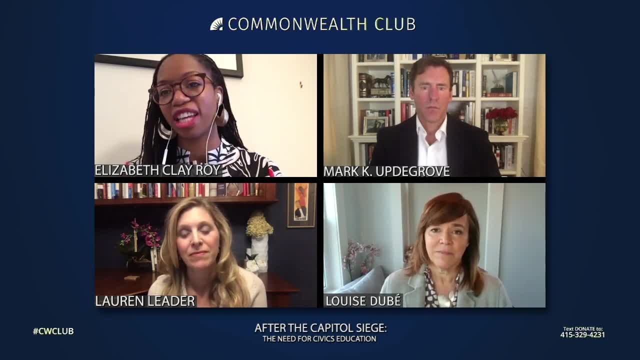 And that's an important question, and one I think, in terms of the answer Louise does come from the voice of students and parents about saying what they are looking for, But it brings us as well to another good question that's come in from YouTube. 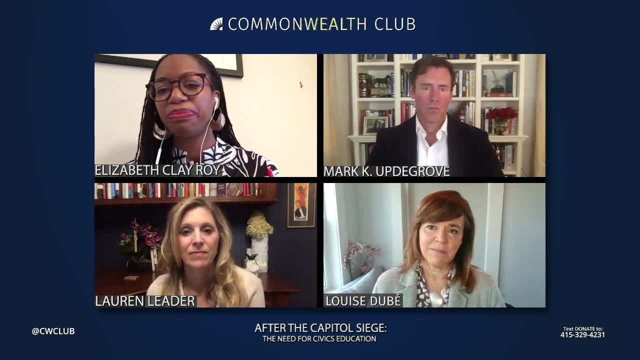 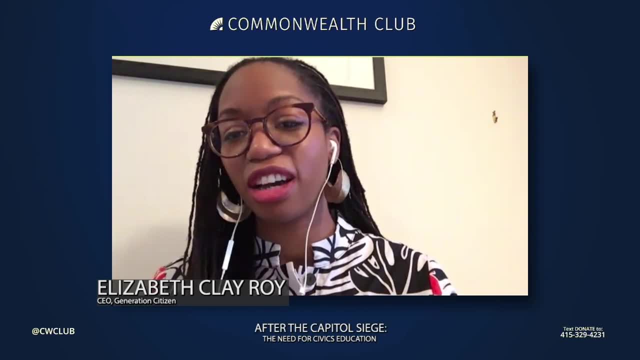 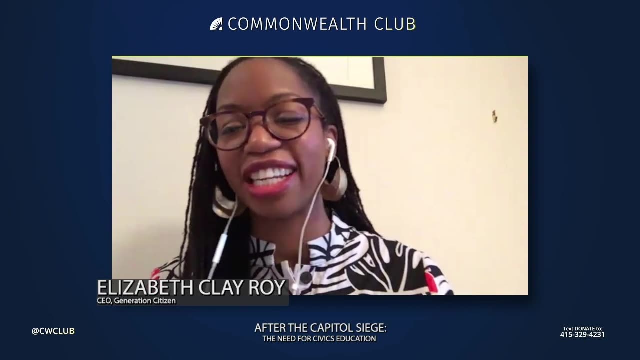 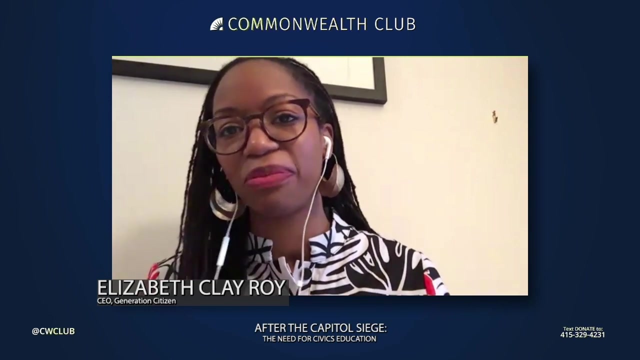 And I encourage others to keep adding your questions in. There is two questions that are connected: How do we communicate this universal idea within our decentralized education system? And then a question about what are the stumbling blocks for civics, ed And, and so recognizing the complexity- appropriate complexity- of our education system. 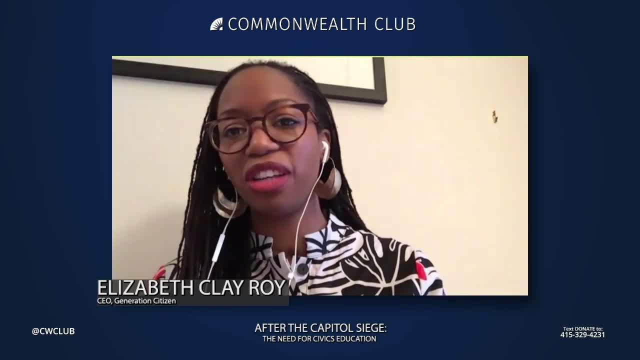 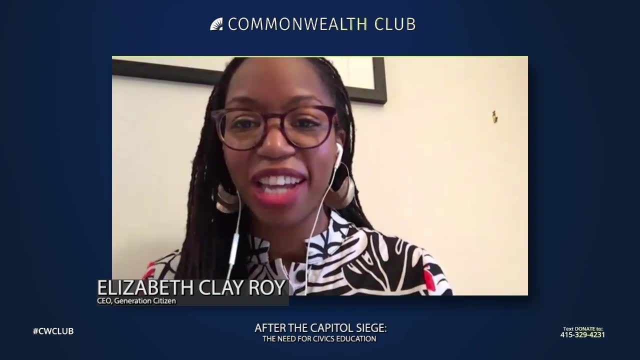 How is that an impediment potentially to civic performance? Yes, Yeah, I mean, I think that that's important. Okay, education in the way that we're talking about it today, And how do you move through that? Anyone want to pick up on that? The expert on this and I want her to answer it, but I wonder if I could. 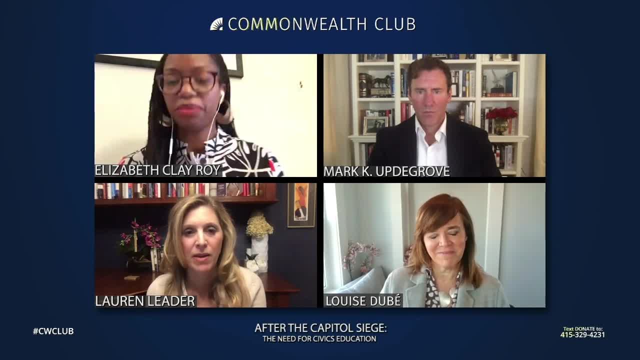 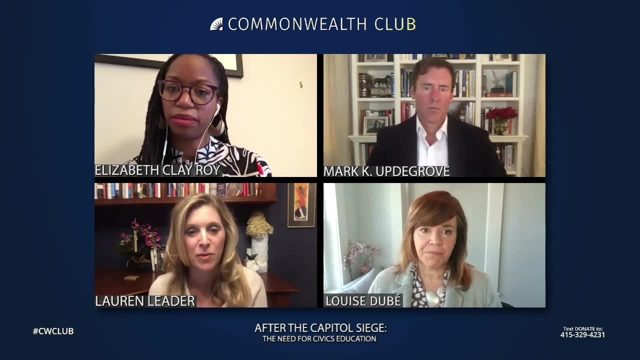 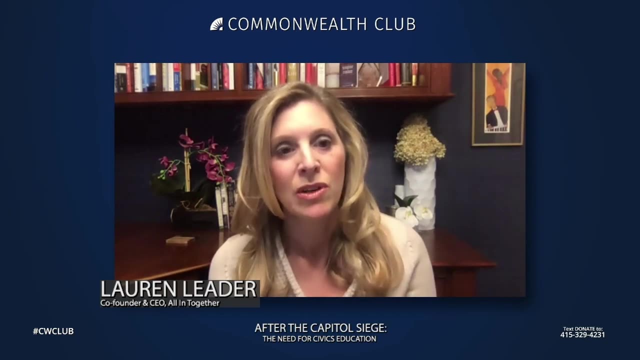 just make one quick point from the last point about this. You know one thing that I am concerned about and I think- and I really this was something I really learned from the LBJ library and particularly from Bill Moyers: the history can't be whitewashed. So history and civics are. 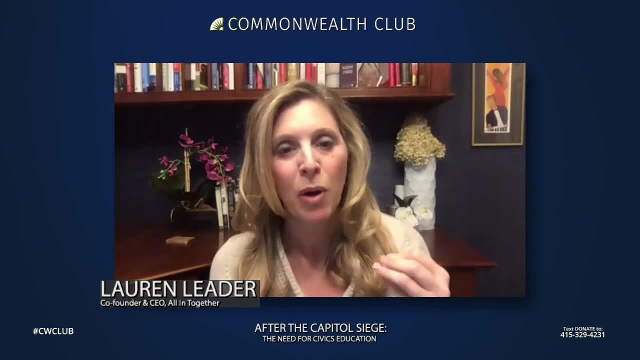 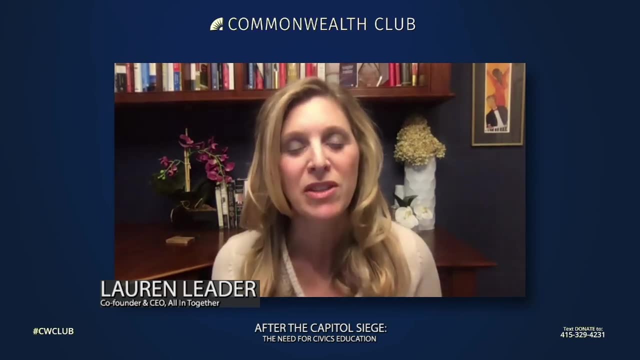 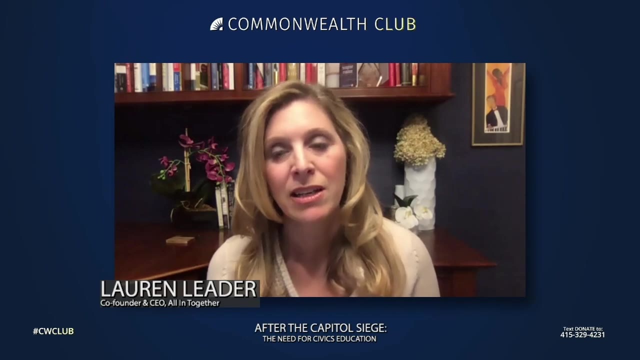 inter are inseparable. But part of what has also happened is that the history, part of the civics education in the last, from particularly the last 50, to even back to the Civil War, to your point- has been whitewashed And that whitewashing, I think, is also part of what the racial you know. 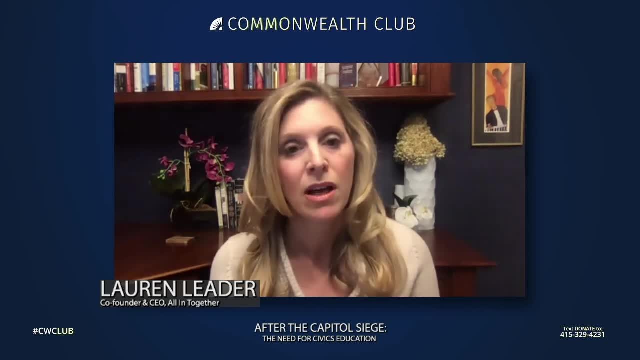 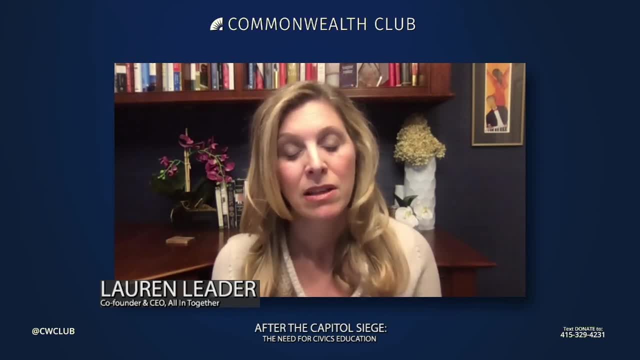 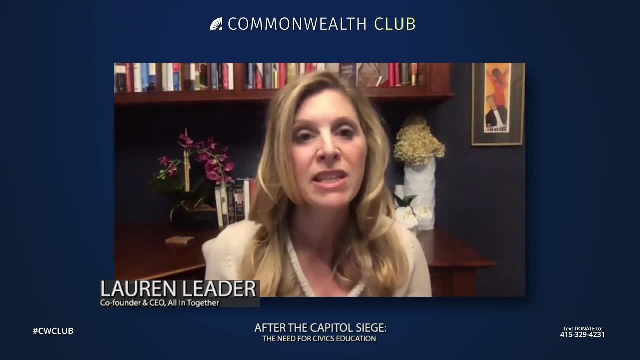 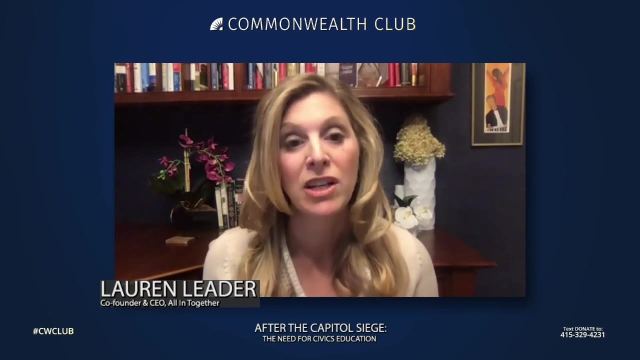 and he had a 60% unfavorable rate. you know, approval rating and all of these things that, like we think about the civil rights movement now in a very sanitized way And that has the implications of that, you know, enables white supremacy to continue to rise, because we just 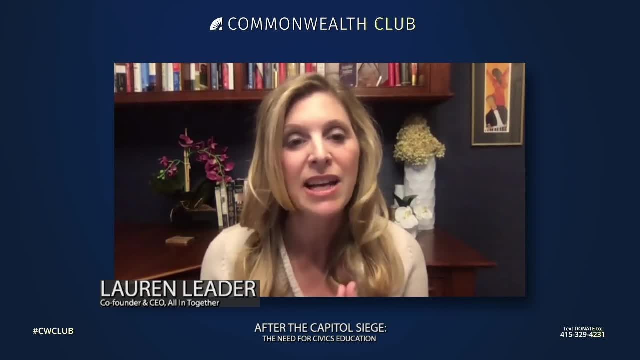 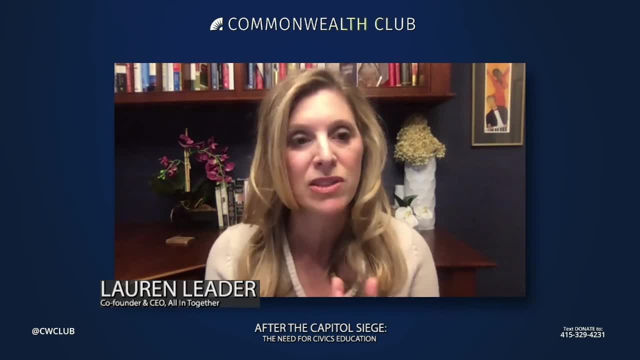 to the like, just inseparability, and, Louise, you just said it so perfectly about the just inextrability of civics and history- That history has to be honest And what's been happening is that education- and I'm not an expert on that, Louise, you'll speak to it, but in the states, 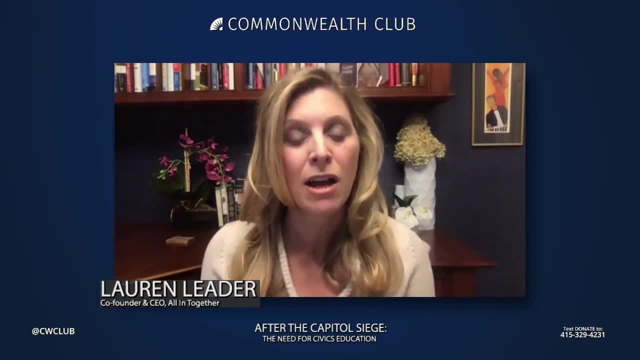 you know- and this is back to civic participation- you know state governments determine a lot of the curriculum that gets taught across the country and that has become extremely politicized And Americans have not been paying attention to what's been going on in their state houses. 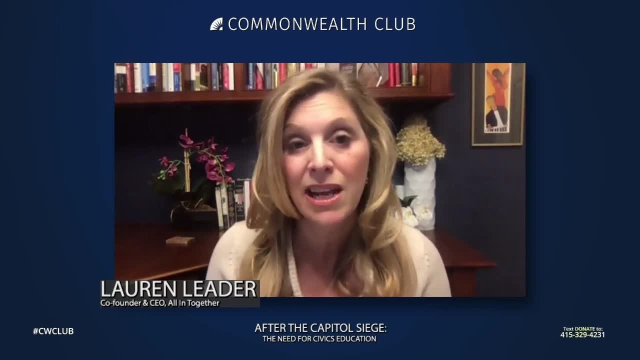 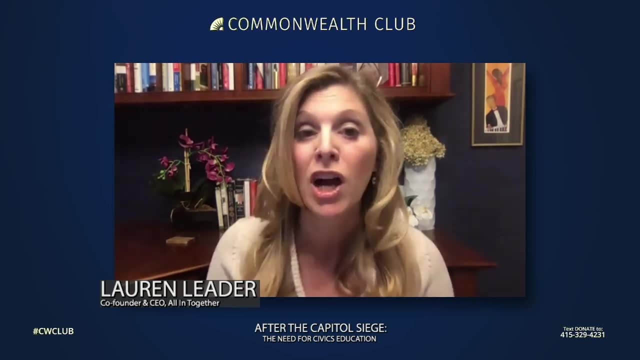 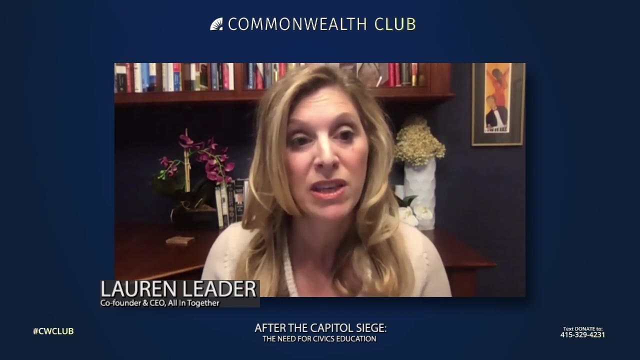 They have been really not engaging in state races, not paying attention to who's getting elected to those races and winding up with sometimes some very shocking outcomes for people who are committed to- you know, certainly- progressive values and to some of these issues. 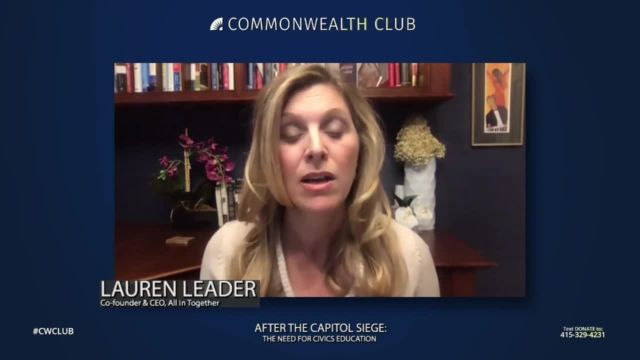 So you know, you've seen this in many states where the part of why education has failed around civics and is failing to teach true and honest history about the you know the you know our race's past and about you know the real who we really are as a country is partially just. 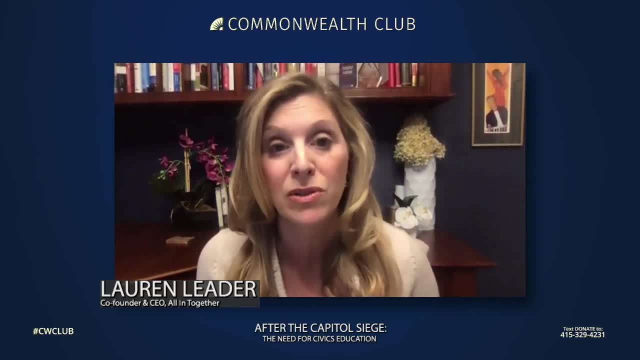 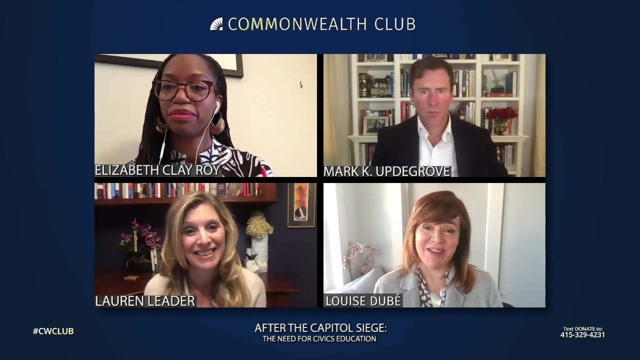 the lack of attention to the importance of those state houses and local school boards, et cetera, all that local state political structure that determines what our kids are learning. Louise, I'm sure you have more to say about that. Yeah, I completely agree. So I love the quote. 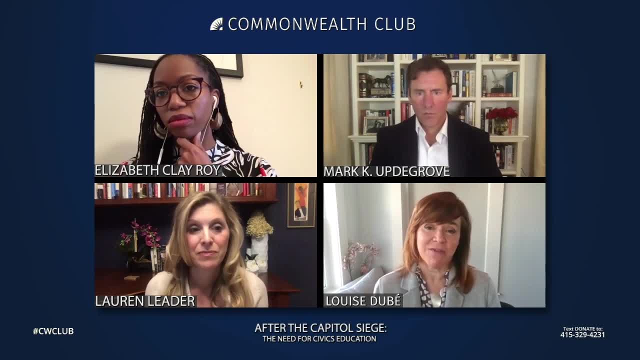 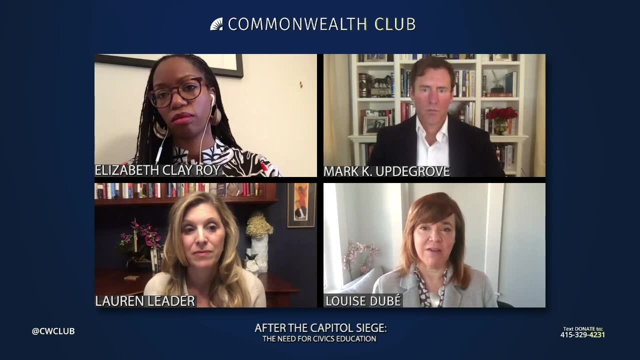 that Mark said from Harry Truman about the history you don't know, because, frankly, we need to dig a little- not a little- a lot deeper to tell the histories of marginalized people and histories that are not known, that are just as actual, factual as the history that 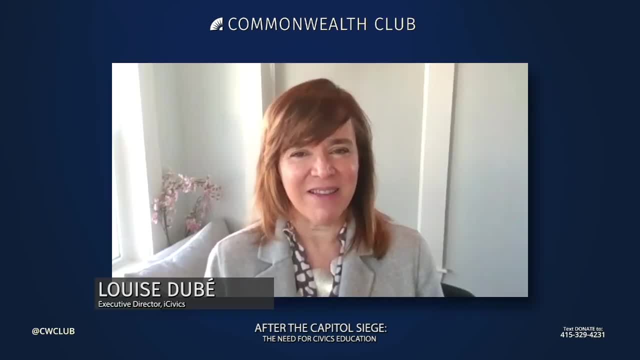 we do know. So there is a sense that things just happened, but the actual history is much more complex, much more in-depth, and that's what our project really is about is to be able to unearth all those stories and to be able to tell the stories of marginalized people and to be able to 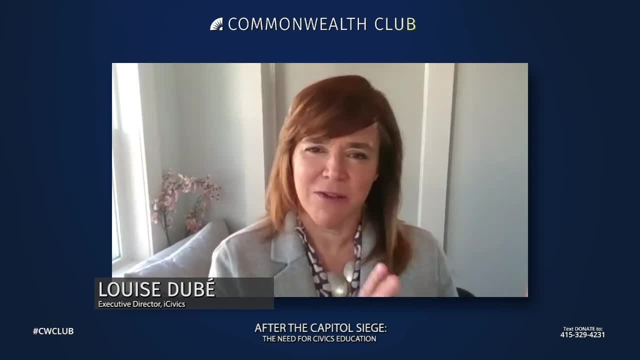 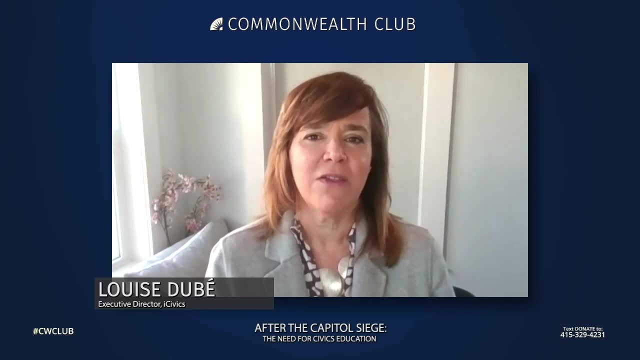 tell the stories for all students, right? It's not. there's not one segment or a problem for one type of students, a problem for all types of students that we just haven't given them the skills, the knowledge, the capacities that are needed in this today's democracy, which is very 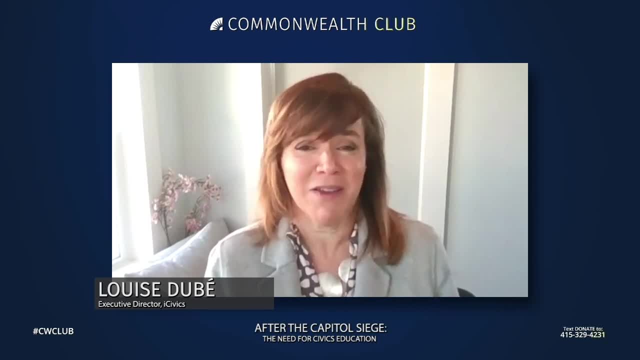 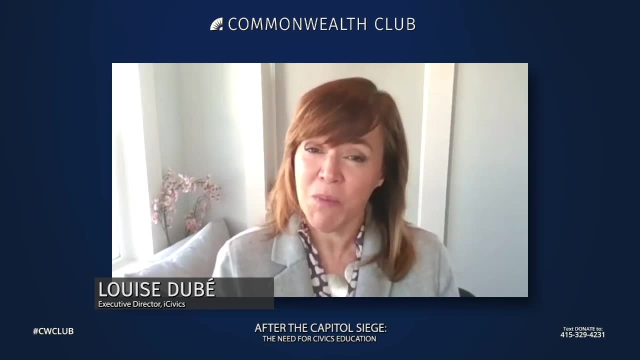 diverse, very complex and lots of people don't know about the Tulsa Massacre. They just we need to tell stories and we need to tell them in a way that leaves young people hope but also understand that our country is built on very, very painful episodes and, to this day, our history. 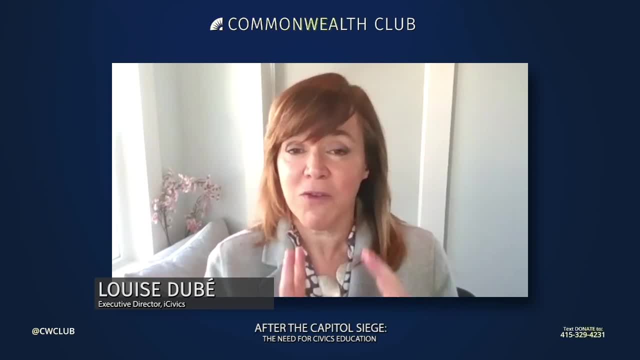 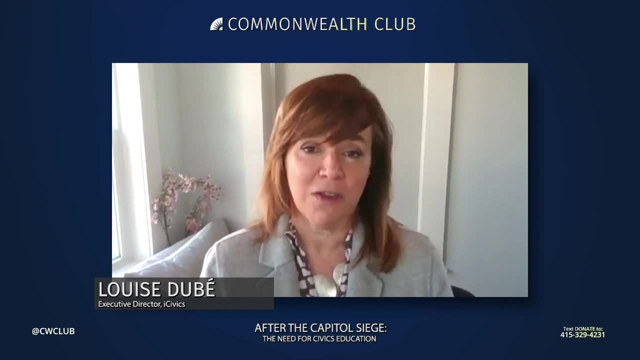 is very painful, So I will just address two things. One is, as my colleagues Danielle Allen and Paul Carice noticed, the mission of the US Department of Education does not include generating graduating students who are civically prepared and engaged, and that needs to change. And also, if you look at the district, 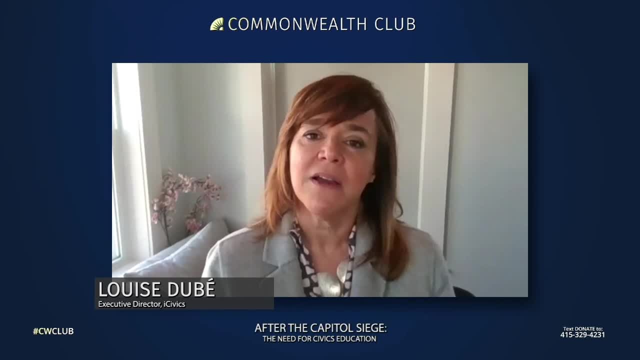 missions, as one of our other colleagues, Robert Pondicio, did. that's a problem, right? We need to make sure some of these missions talk about global citizenship. How about also citizenship in our country? So that would be important. So that's one You know I've been in education for. 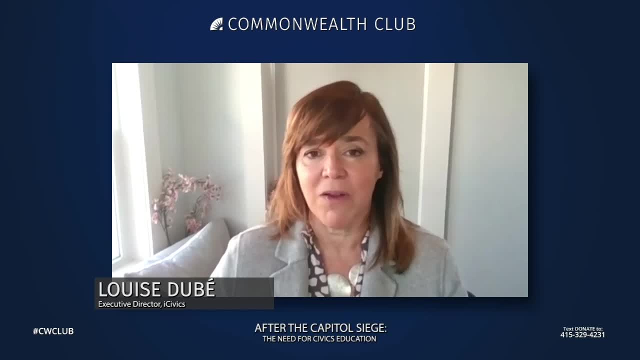 a very long time, and I think the person who sent in the question is absolutely right. This is a complex system that is hard to change, and what we've learned is that it cannot be a top-down measure, right, So we've had a lot. 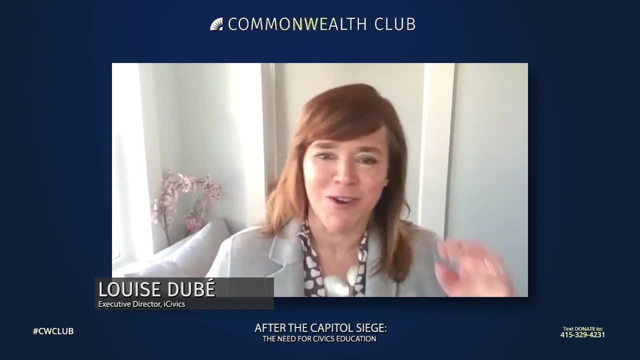 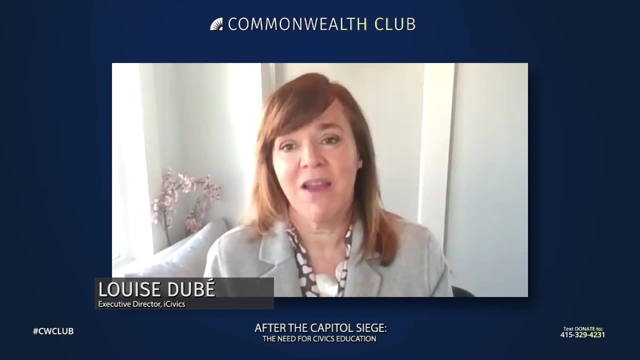 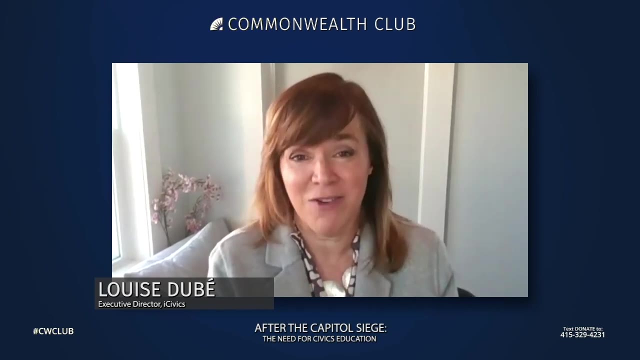 of top-down, top-down, whatever top you want to talk about- federal, state, local, whatever it is. We need to have a very systemic approach to this. We need to have parents demand it. You need to have young people speak up as to what they want and they do. We need to have educators involved. 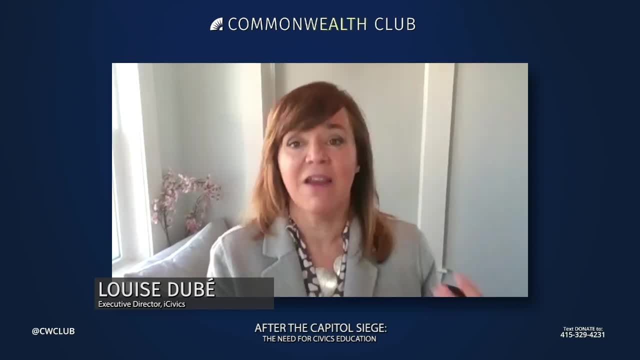 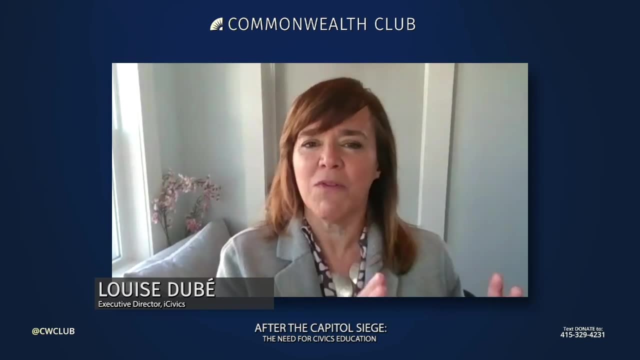 at the table And again, we've had that not only from day one, but we also need institutionalized structures because it's not a short-term problem. A lot of the issues around civic education in K-12 is that people feel like this is a very long-term investment and it is right, But the urgency 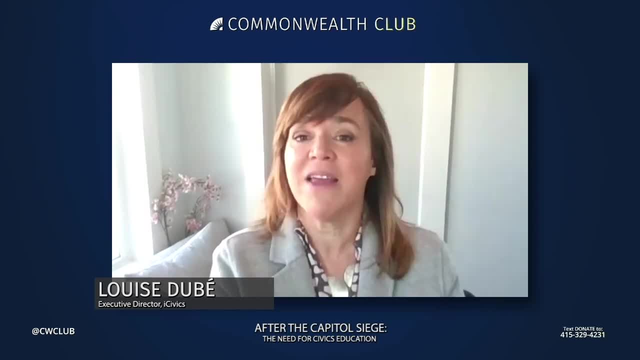 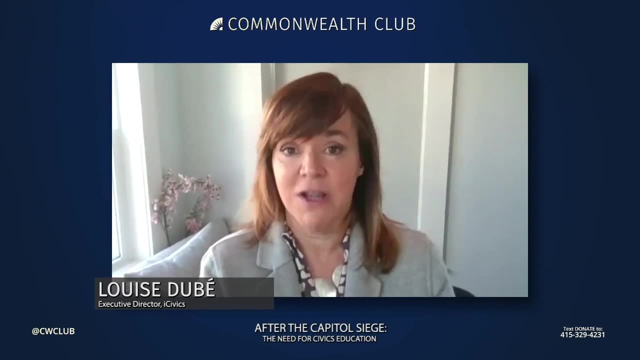 we feel now needs to make sure that it results in some structures that will live for decades and even beyond that, forever, And so we need those institutionalized structures to be able to institutionalize that. So we need to have a very systemic approach to this, and we need to 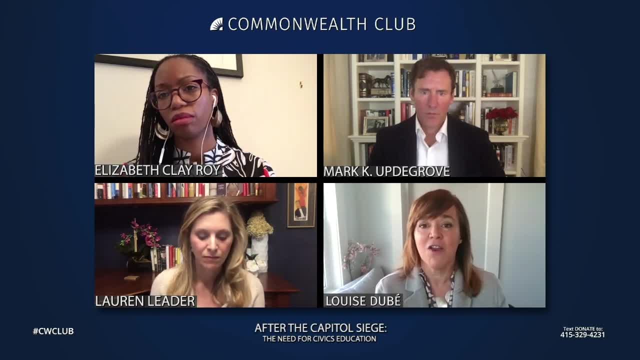 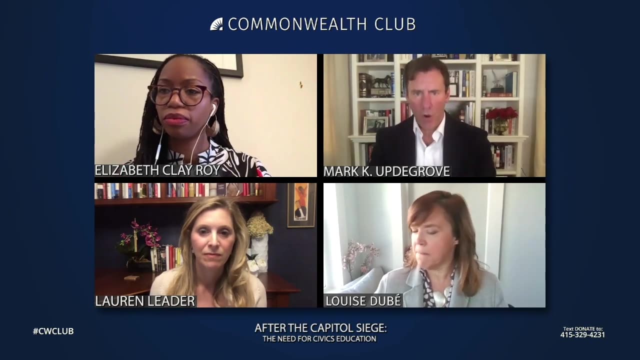 institutional homes for that kind of change. So if we were able to do that- and that is what we're working on- I think we would be a better country for it, And so I'll just stop there. Elizabeth, can I just add one thing to what Lauren said earlier? She mentioned Bill Moyers. 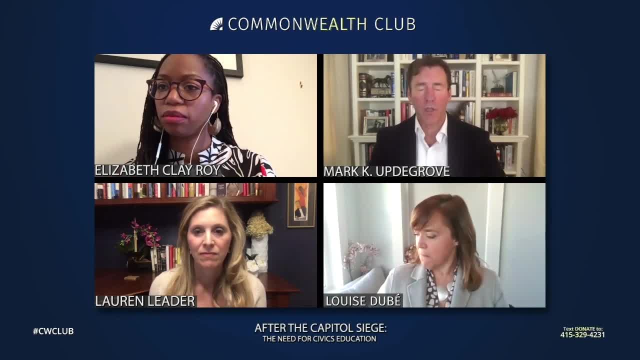 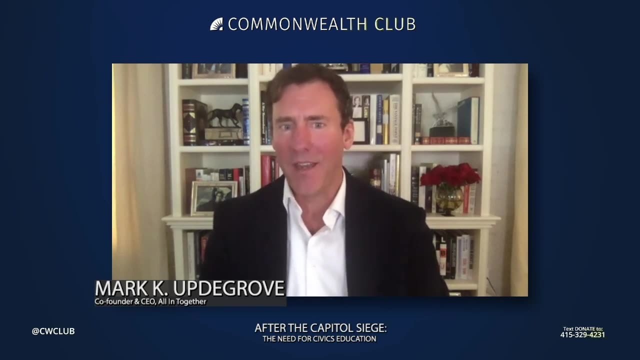 warning about the whitewashing of history. Bill Moyers was the press secretary to Lyndon Johnson during several years of President Johnson's White House term. But there's an old axiom that says it's easier to build a monument than it is a movement, which is to say it's easy to 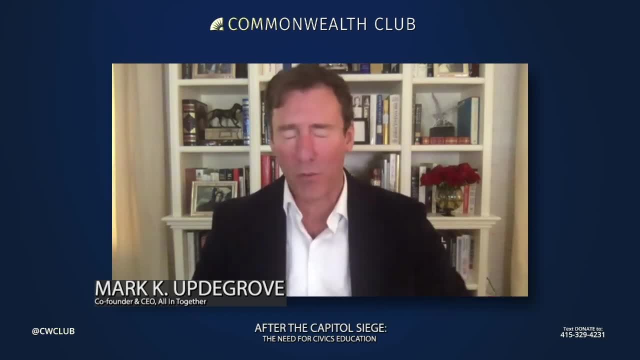 look back at Martin Luther King. I'm looking and I'm in my study and I'm looking at a wonderful black and white photograph of Martin Luther King there. It's easy to look back and make a holiday for Martin Luther King, But we cannot forget about how fierce 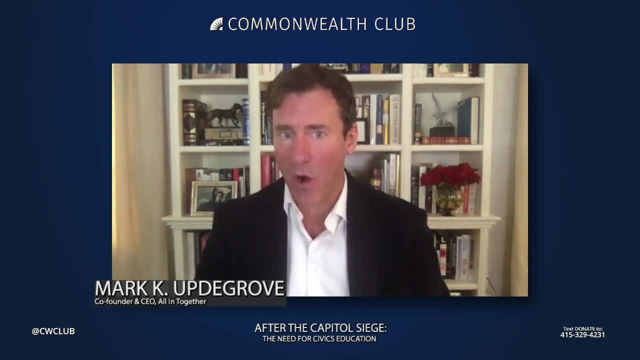 it is to build a monument for Martin Luther King, And I think that's one of the things that we need to look at: How defiant, how iconoclastic Martin Luther King was. As Lauren said, I think he had a disapproval rating in the United States of almost 70%. He was considered a rabble rouser. 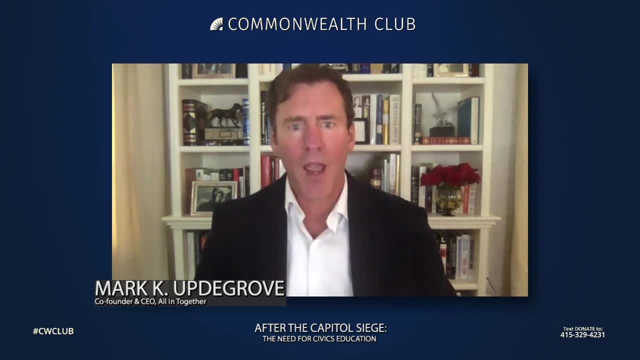 somebody who was stirring up trouble And in fact what he was trying to do, as we heard in his iconic I have a dream speech- is to get us to reach beyond ourselves to actually live up to our ideals. But we need young people to see. 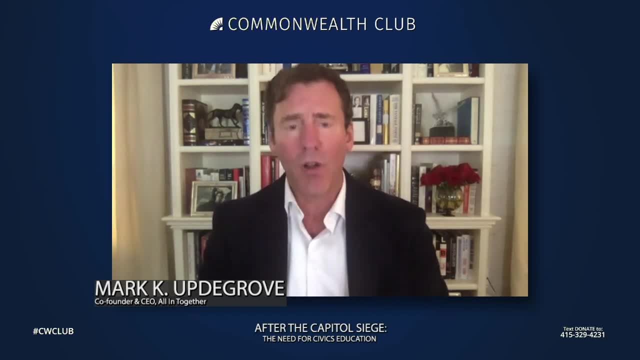 the struggle that he had and the real, non-whitewashed story of Martin Luther King, so that we can equate it to what people are saying about Black Lives Matter now. Oh, they're just stirring up trouble. They're rabble rousers, right, They're just getting in the way. 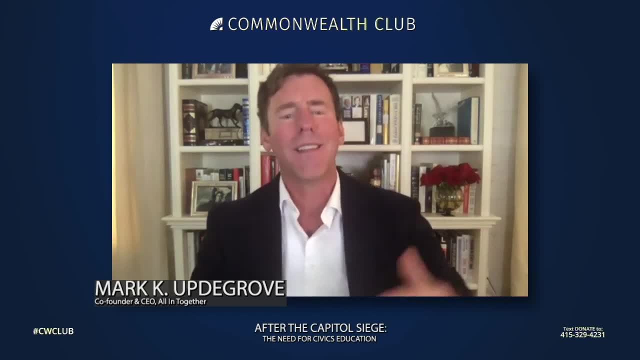 They've already gotten so much and they want so much more. That's exactly what they were saying to Martin Luther King 50 years ago, And now we have a national holiday in his honor, So it's vitally important. I think, too young people can relate to history if it's told in a 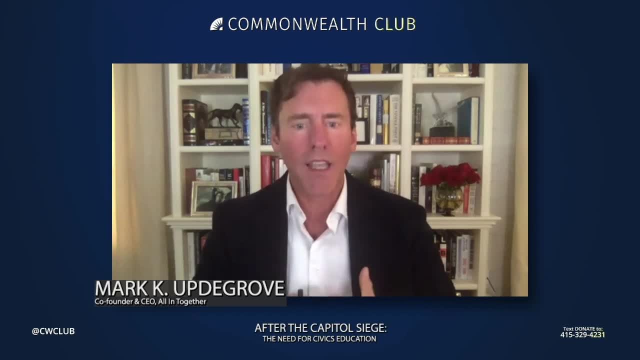 truthful, credible, realistic way. That's what gets you involved. You can relate to these people and the struggles that they have, So I could not agree more with that notion of not only teaching history, but teaching it in a way that is realistic and that reflects the struggles that we have had. 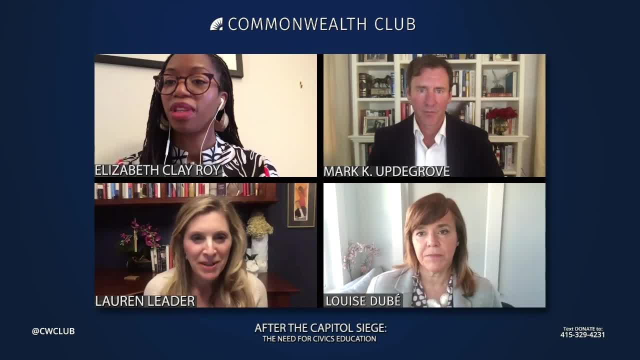 during the war, And I think that's what gets you involved, And I think that's what gets you involved During the course of our years as a nation. Amanda Gorman, twice in the poem, references Hamilton And my 11-year-old who literally 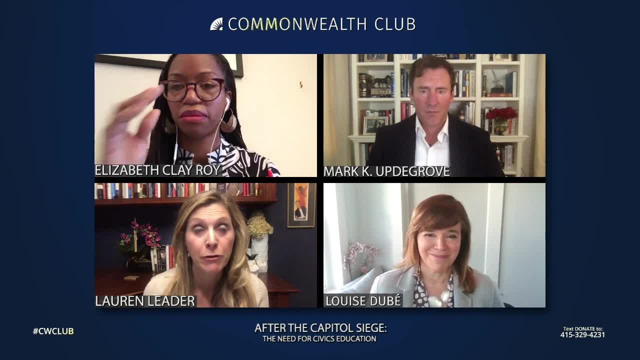 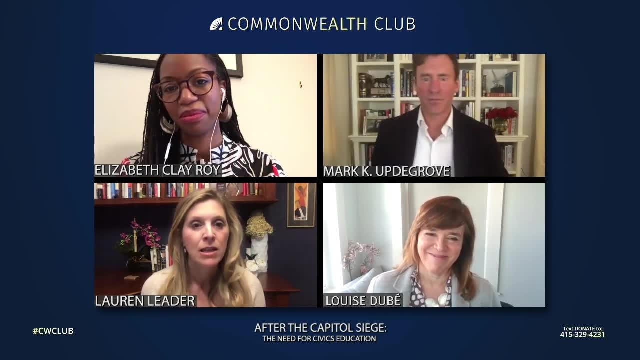 has been listening to it on permanent loop for four straight years. I wish I was exaggerating. It's every day, all day. for four years. my kid has Hamilton playing In one second. she heard that was what stood out to her when Amanda Gorman spoke. She's like: oh, that's Hamilton History. 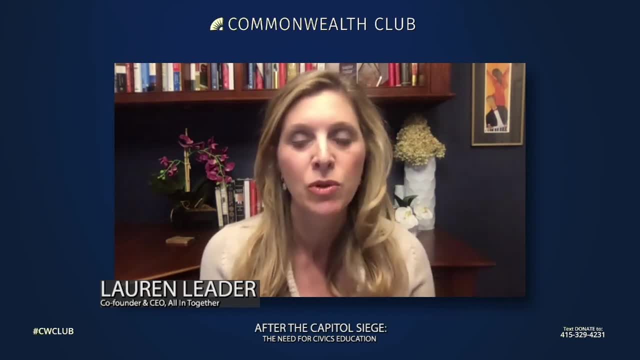 has his eyes on us. And then she yesterday was reciting George Washington's speech in his departure when he first- which is part of that wonderful song- In Hamilton George Washington's going home. She knows every line and she knows his entire speech And she's 11 because of it. And Amanda Gorman uses a small piece of it. 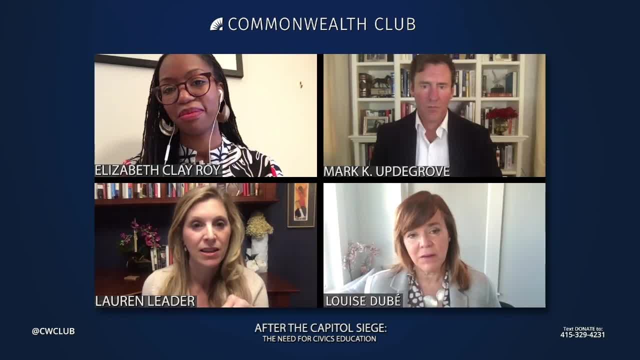 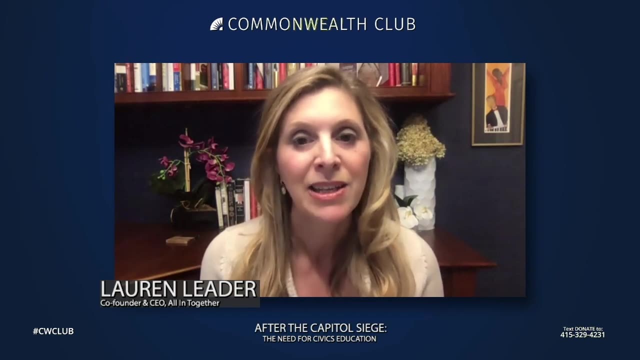 in the poem. There are ways that we can reach people in these very deeply personal ways. There are ways where it the root of this extraordinary ideal, of what it means to be American, connects. And you know Hamilton for all, you know, whatever criticism you can lodge, 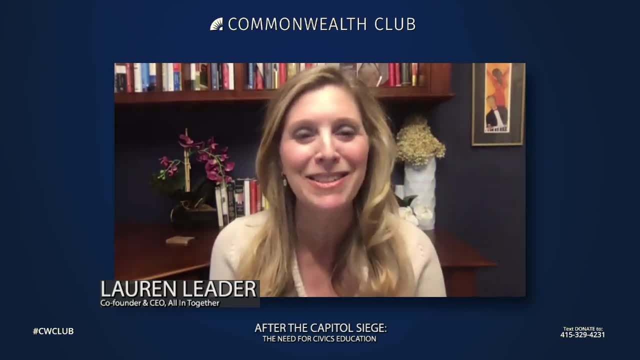 about. it's not exactly perfectly historical at all places, but it is so. it is such a perfect example of because none of us mentioned art And so, as Mark was speaking, I had to say that, just because it's literally 24 hours a day in my house for years. So I think that like that, I hope we'd 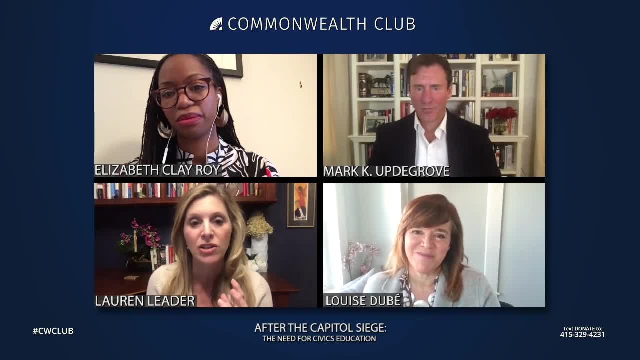 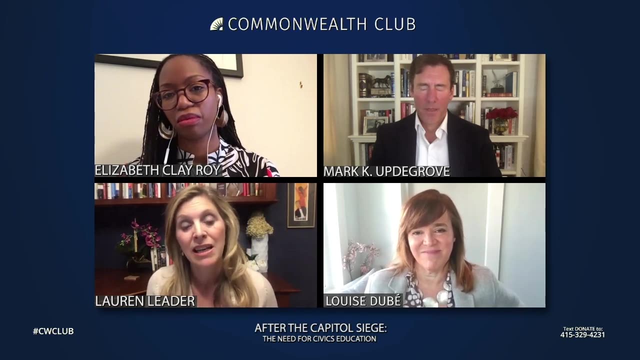 see more of that, Of that kind of willingness to also bring art and culture to that. this piece of it- And I hope that's actually something I think many of us are hopeful will come back to the White House in this new administration- is the power of art and music and to help people connect to our ideals. 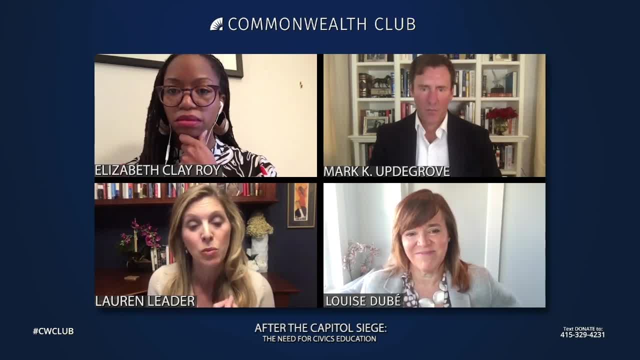 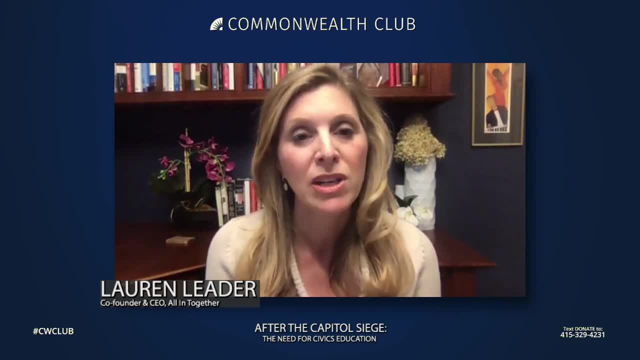 And you so beautifully. Elizabeth started by talking about Amanda Gorman, And I think that is why she struck such an extraordinary chord. Is that the beauty, The beauty of the way poetry and art can elevate our national ideals, is something that speaks to. 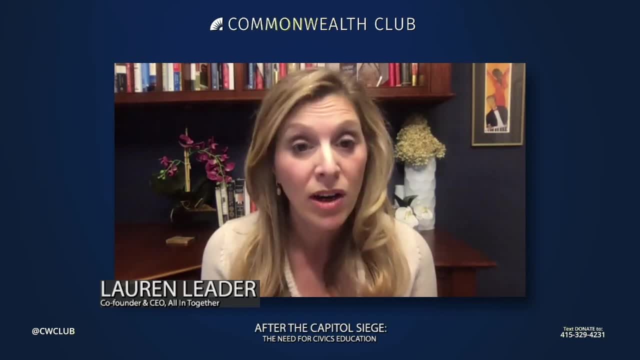 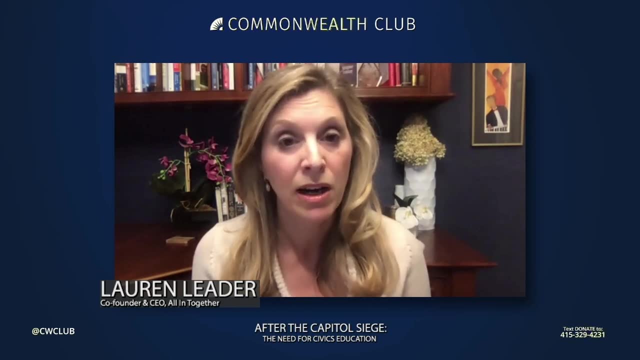 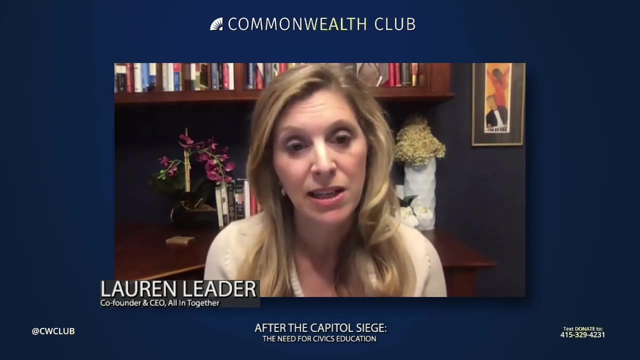 people across so many lines And you know we need more of that and we need to bring more people into that. And you know I've worried very much about suffering Americans in this particular moment, who you know are. so I mean we haven't even touched on how totally disconnected now 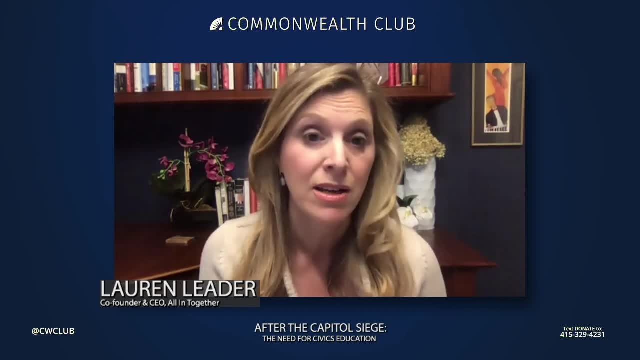 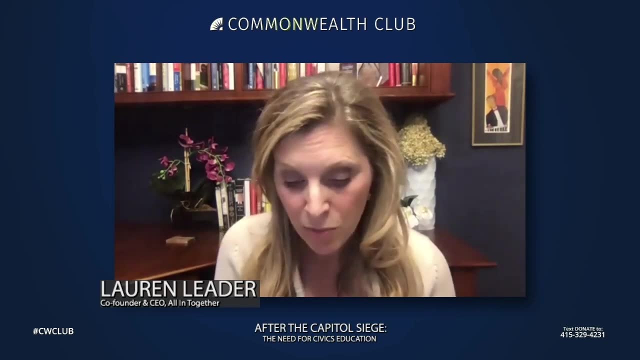 so many millions of kids are from the core Of what is even their academic experience, because they're at home and not in school and all of that. We all know that's the background. but I loved Mark's point about not wasting a crisis And I 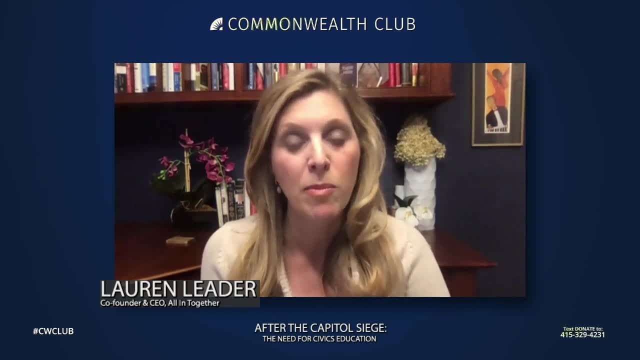 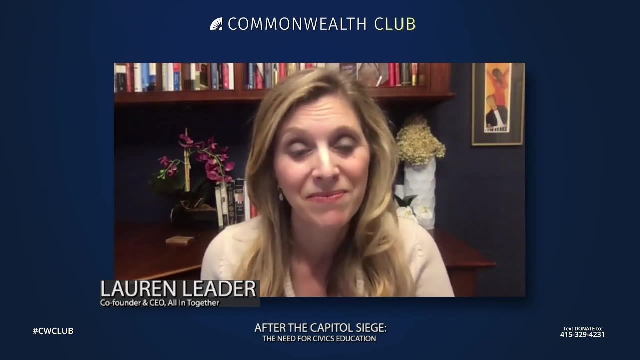 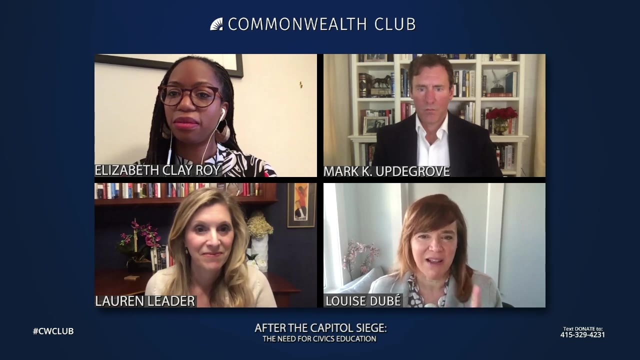 think that's exactly what this moment is, is this incredible opportunity to just refresh and renew and rebuild the best of what we are. Let me just, I'll just add- I love this And I think it would be great to you know unshackle civics from civics class. It belongs everywhere. I think our students 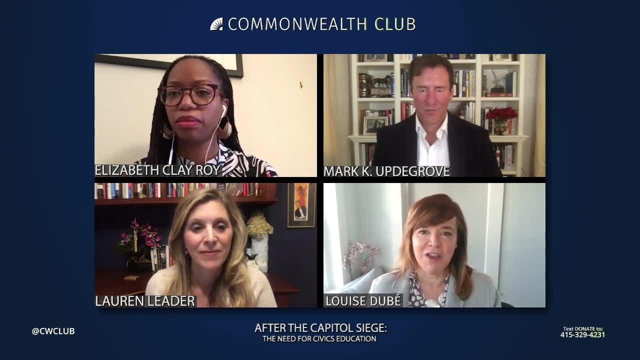 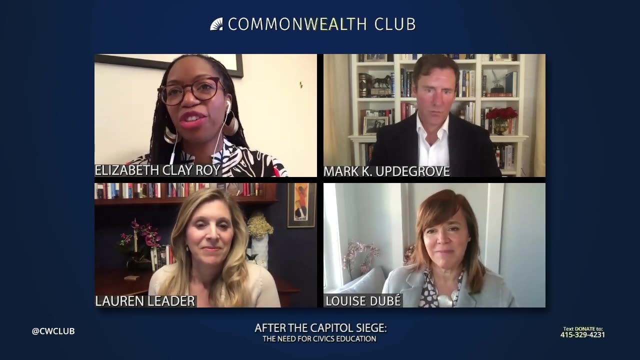 young people are really paying attention now And that attention can be used in so many different ways: Poetry, math, English, everywhere you could infuse civics, Absolutely agree. And you know, I think, the part of this conversation that's really stirring me. 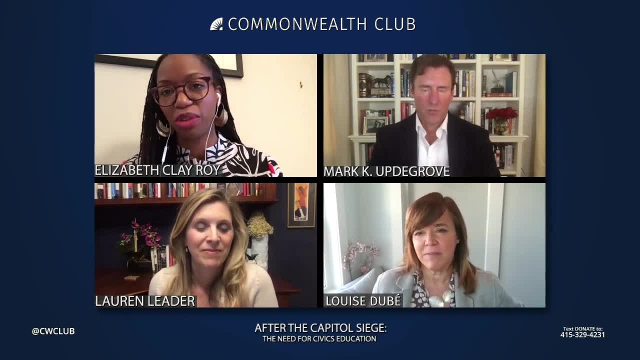 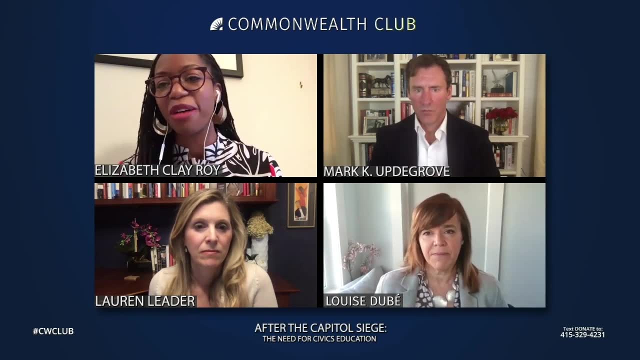 is, you know, our attention to the connection between history and civics, the need to be honest. in the same way that right now it means something to say you're pro-democracy- We can no longer assume that that is true of everyone- It also means something to be pro-truth. 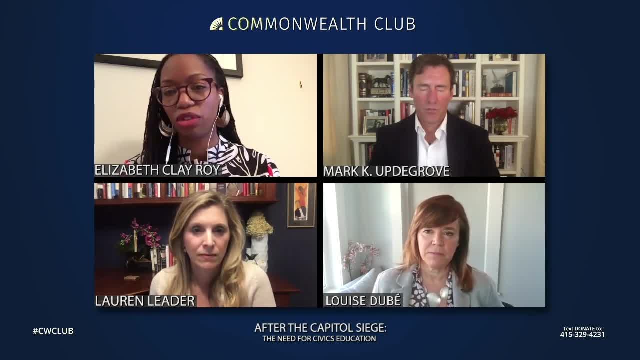 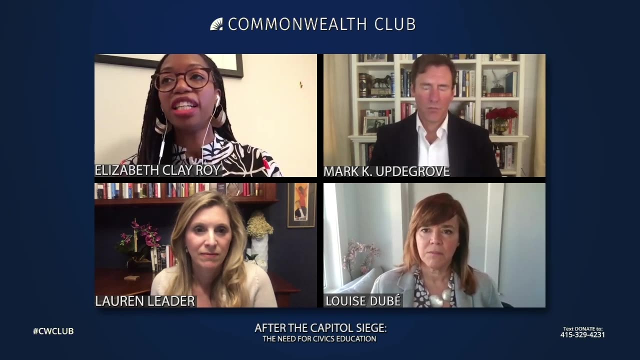 right And to make sure that we are attentive to bringing- not gaslighting students, but bringing them the complexity of the situation, the country that they've been born into, And recognizing and trying to be honest, And I think that's something that we need to be honest about And I think that's. 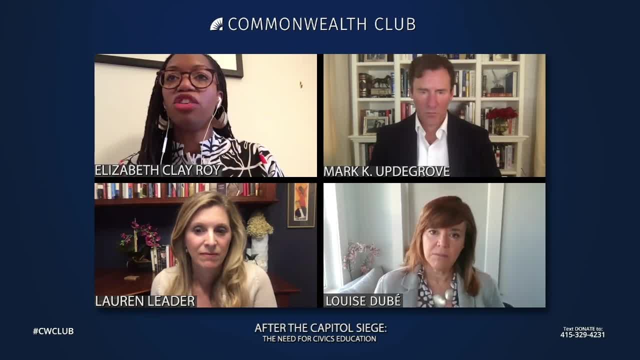 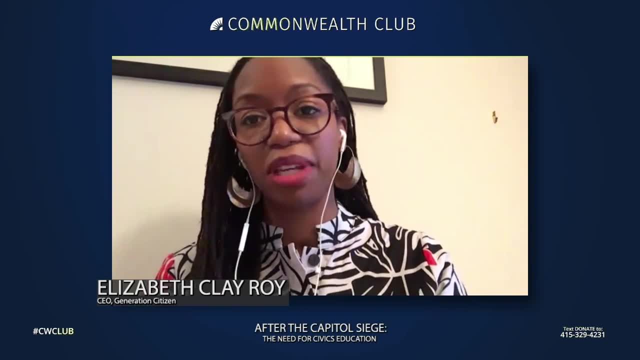 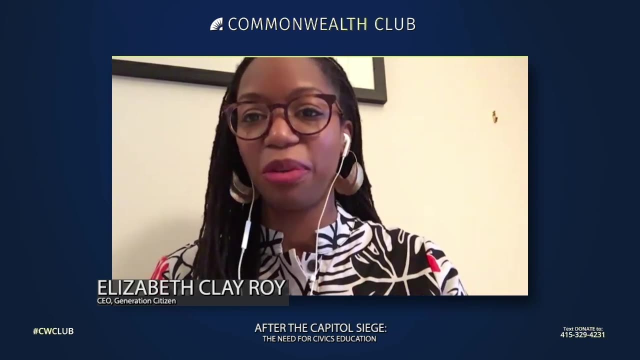 interesting to some degree in the resilience of young people. You know I, on January 6th, was certainly thinking about you know how do we talk about this to young people? What must they be thinking? And I was reminded about, it just came instantly- about how many of our young people 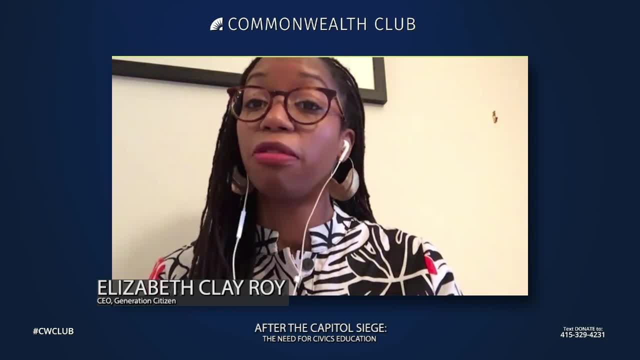 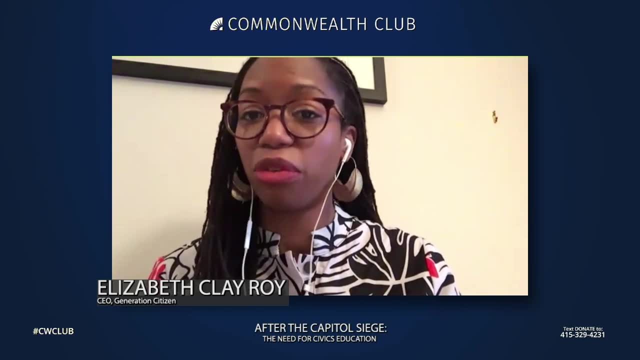 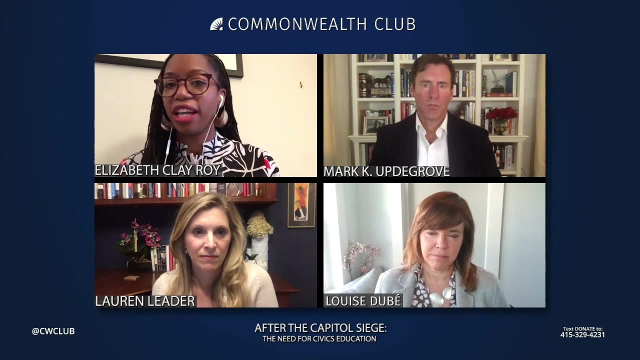 have in fact been dealing with the fear and terror of someone coming into their classroom with a weapon, And that this is a generation that has grown up with that In such a visceral and difficult way, And that we need not shy away from telling young people the 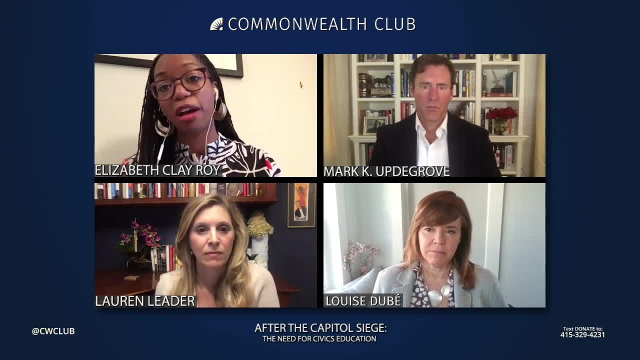 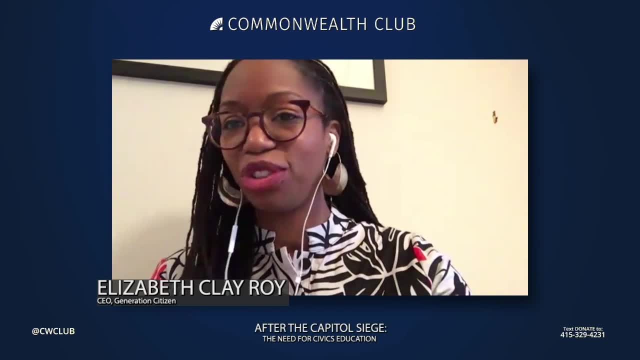 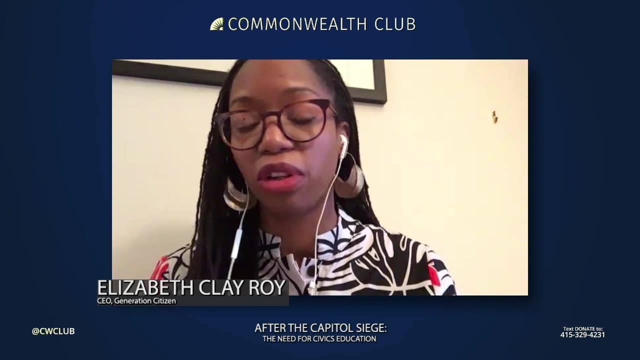 truth in developmentally appropriate ways, from elementary school on up, about this country, Not shying away from the difficult parts, Because that prepares them to help us move to the next place forward. And the civil rights movement is such a, you know, beautiful example of this. 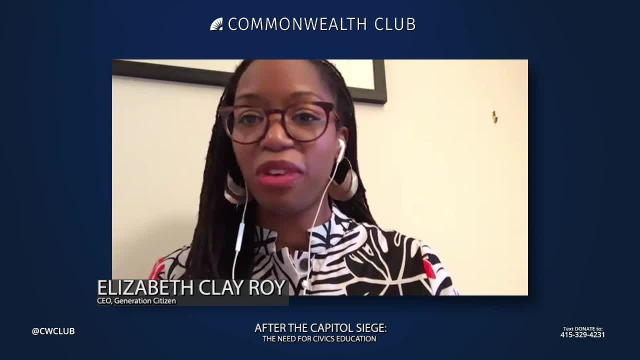 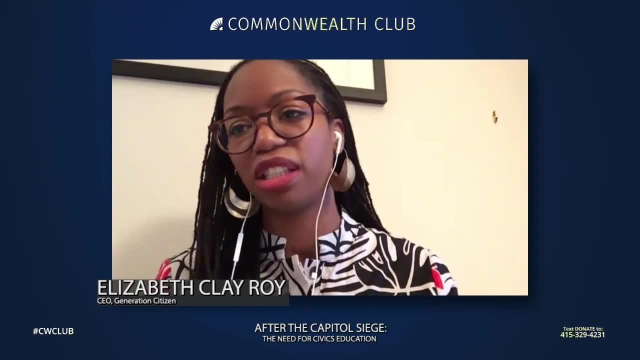 And recognizing that it was the boldness of young people that made it possible for young people to move forward, And the boldness of young people in streets, in boycotts, putting their bodies on the line, that helped us move forward as a country in such a profound and you know, and consequential. 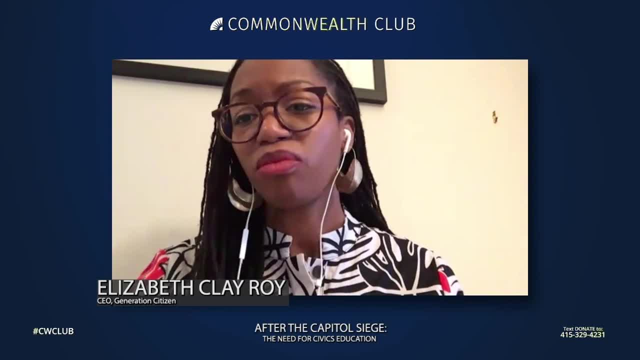 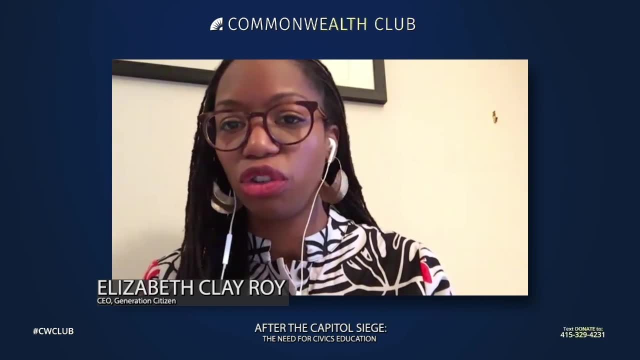 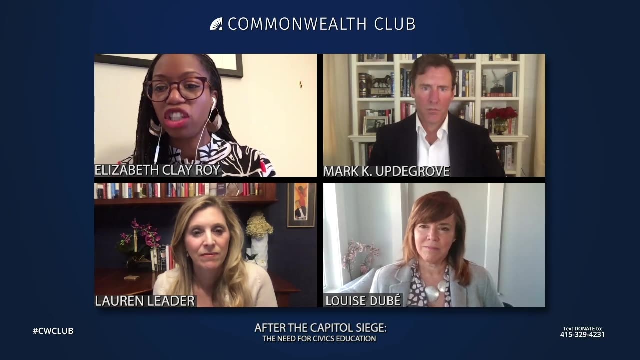 way for the entire country. I want to try to pull in one more question from the conversation on YouTube. It might not get to go to everybody, But I you know there's a question here that I want to hear about Teacher preparation programs that have civic ed, and there's a suggestion even. 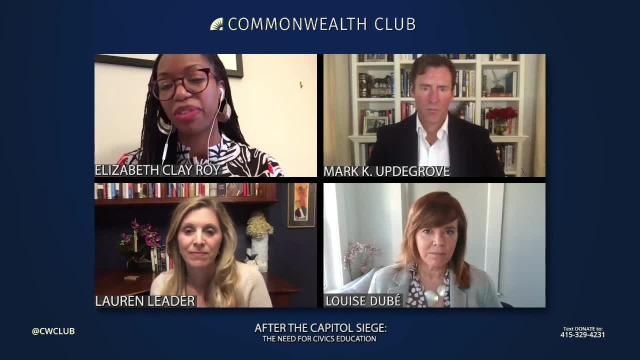 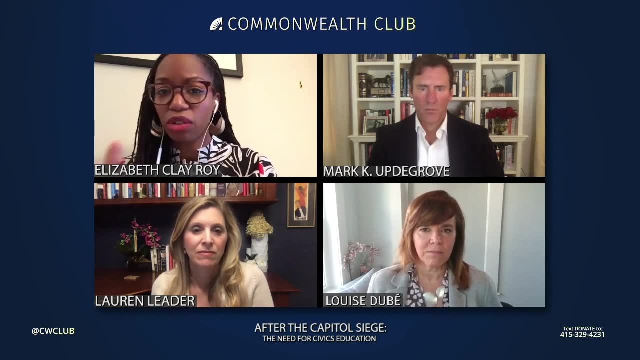 of a civic ed and anti-racist requirement for graduation, Maybe for schools and for teacher preparation. I'll say one thing briefly and then invite Louise or Lauren or Mark to say anything that they want to about the role of teachers. We at Generation Citizen think a lot about that. 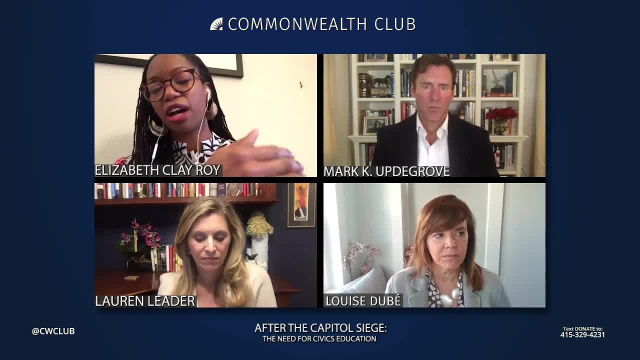 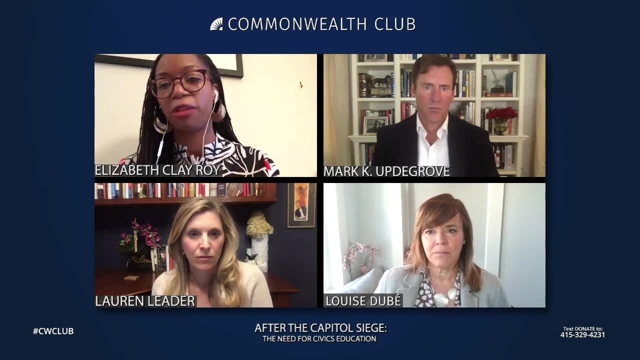 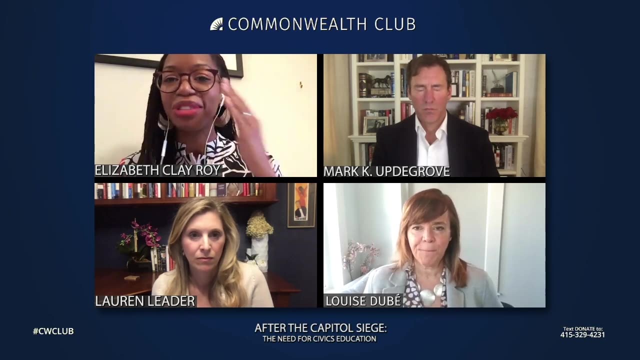 Our model is actually to support teachers and provide them professional development, Coaching and support to do experiential, project based civics in the classroom, And so we think teacher preparation is everything and recognize that teachers are emerging through the same society that we're all in, Which means they might not have had a really robust engaging civics. 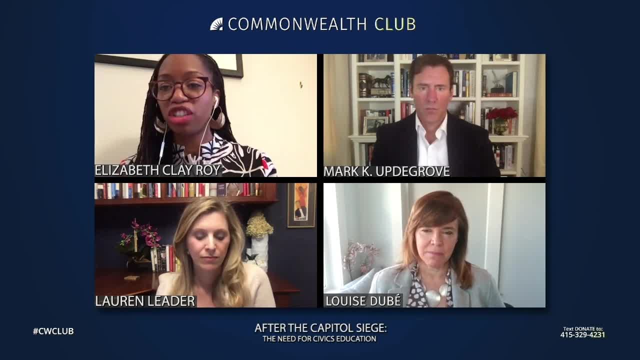 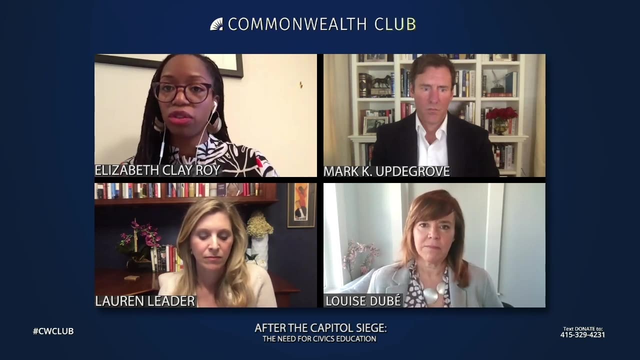 education in their own growing up And that we want to co-create something powerful for their students together. So I think teacher preparation is essential. It's a part of our focus on equity in civics. We bring an equity rooted both curriculum but also values in terms of what we bring to teacher. 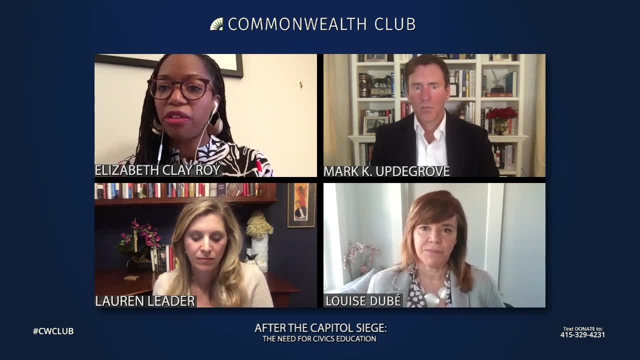 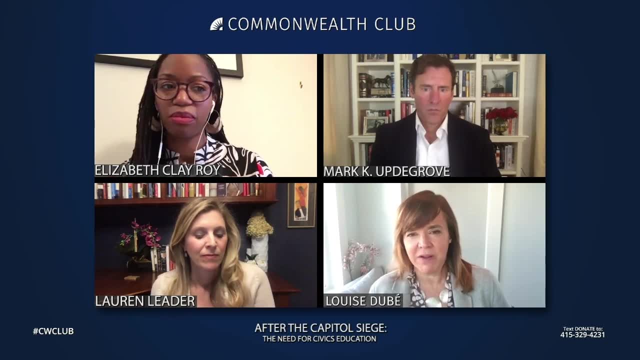 preparation. So that's really important for us. Anyone else want to pick up on teacher preparation before we go to our last question? So I'll just say briefly: 100% agree. As a result of the disinvestment in the field, in history and civics, we haven't had the capacity building, And this is 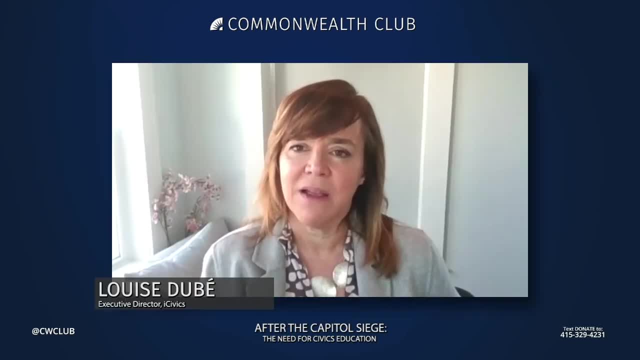 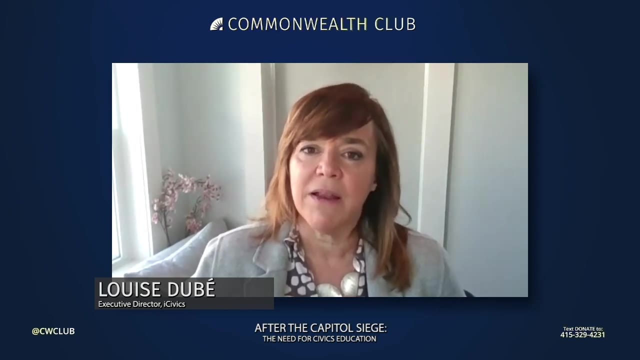 one area that I think is really important for us, And I think it's important for us to have a. we need to invest in our educators to be able to do the deep level work that is needed. As part of the Educating for Democracy Act, there is a provision calling for an investment in 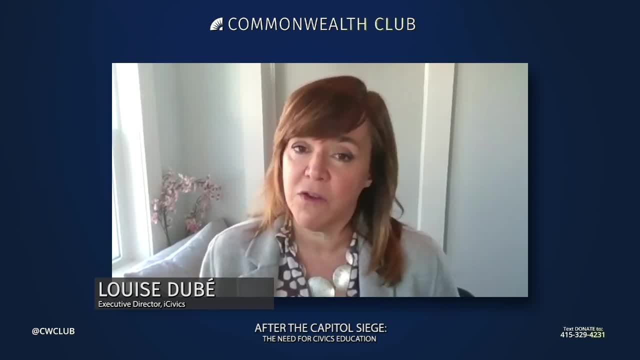 graduates from the humanities, particularly graduates of color, to diversify the pipeline, And that is very important. And having a background in the humanities, in history, civics, political science, is important because you need that depth of knowledge, And so, the idea being that we should incentivize. 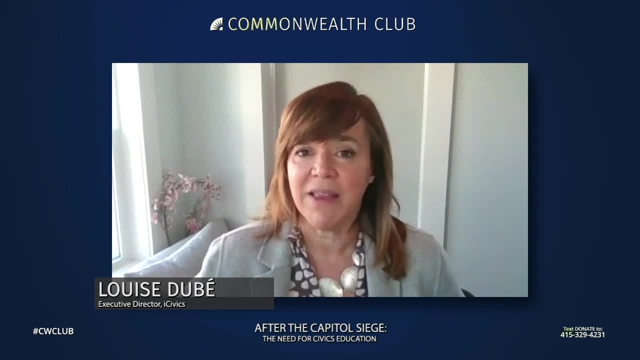 that kind of participation and that pipeline, And obviously teacher preparation programs have a role to play. There's also alternative certifications that could be applied. So there's a range of ways to get that. But I think everybody agrees that this is an area that's been 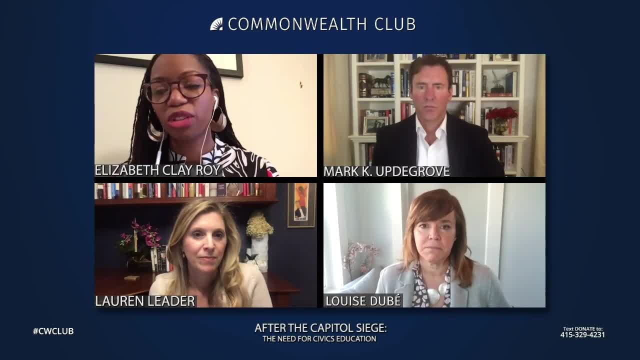 vastly underfunded ELIZABETH LITTLEFIELD FD. Absolutely, Absolutely. So we're going to go to just our last question And I'll invite you to go in reverse order of how we started, So starting with Mark, then Lauren, then Louise. 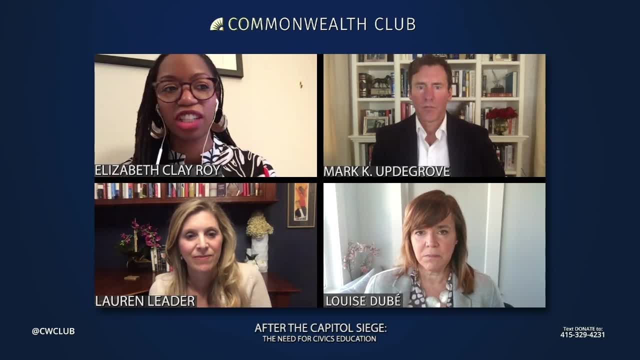 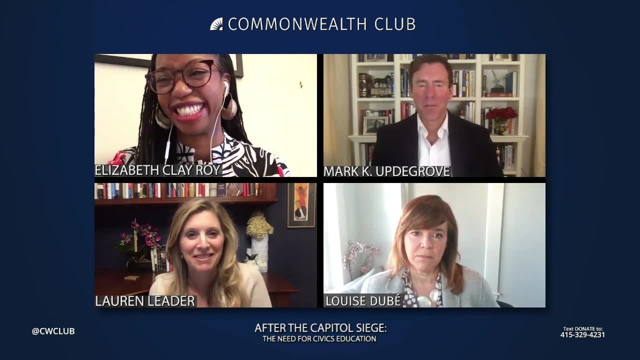 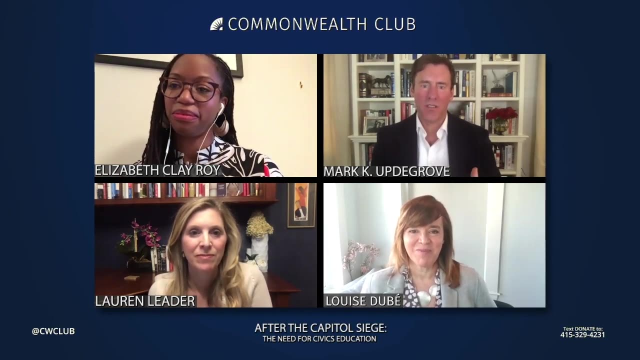 What's one thing that people can do in their communities to make civics education a priority for everyone? In 30 seconds, if you can. MARCIA KERNAN- I'm glad Marc's first. LAWRENCE BAKER- I think Louise said it- You've got to go to your school boards and talk to them about the importance of teaching civics. 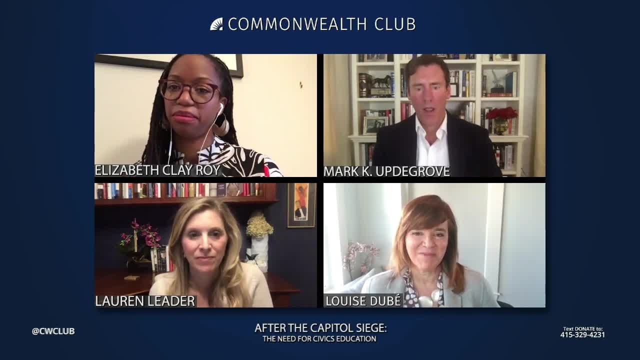 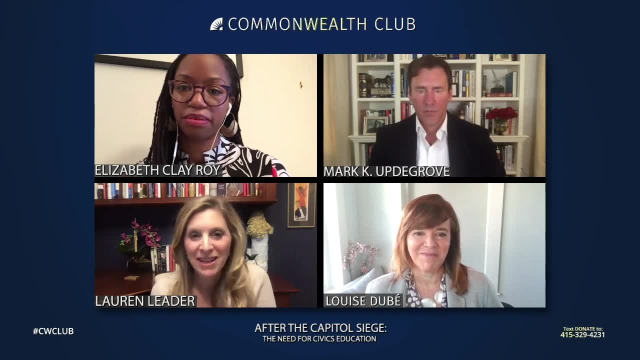 We can all get involved in this, But we can all improve our between school districts, And so our mission is to make that a priority, implore our schools to take this seriously, and now is the moment, I would add, lead by example. Our children are watching, and the more we participate and bring. 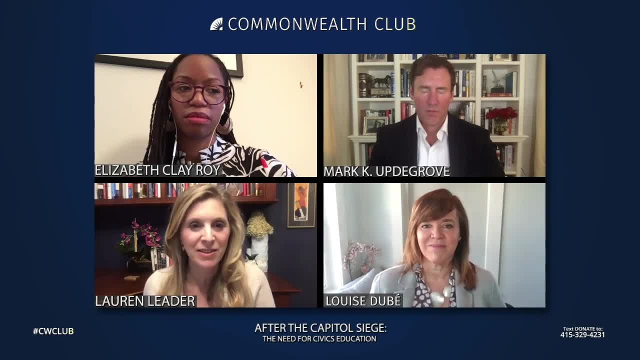 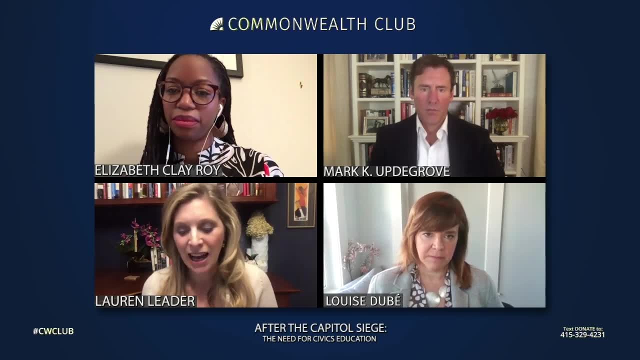 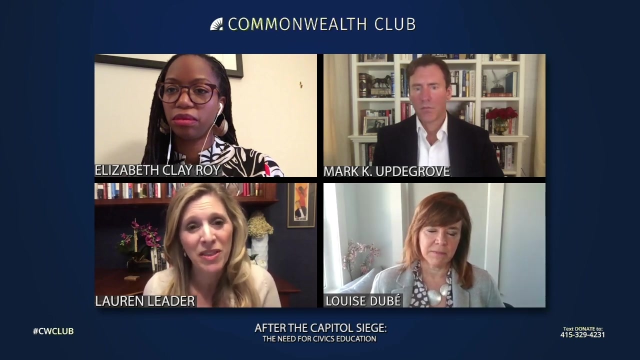 our children along to see what that participation is and means. the way, showing up at our town board meetings and our local elected gatherings and writing to our elected officials and showing our children the model of civic participation that's peaceful and constructive and positive is absolutely transformational. taking our kids to vote with us, introducing them to our local 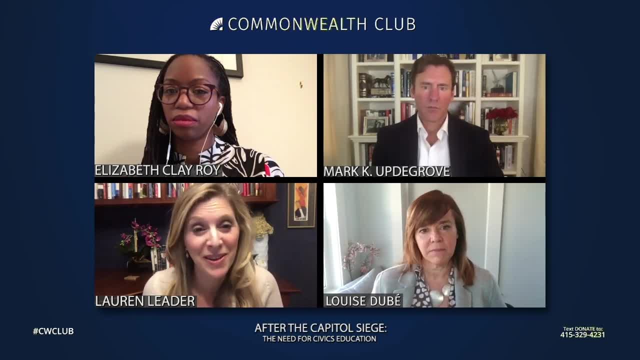 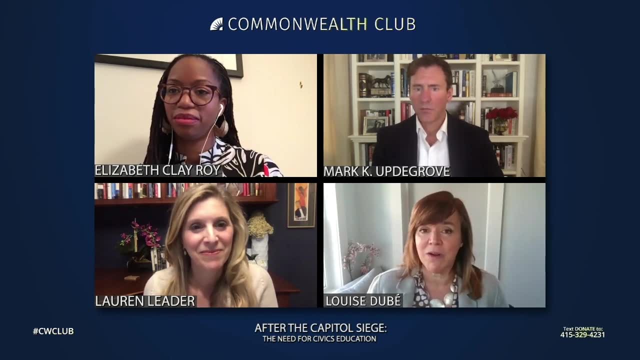 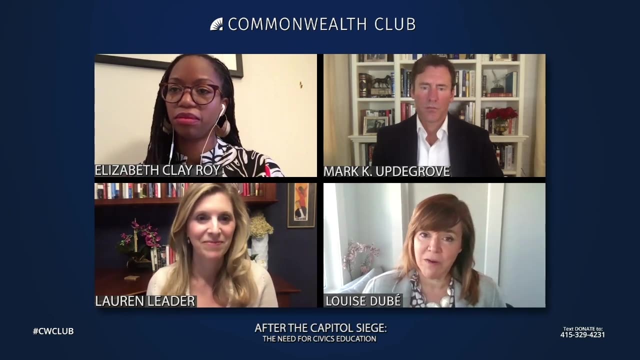 elected officials. They watch and they learn and they replicate. Write to your Congress member and ask them to urge the passage of the Educating for Democracy Act, and write to your school board, as Mark suggested, and ask them to draw up a civic learning plan that will guarantee how each and every student 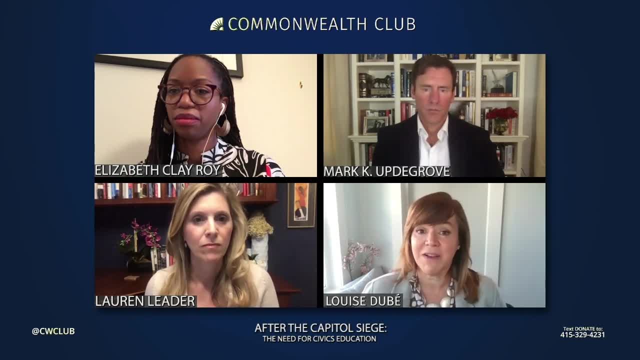 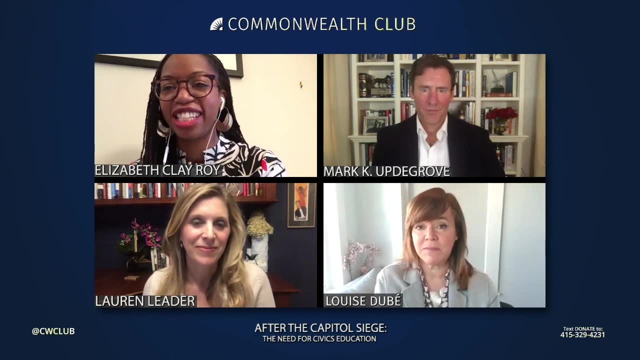 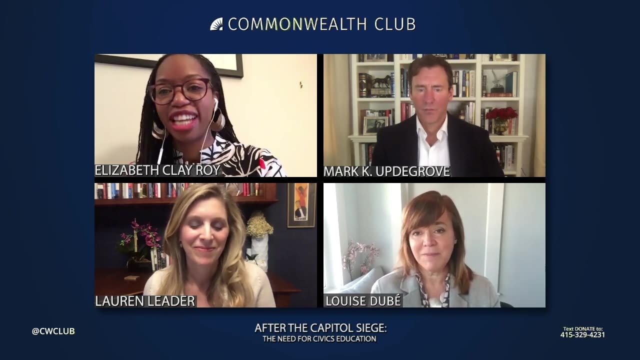 in that district will graduate prepared and engaged for civic life. Fantastic, What tremendous suggestions and things that everyone who is listening can do as we move forward. Unfortunately, this is all the time we have for today's program, and I want to thank each of our speakers today for what they've shared. 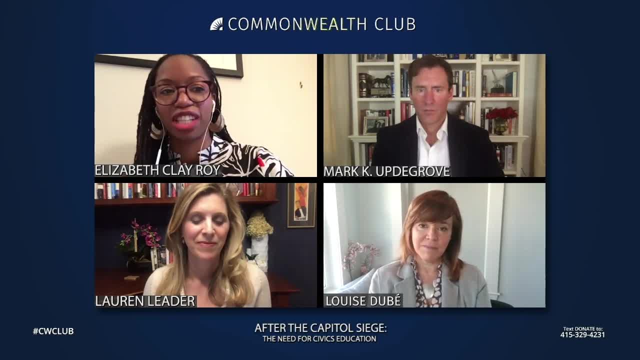 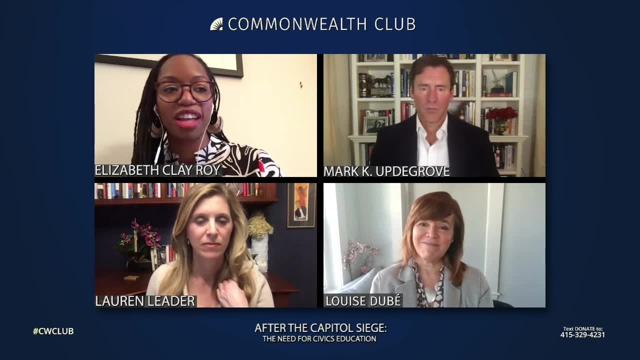 and I hope that you have a great day And, of course, thank the Commonwealth Club, our host, for today's conversation. I hope it's not the last one on this important topic. The club's going to be posting this video along with other. 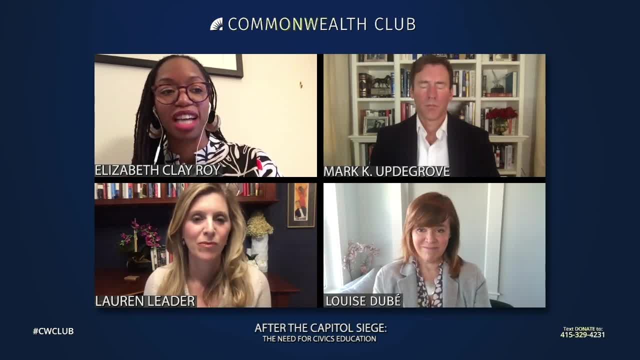 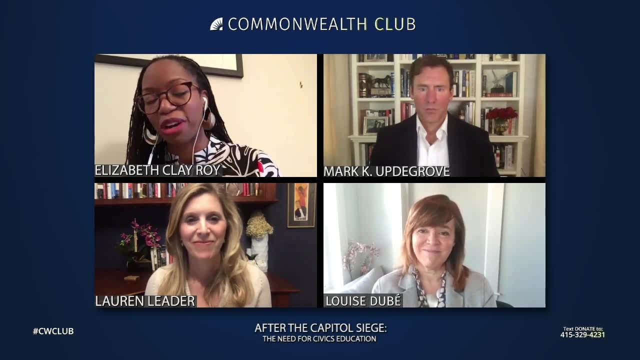 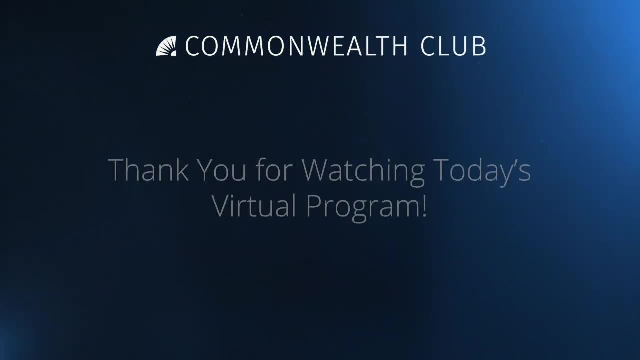 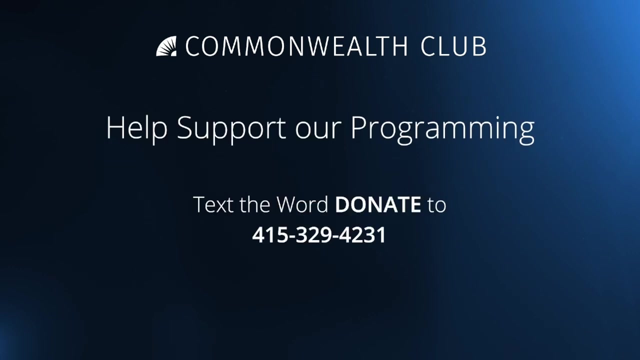 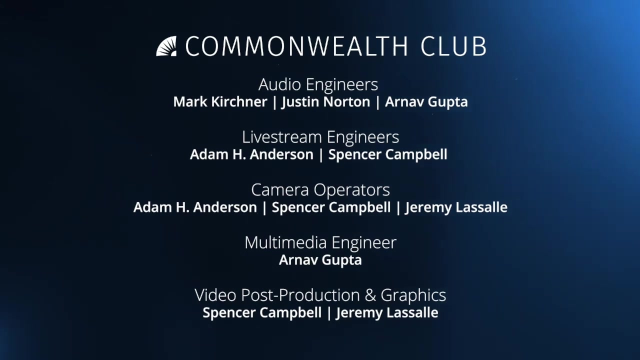 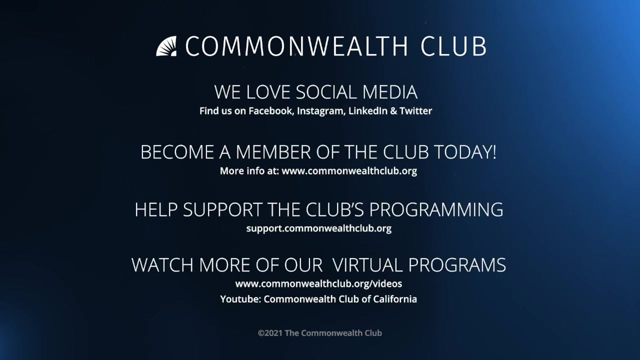 civic education resources at their website, wwwcommonwealthcluborg. I'm Elizabeth Clay Roy, of Generation Citizen, and this special virtual program of the Commonwealth Club has now concluded. Thank you, Thank you.